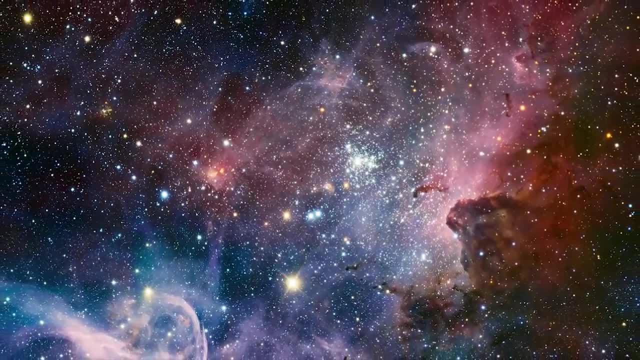 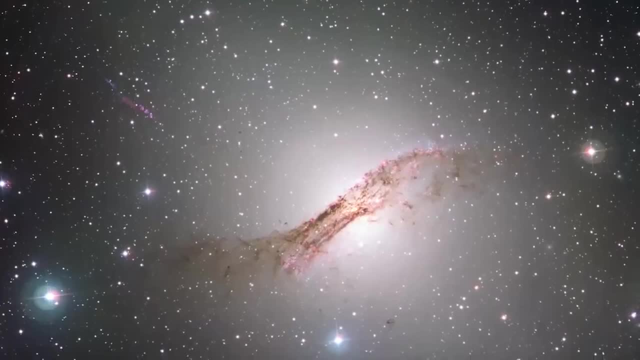 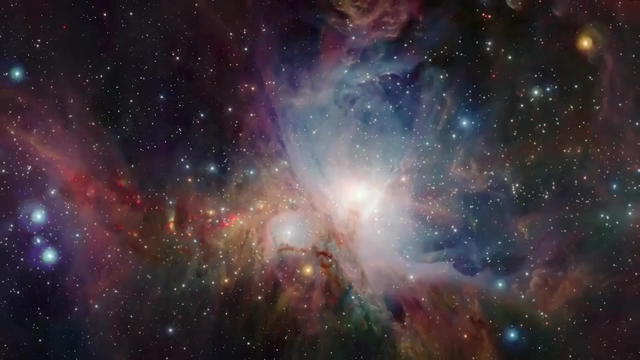 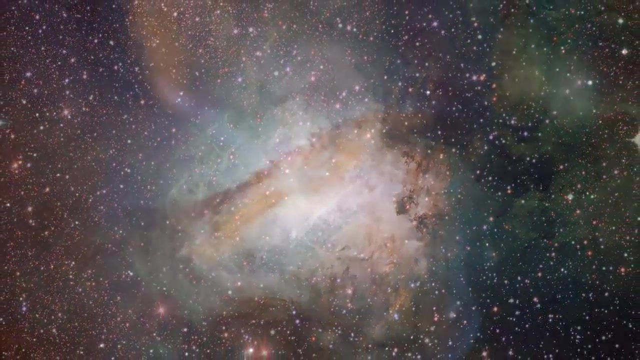 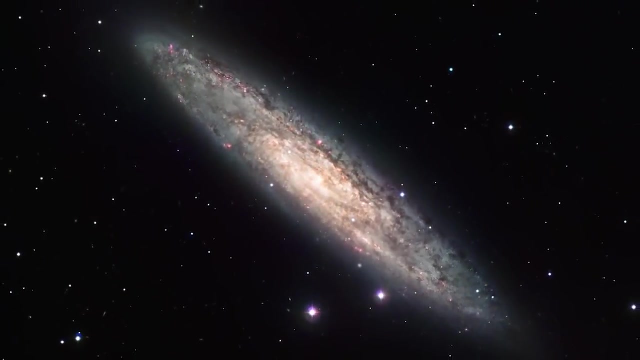 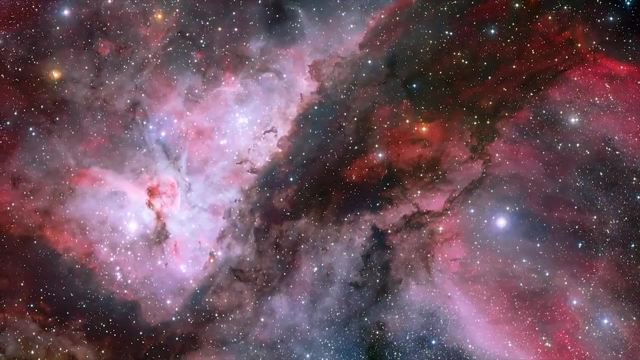 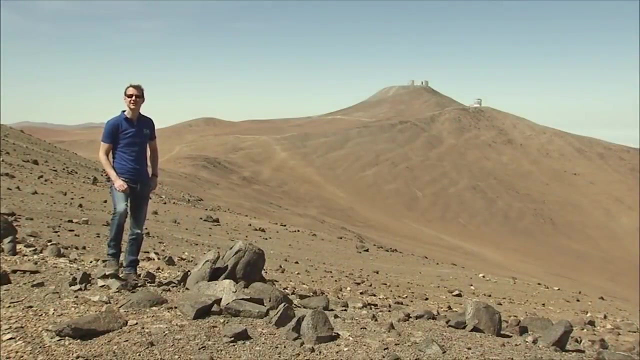 giving us fresh insights and an unprecedented view of the Universe. ESO's Hubble Space Telescope is a world of deep mysteries and hidden secrets… and staggering beauty. A universe of deep mysteries and hidden secrets… and staggering beauty. From remote mountain tops in Chile, European astronomers are reaching for the stars. 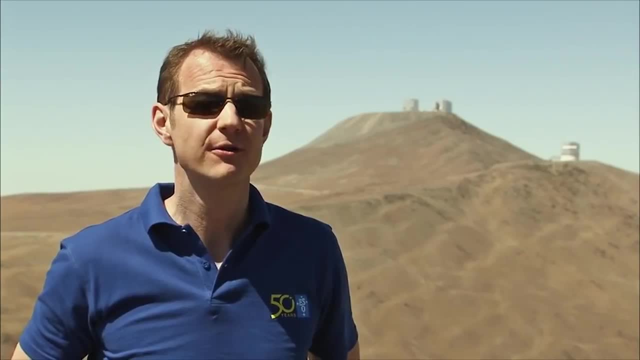 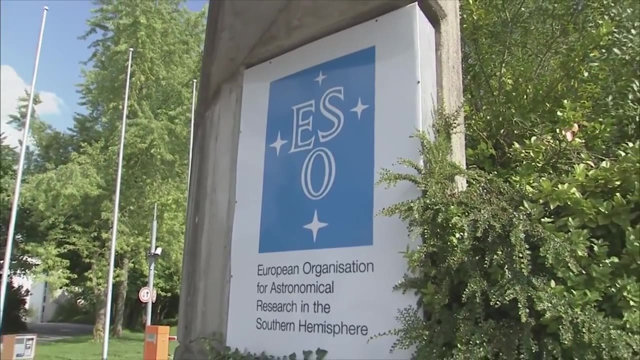 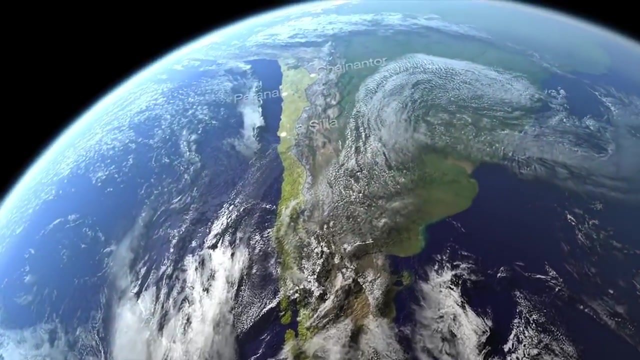 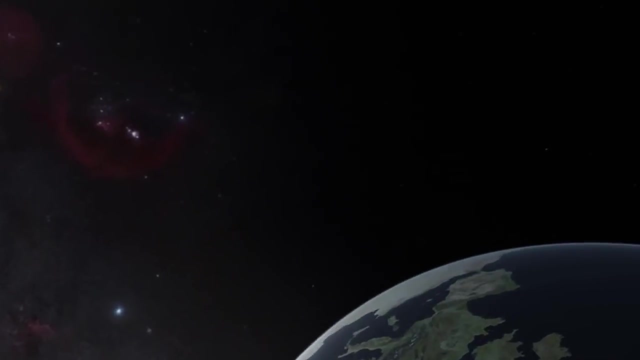 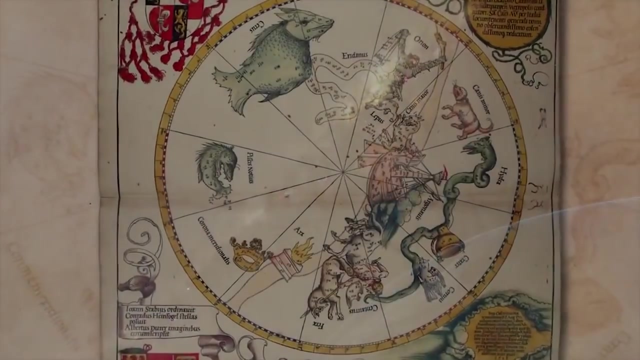 But why Chile? What made the astronomers go south? The European Southern Observatory has its headquarters in Darsingh, Germany, But from Europe only part of the sky can be seen. To fill in the gaps, you have to travel south For many centuries. 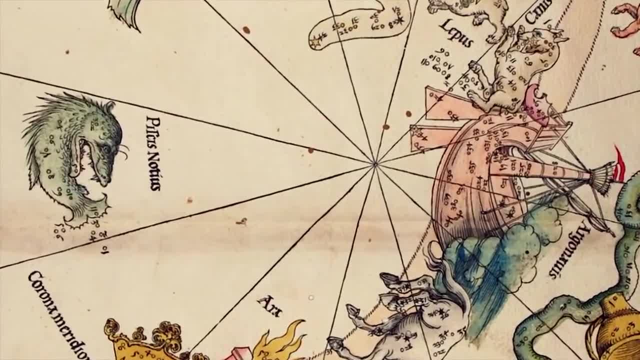 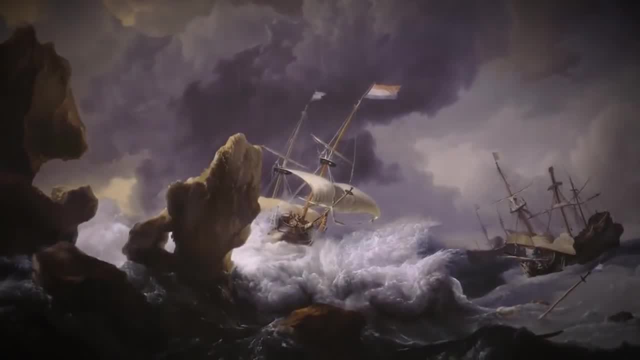 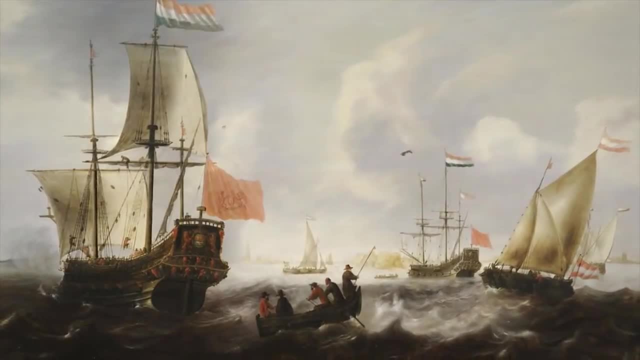 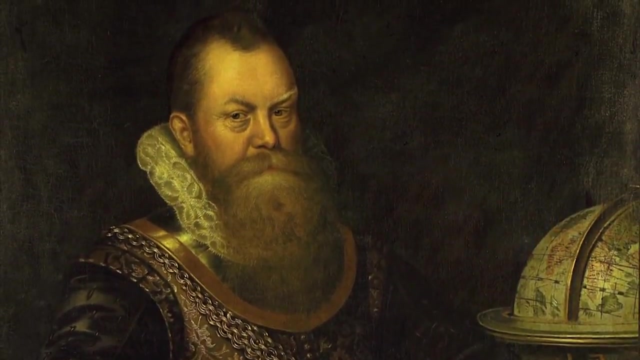 maps of the southern sky showed extensive blank areas, the terra incognita of the heavens, 1595.. For the first time, Dutch traders set sail to the East Indies At night. navigators Peter Keizer and Friedrich de Houtman measured the positions of more than 130 stars in the southern sky. 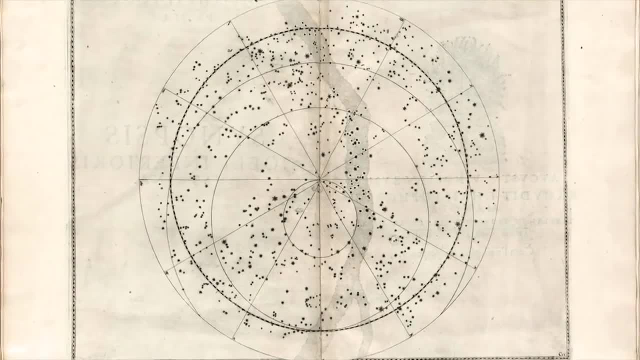 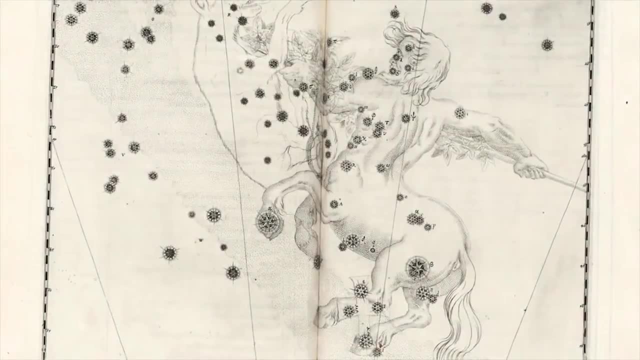 In the early 18th century, the sun was shining in the sky and the stars were shining in the sky. Soon celestial globes and maps showed 12 new constellations, none of which had ever been seen before by any European. 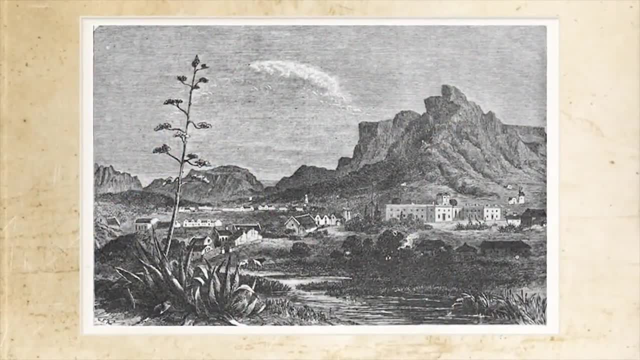 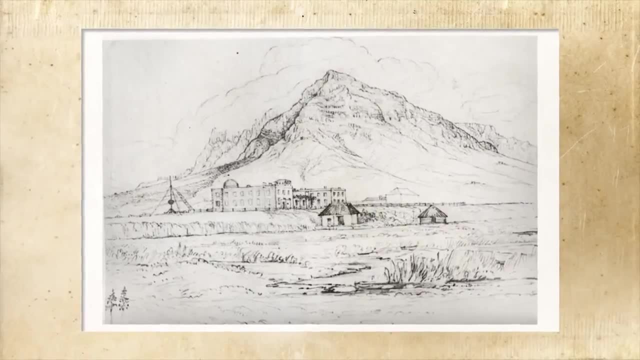 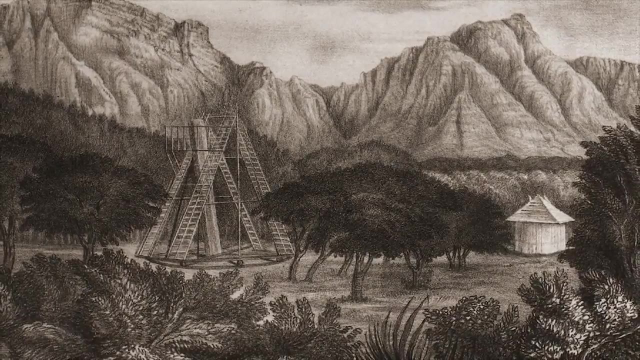 The British were the first to construct a permanent astronomical outpost in the southern hemisphere. The Royal Observatory at the Cape of Good Hope was founded in 1820.. Not much later, John Herschel built his own private observatory close to South Africa's famous Table Mountain. 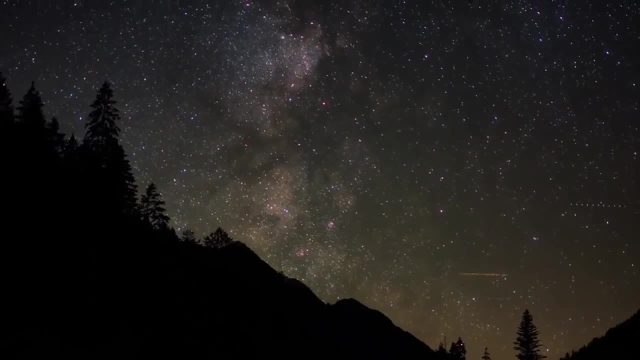 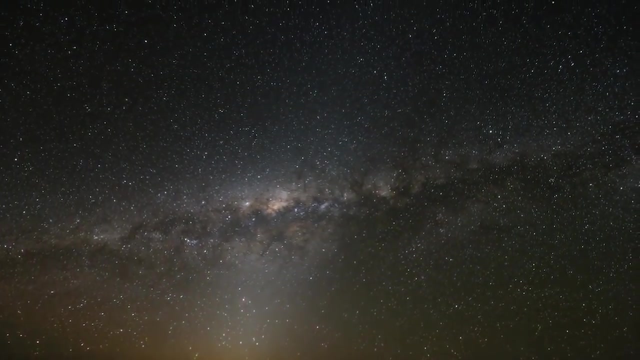 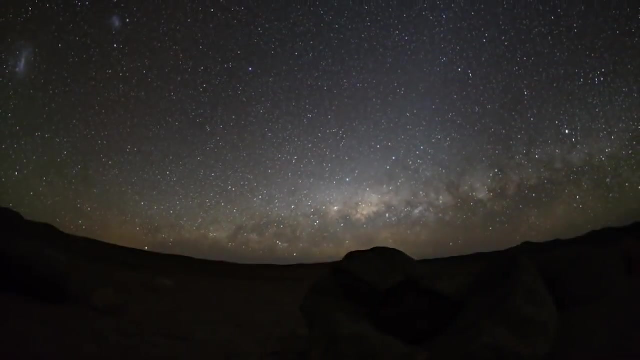 What a view: Dark skies, bright clusters and star clouds high overhead. Little wonder that Harvard, Yale and Leiden observatories followed suit with their own southern stations. But the exploration of the southern sky still took lots of courage, passion and perseverance. 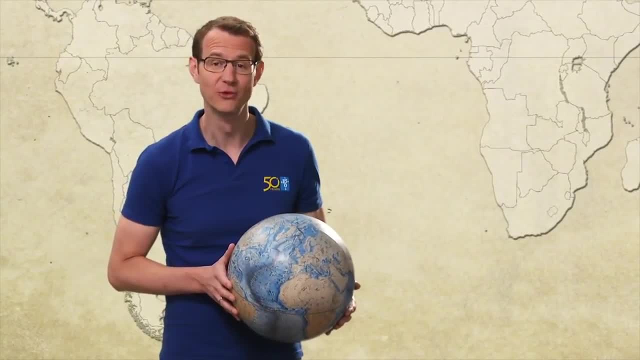 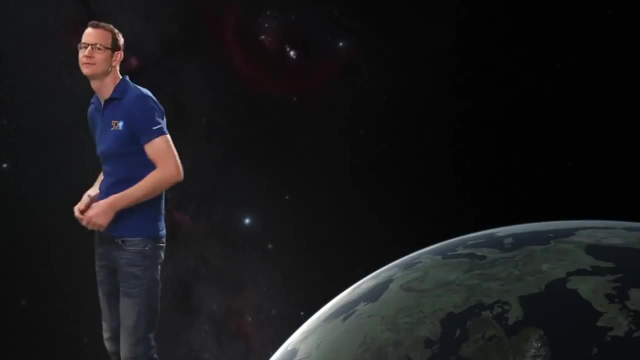 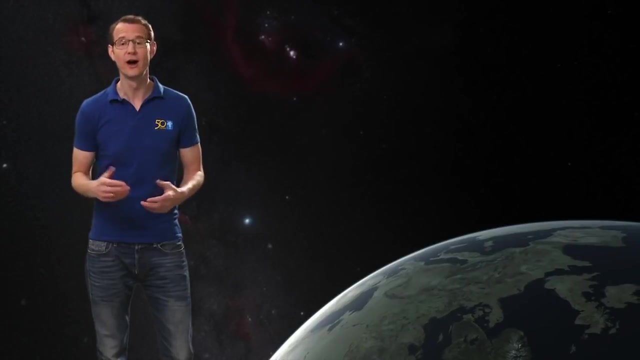 Until 50 years ago, almost all major telescopes were located north of the equator. So why is the southern sky so important? Well, first of all, because it was largely uncharted territory. You just can't see the whole sky from Europe. 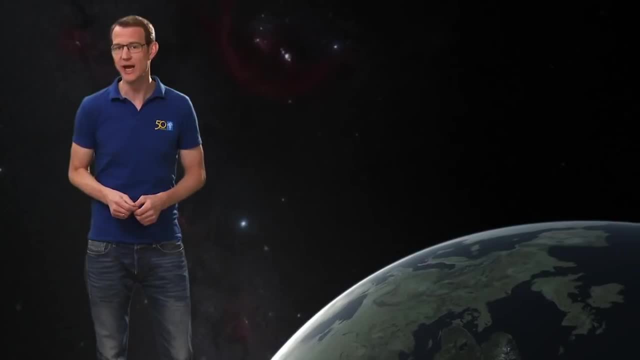 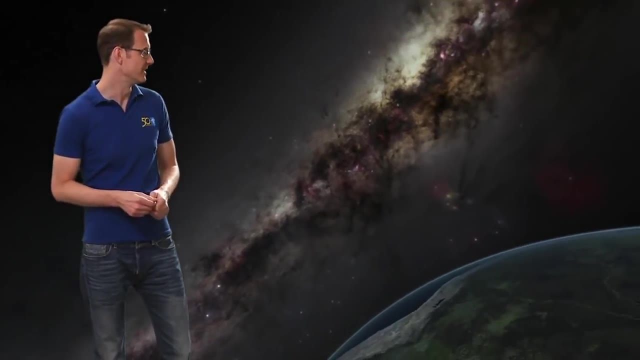 A prominent example is the centre of the Milky Way, our home galaxy. It can hardly be seen from the northern hemisphere, but from the south it passes high overhead. And then there are the Magellanic Clouds, two small companion galaxies to the Milky Way. 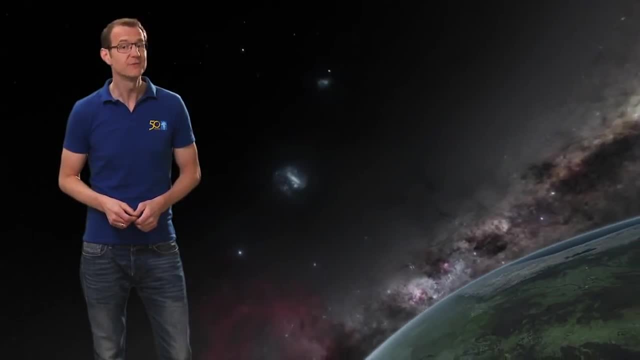 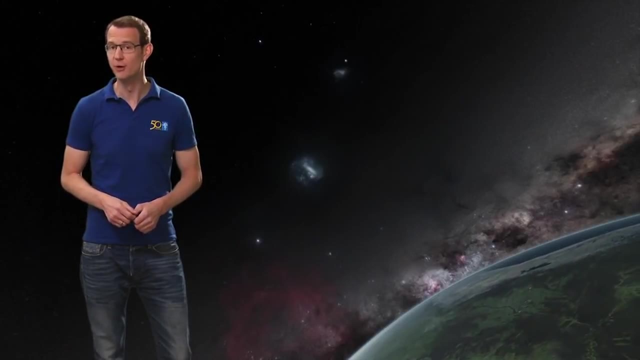 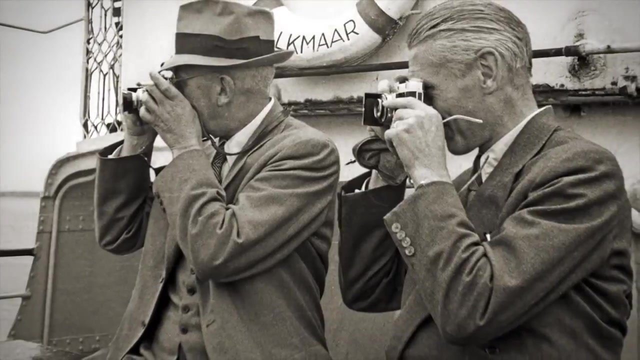 Invisible from the north, but very conspicuous if you're south of the equator. And then, finally, European astronomers were hindered by light pollution and poor weather. Going south would solve most of their problems. A scenic boat trip in the Netherlands, June 1953.. 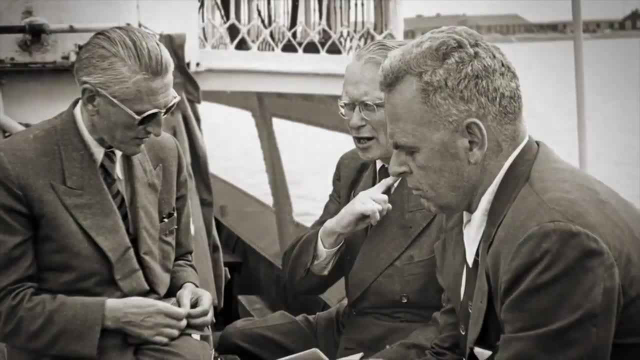 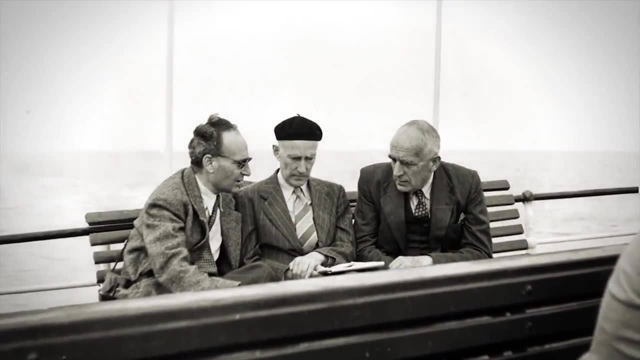 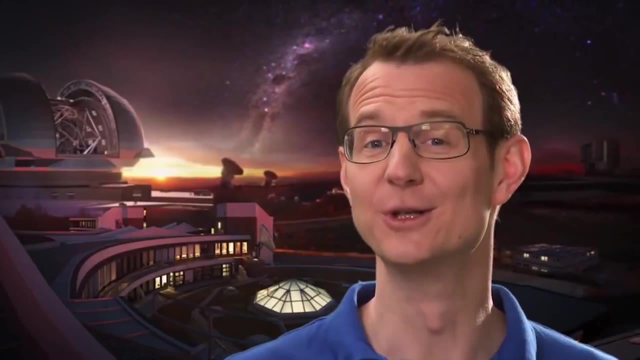 It was here on the IJsselmeer that the German-American astronomer Walter Bardet and the Dutch astronomer Jan Oert told colleagues about their plan for a European observatory in the southern hemisphere: The European Observatory. Individually, no one European country could compete with the United States. 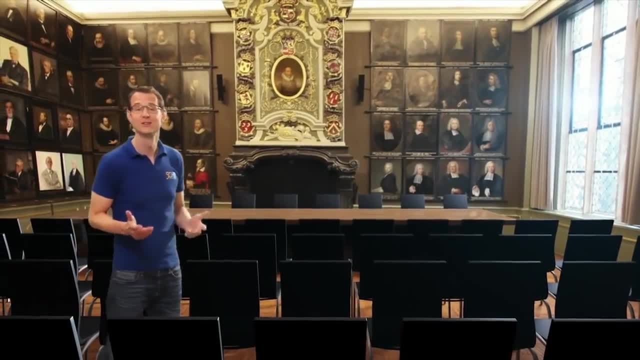 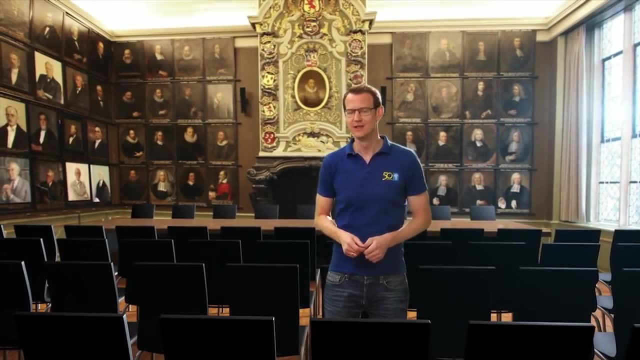 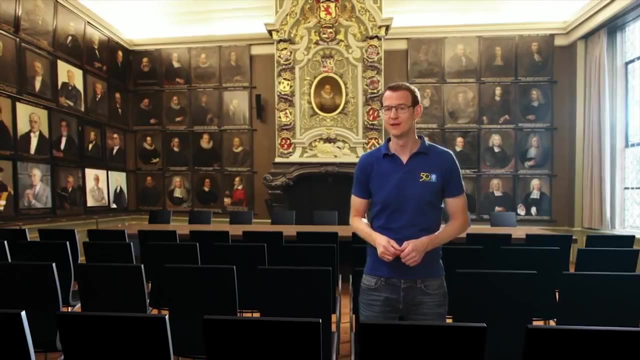 But together they might. Seven months later, twelve astronomers from six countries gathered here in the stately senate room of Leiden University. They signed a statement expressing the desire to establish a European observatory in South Africa. This paved the way for the birth of ESO. 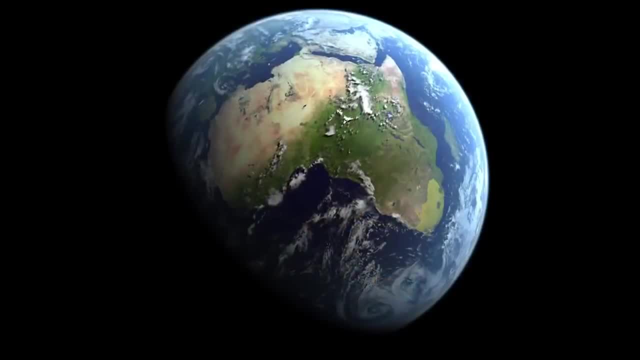 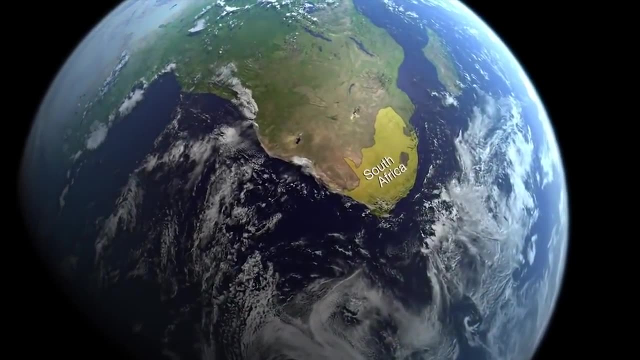 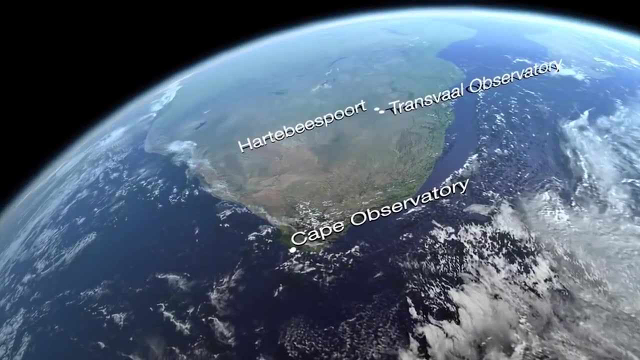 But hang on, South Africa. Well, it made sense, of course. South Africa already had the Cape Observatory and after 1909, the Transvaal Observatory in Johannesburg. Leiden Observatory had its own southern station in Hartebeespurth. 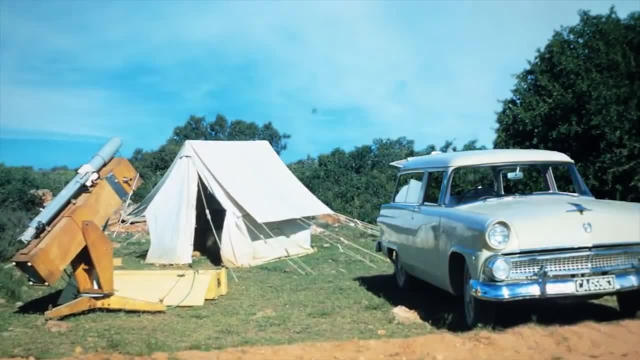 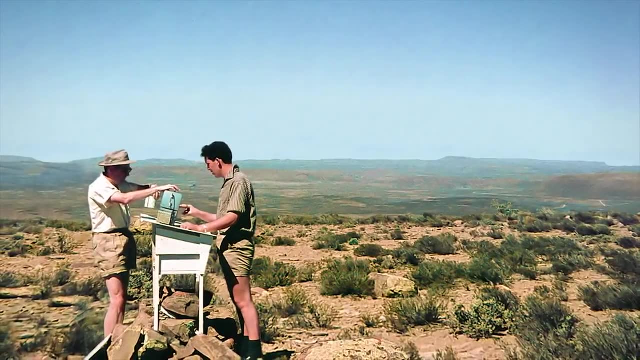 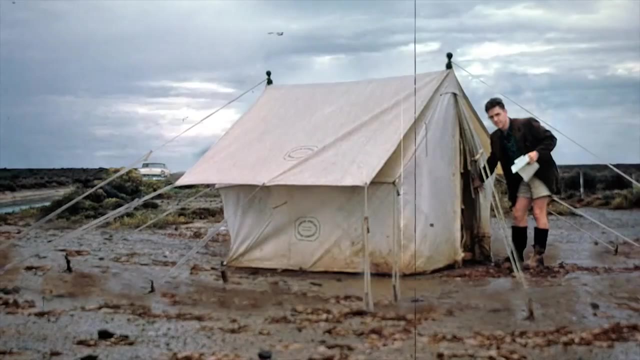 In 1955, astronomers set up test equipment to find the best possible spot for a big telescope. They could have it in the Great Karoo or Tafelkopje near Bloemfontein, But the weather was not all that favourable. 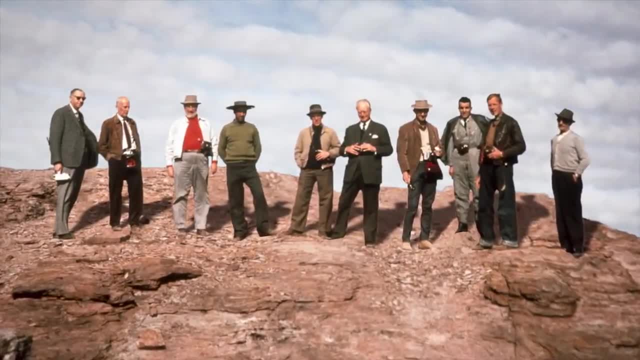 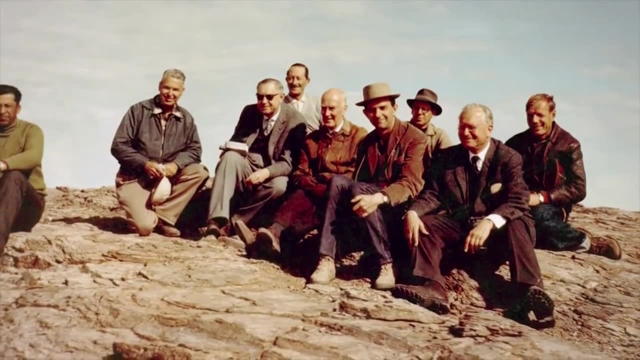 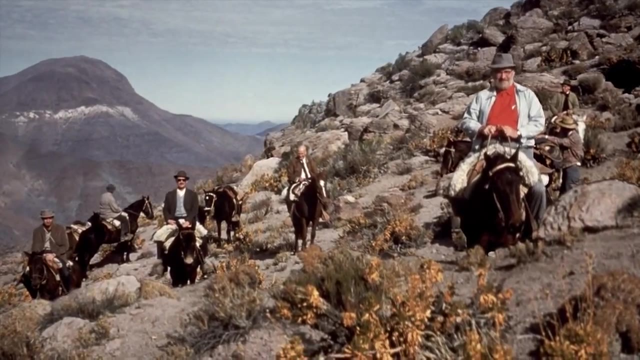 Around 1960,, the focus shifted to the rugged landscape of northern Chile. American astronomers were also planning their own southern hemisphere observatory. here, Harsh horseback expeditions revealed much better conditions than in South Africa. In 1963, the die was cast. 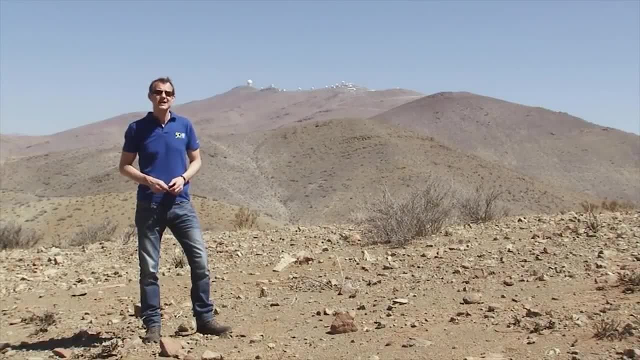 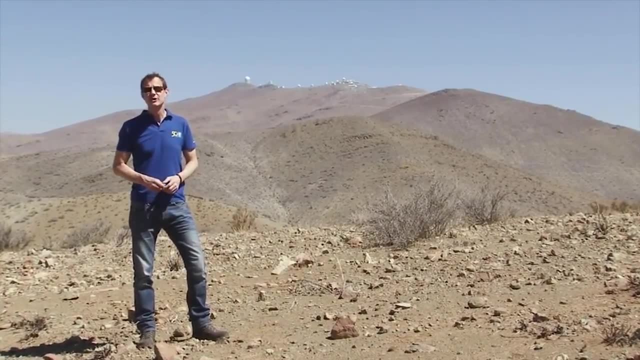 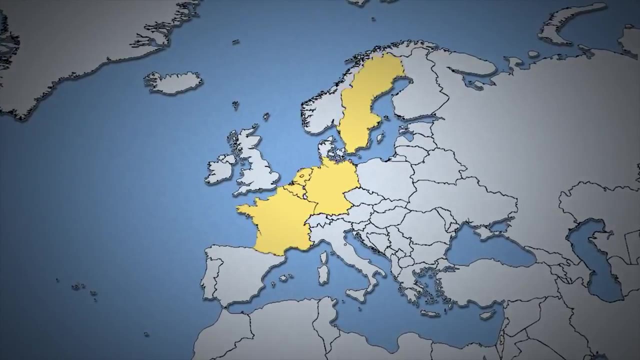 Chile. it would be Six months later. Cerro La Silla was picked as the future site of the European Southern Observatory. ESO was no longer a distant dream. In the end, five European countries signed the ESO Convention on 5 October 1962.. 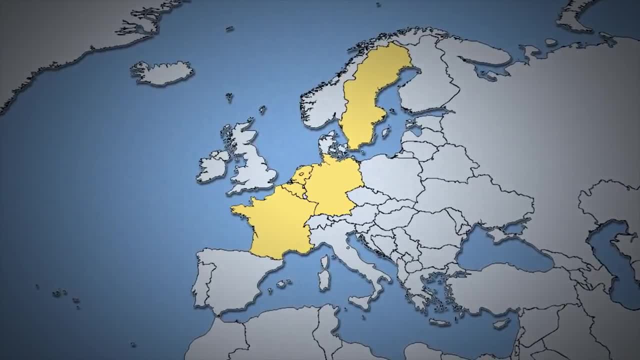 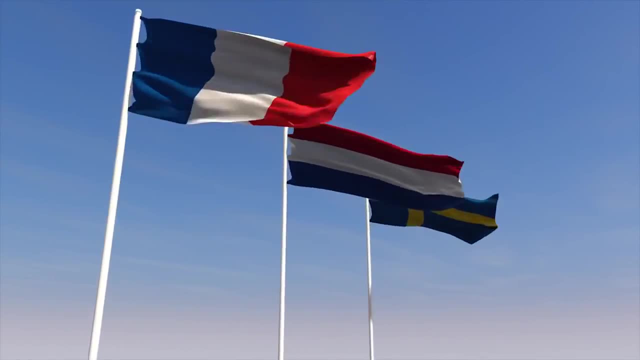 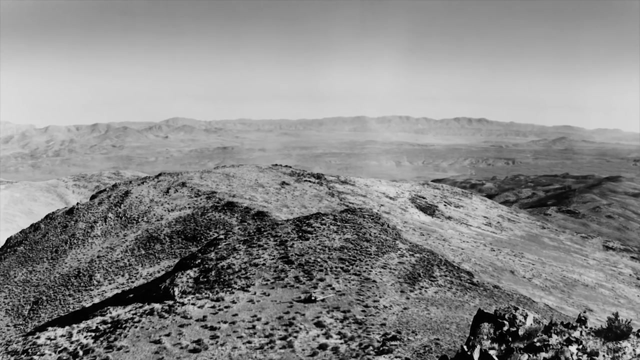 The official birthday of the European Southern Observatory. Belgium, Germany, France, the Netherlands and Sweden were firmly committed to jointly reach for the southern stars. La Silla and its surroundings were bought from the Chilean government. A road was built in the middle of nowhere. 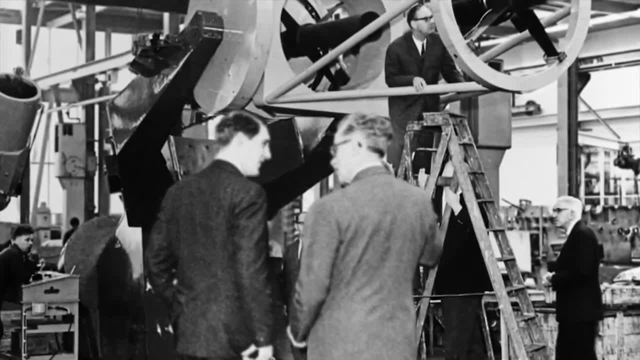 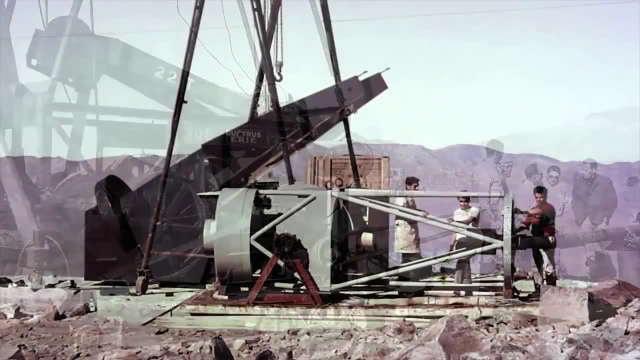 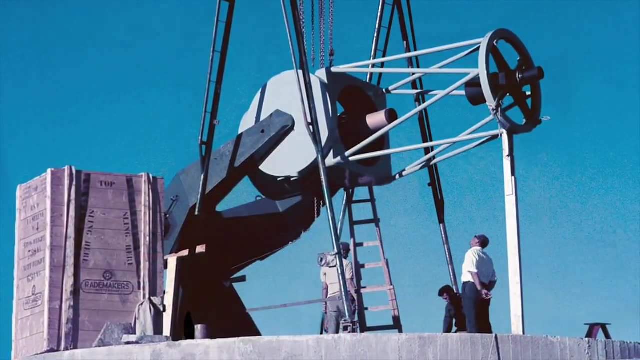 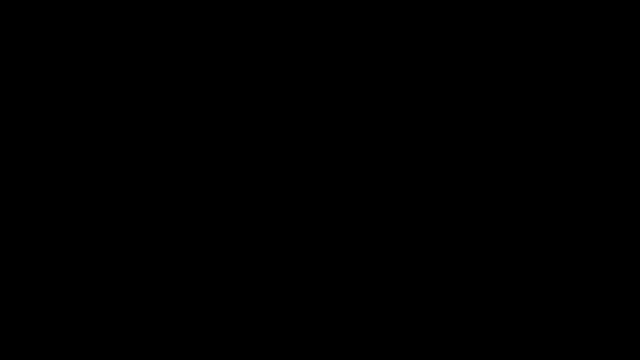 ESO's first telescope took shape at a steel company in Rotterdam, And in December 1966, the European Southern Observatory opened its first eye on the sky. Europe had embarked on a grand voyage of cosmic discovery. It was the first time in the history of the world that a star exploded in a small galaxy orbiting the Milky Way. 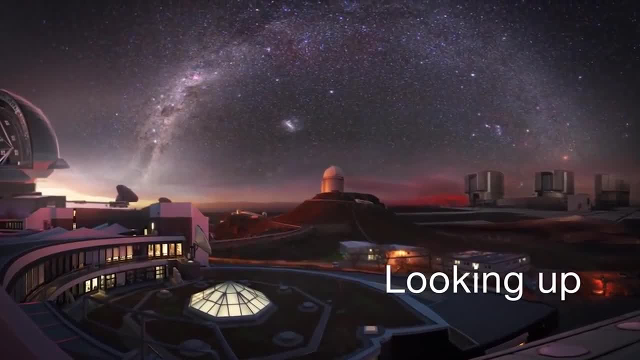 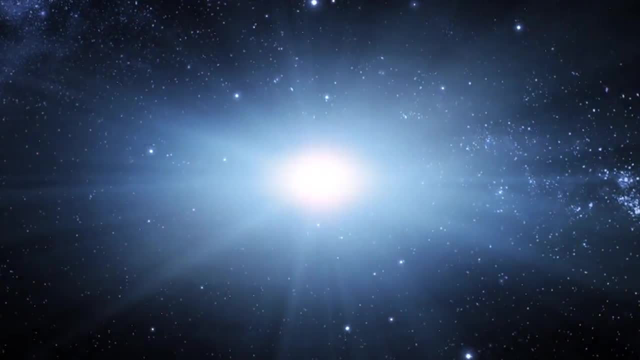 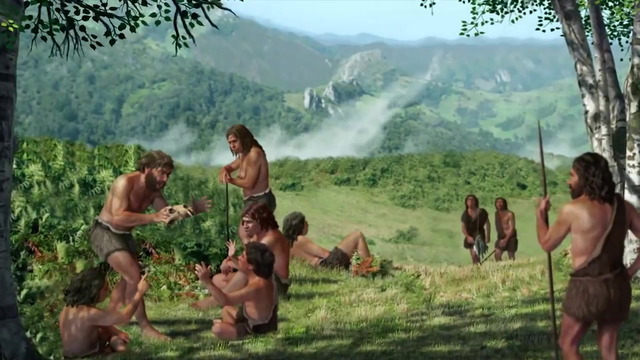 The Milky Way is a small galaxy orbiting the Milky Way. 167,000 years ago, a star exploded in a small galaxy orbiting the Milky Way. At the time of the distant explosion, Homo sapiens just started to roam the African savannah. 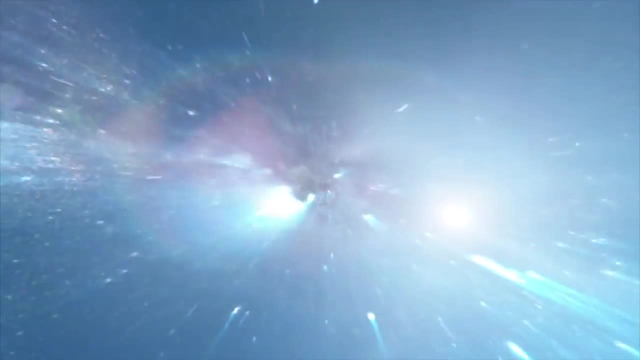 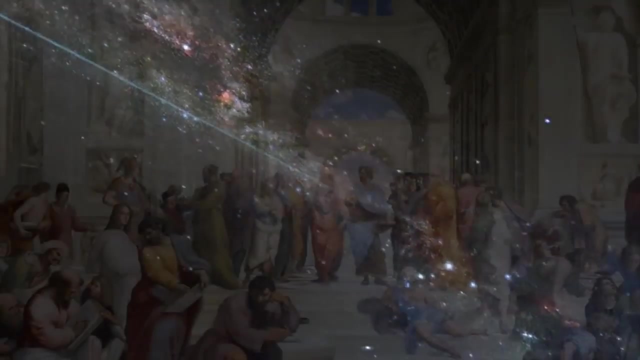 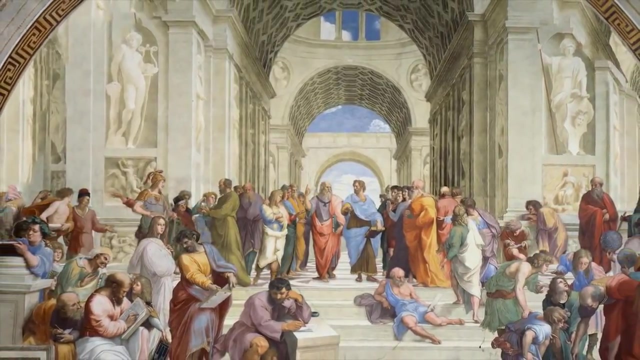 But no one could have noticed the cosmic fireworks, as the blast of light had only just embarked on its long journey towards Earth. By the time, light from the supernova had completed 98% of its journey. Greek philosophers had just started to think about the nature of the cosmos. 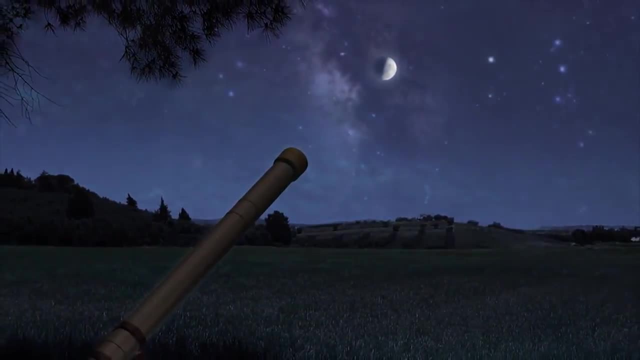 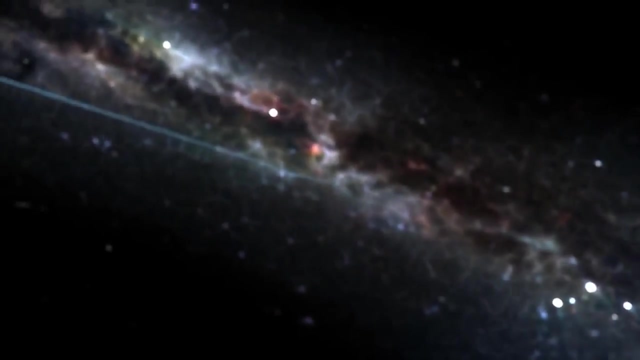 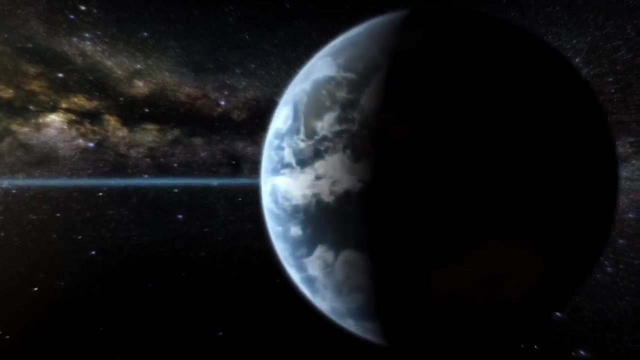 Just before the light reached Earth, Galileo Galilei trained his first primitive telescope on the heavens, And on 24 February 1987, when photons from the explosion finally rained down on our planet, astronomers were ready to observe the supernova in great detail. 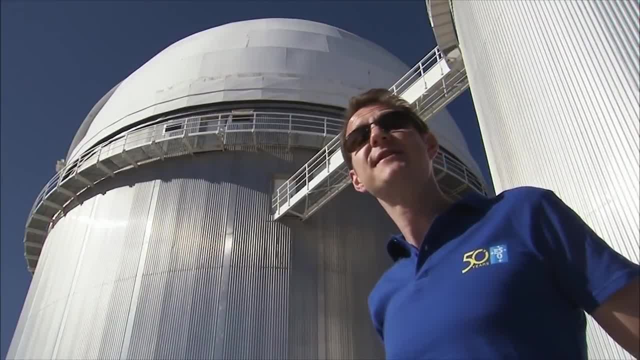 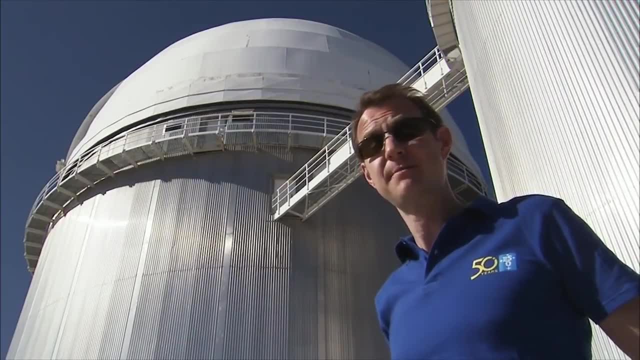 Supernova 1987A flared up in the southern sky, unobservable from Europe or the United States. But by this time ESA had built its first big telescopes in Chile, providing astronomers with a front-row seat to this cosmic spectacle. 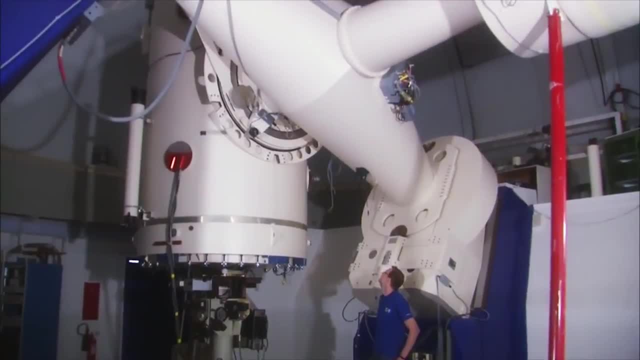 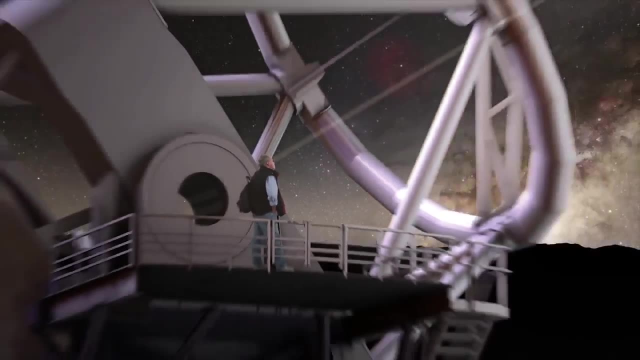 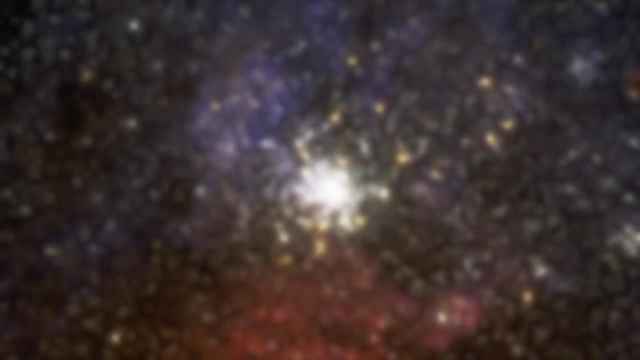 The telescope is, of course, the central tool that allows us to unravel the secrets of the universe. Telescopes collect far more light than the unaided human eye, so they reveal fainter stars and let us peer deeper into space Like magnifying glasses. they also show finer detail. 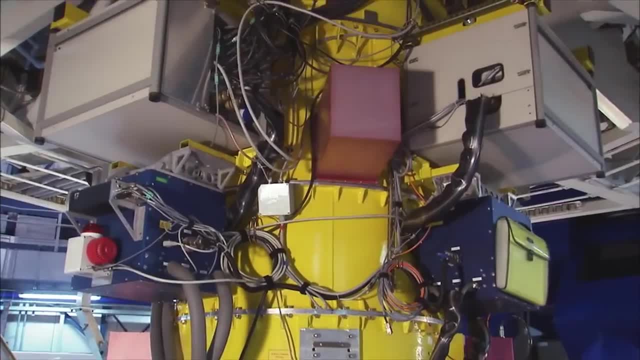 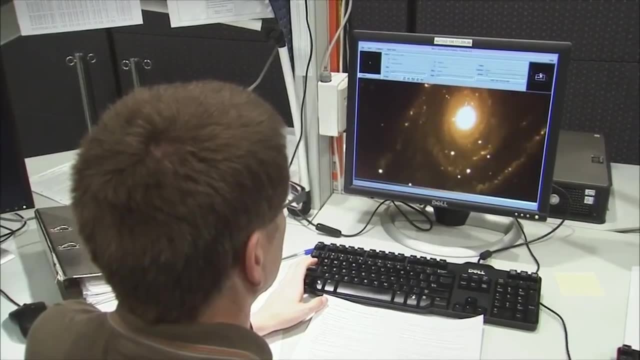 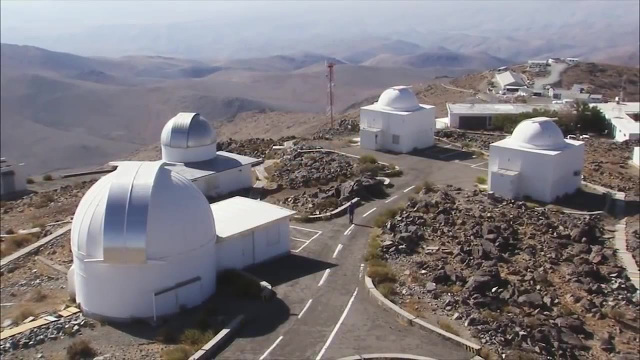 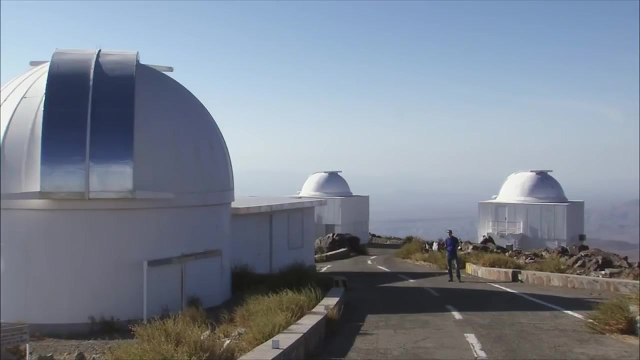 And when equipped with sensitive cameras and spectrographs, they provide us with a wealth of information about planets, stars and galaxies. ESO's first telescopes on La Silla were a mixed bunch. They ranged from small national instruments to large astrographs and wide-field cameras. 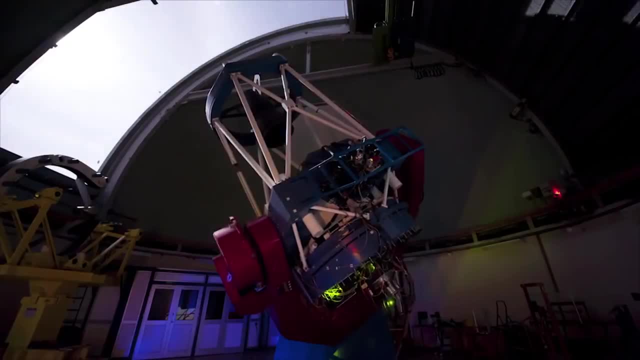 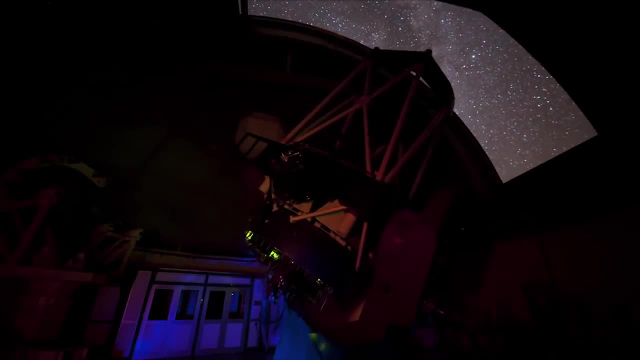 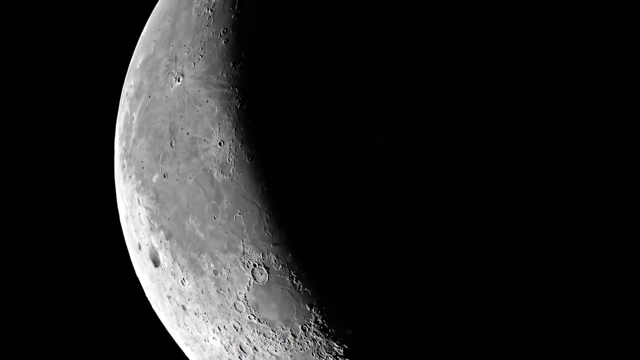 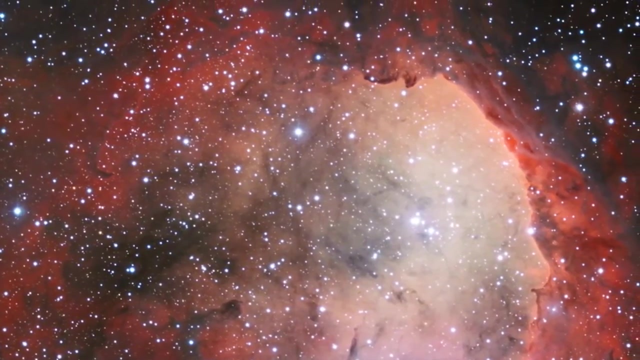 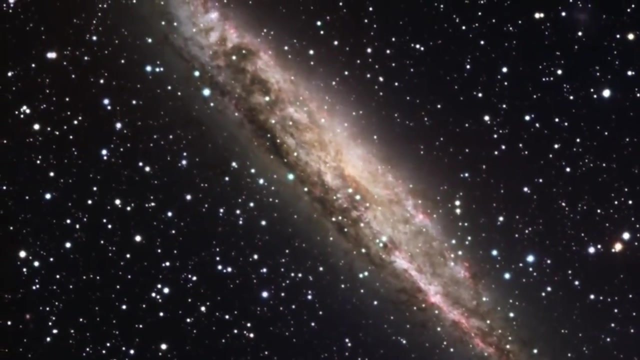 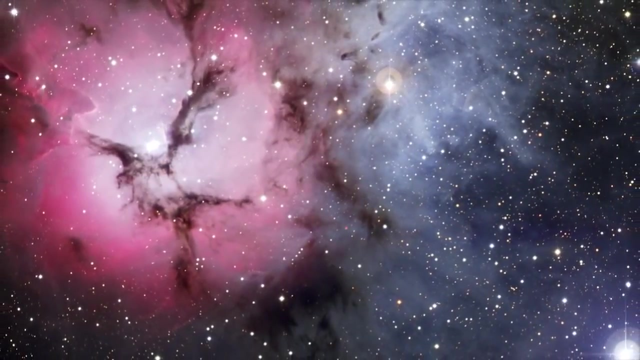 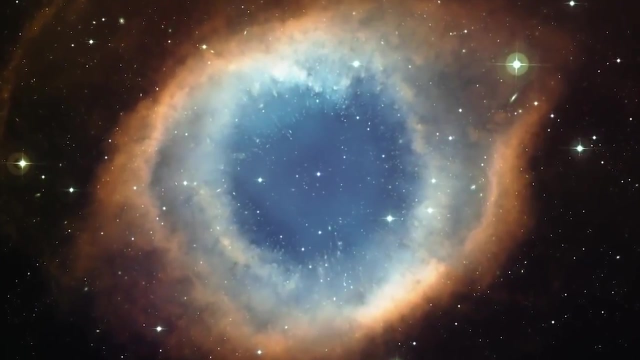 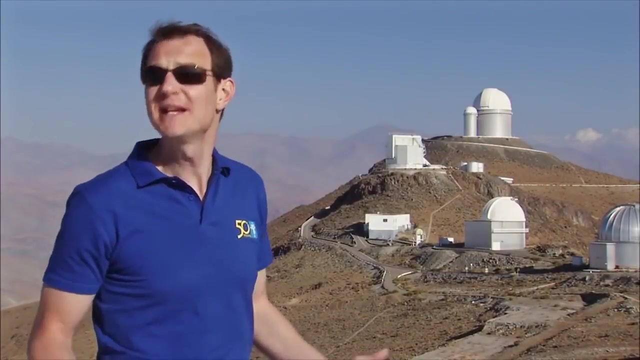 The 2.2-metre telescope, now almost 30 years old, is still producing some of the most dramatic views of the cosmos, TELESCOPES, The Earth. ESO's first telescope, ESA's first telescope, ESA's first telescope. At the highest point of Cerro La Silla lies the biggest achievement of ESO's early years. 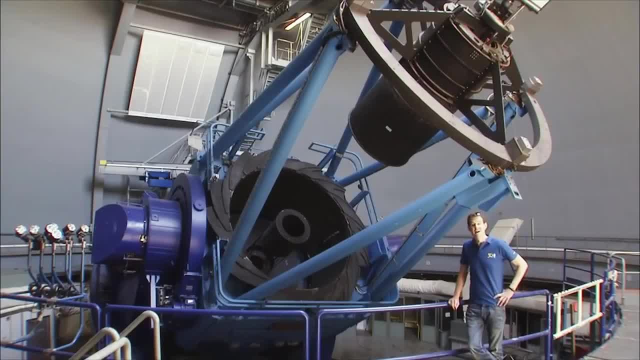 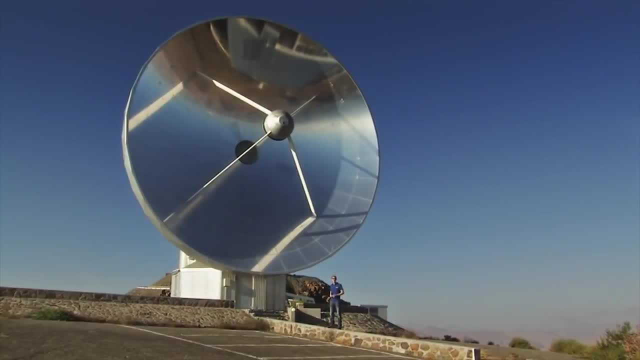 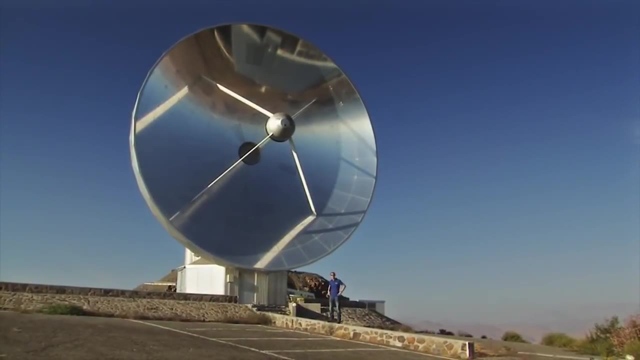 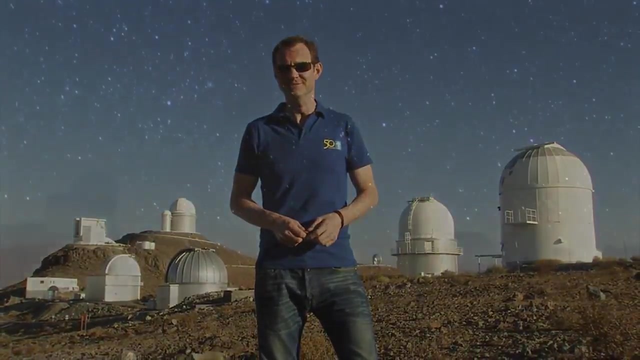 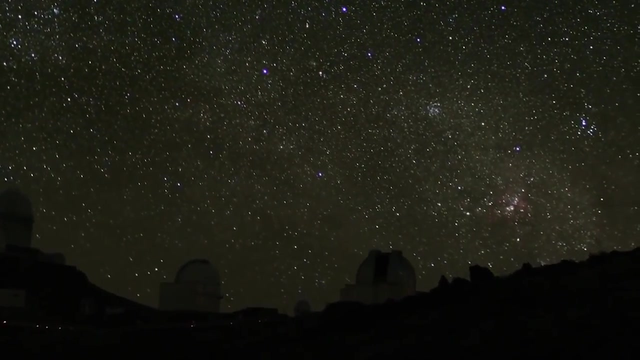 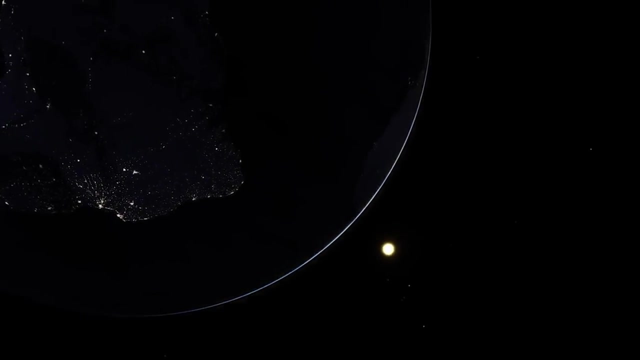 the 3.6-metre telescope. Aged 35,, it now leads a second life as a planet hunter. Also, Swedish astronomers built a shiny dish 15 metres across to study microwaves from cool cosmic clouds. Together, these telescopes have helped to unveil the universe in which we live. 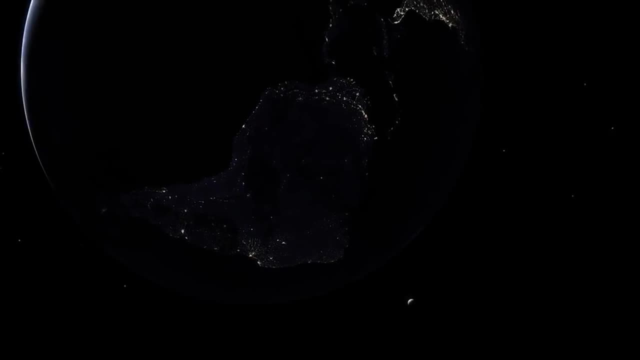 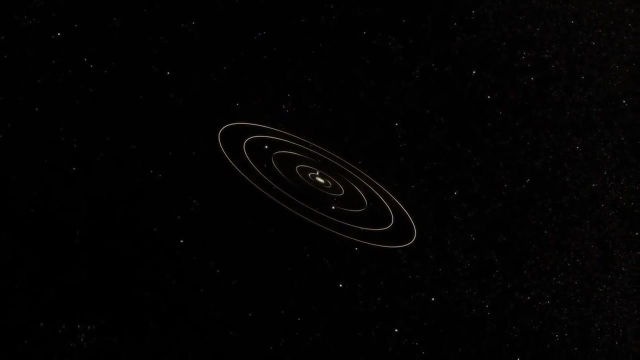 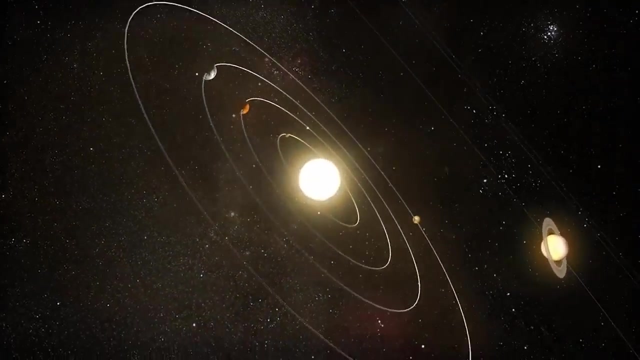 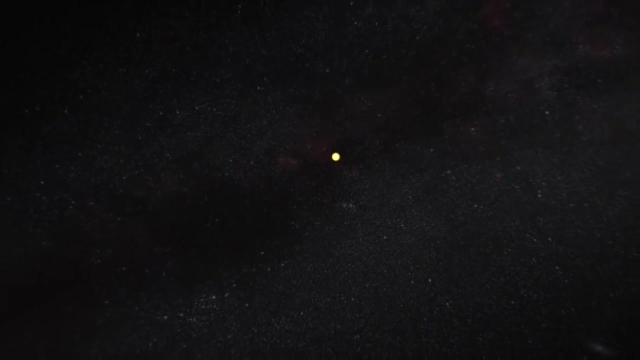 Earth is just one of eight planets in the Solar System. Oh boy buzzer, From tiny Mercury to giant Jupiter. these rocky spheres and gaseous balls are the leftovers of the formation of the Sun. The Sun, in turn, is a middle-of-the-road star in the Milky Way galaxy. 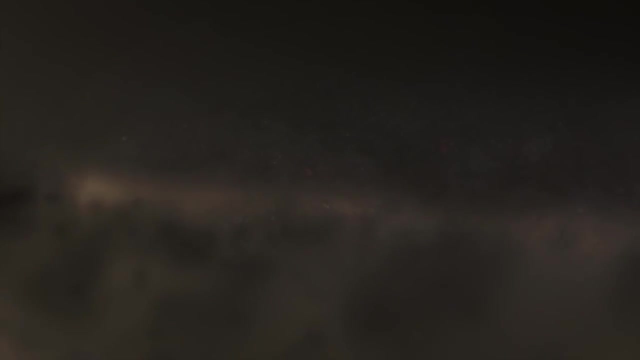 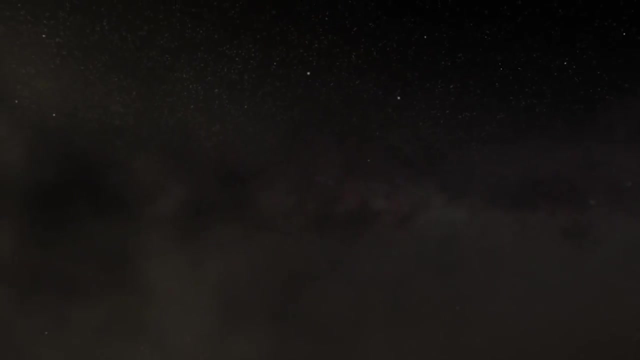 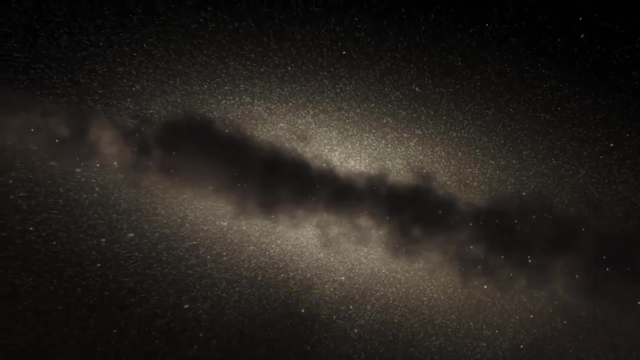 One pinprick of light amidst hundreds of billions of similar stars, as bloated red giants, imploded white dwarfs and rapidly spinning neutron stars. The spiral arms of the Milky Way are sprinkled with glowing nebulae, spawning bright clusters of newborn stars. 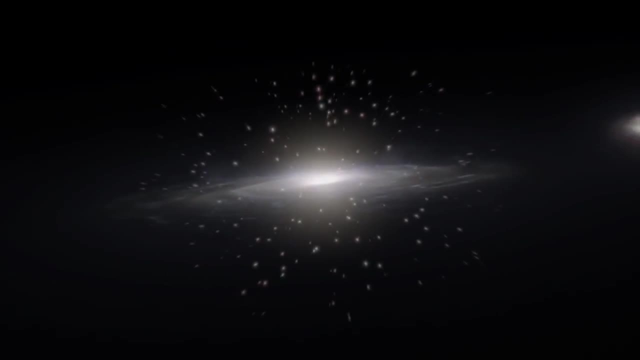 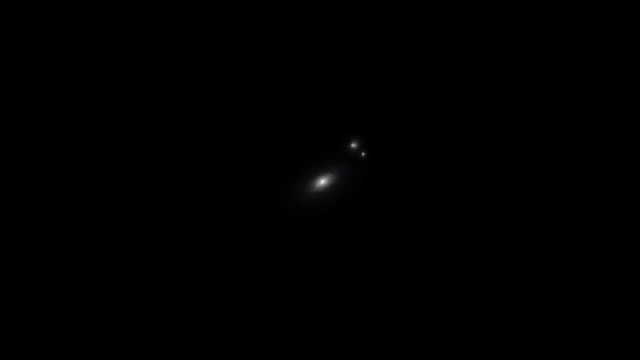 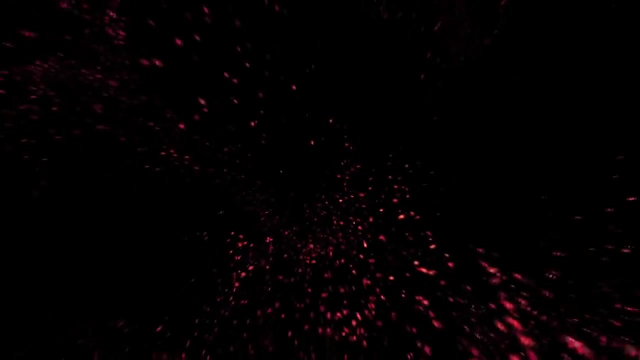 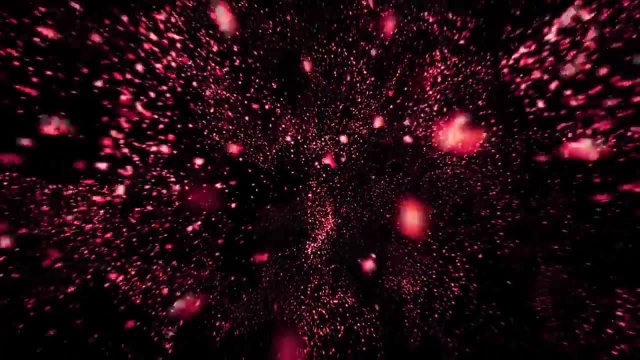 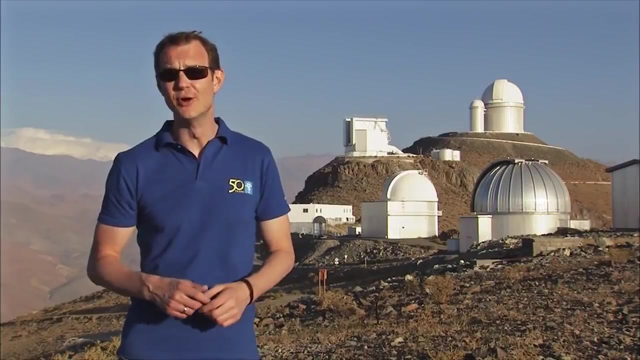 while old globular clusters slowly swarm about the galaxy, And the Milky Way is just one of countless galaxies in a vast universe which has been expanding ever since the Big Bang almost 14 billion years ago. Over the past 50 years, ESA has helped to uncover our place in the universe. 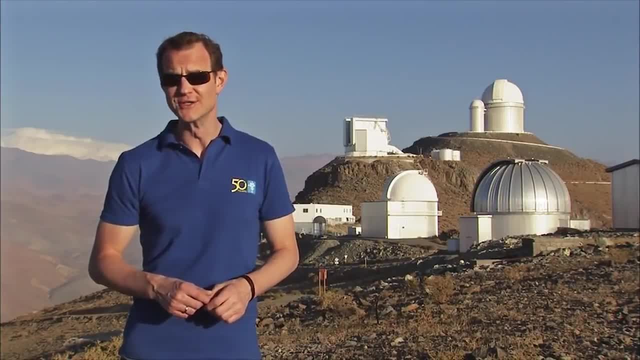 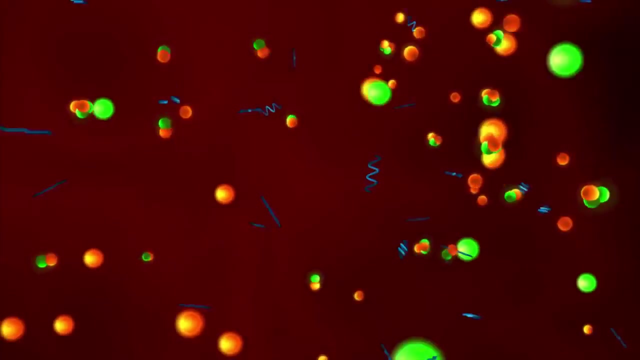 And by looking up, we have also discovered our own origins. We are part of the big cosmic story. Without stars we wouldn't be here. The universe started out with hydrogen and helium, the two lightest elements, But stars are nuclear ovens. 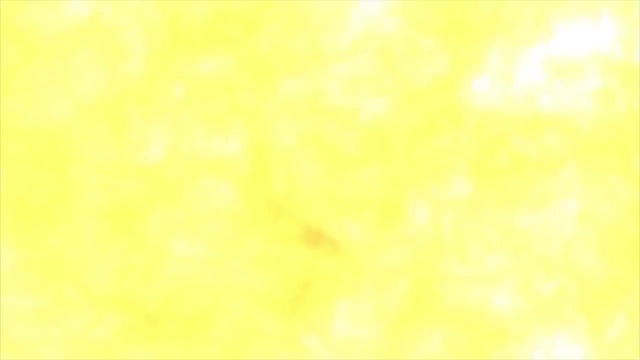 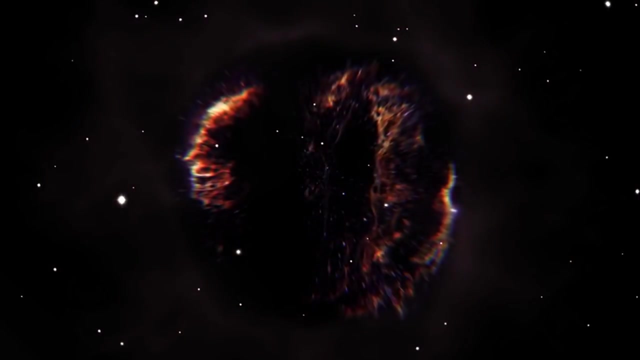 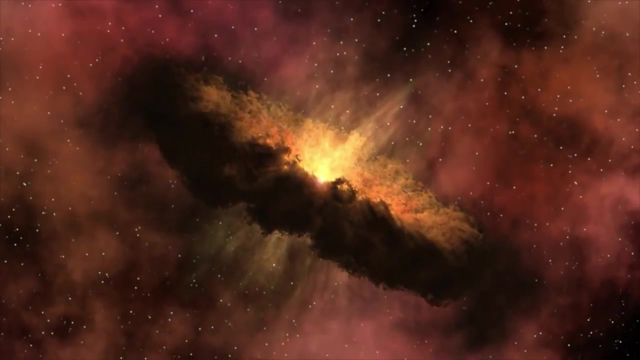 turning light elements into heavier ones, And supernovae like 1987A seed the universe with the products of this stellar alchemy. When the solar system formed some 4.6 billion years ago, the universe was formed It contained trace amounts of these heavier elements. 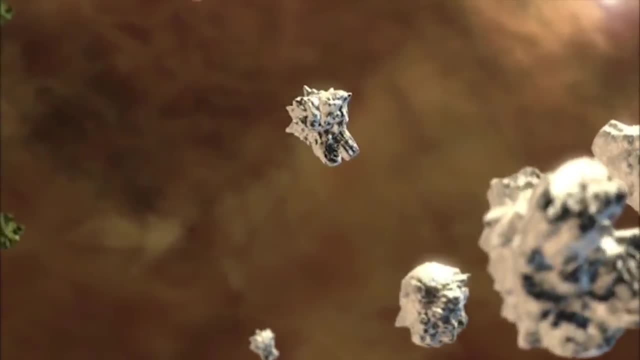 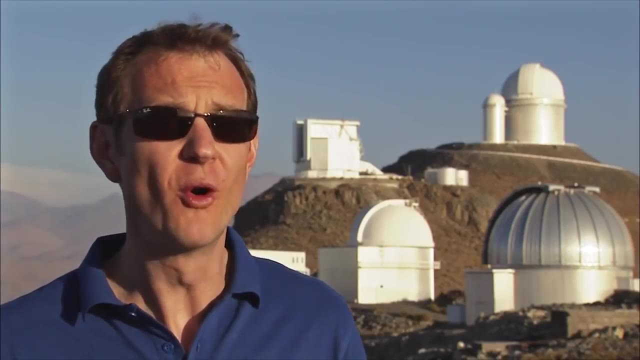 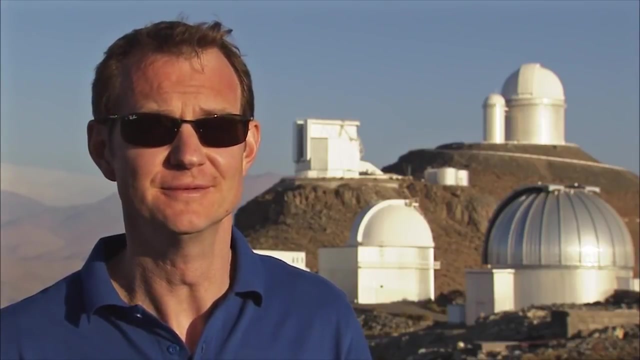 Metals and silicates, but also carbon and oxygen. The carbon in our muscles, the iron in our blood and the calcium in our bones were all forged in an earlier generation of stars. You and I were literally made in heaven, But answers always lead to new questions. 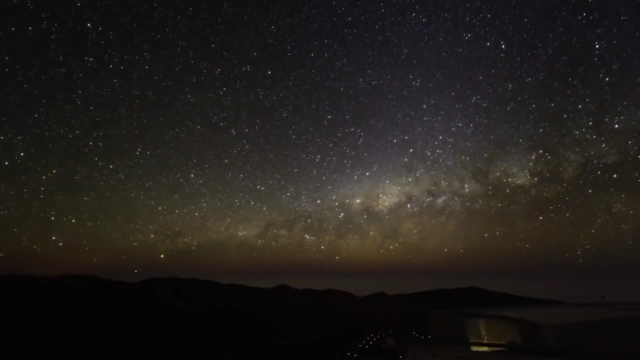 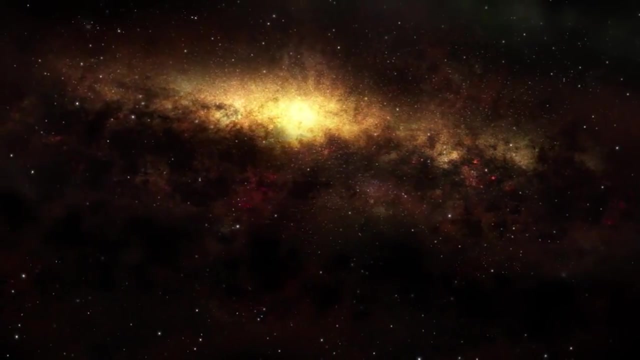 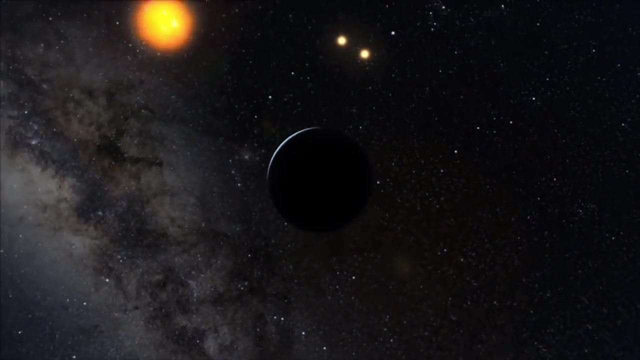 The more we learn, the deeper the mystery. The more you try, The more we run, the deeper the mysteries become. What is the origin and ultimate fate of galaxies? Are there other solar systems out there, And could there be life on alien worlds? 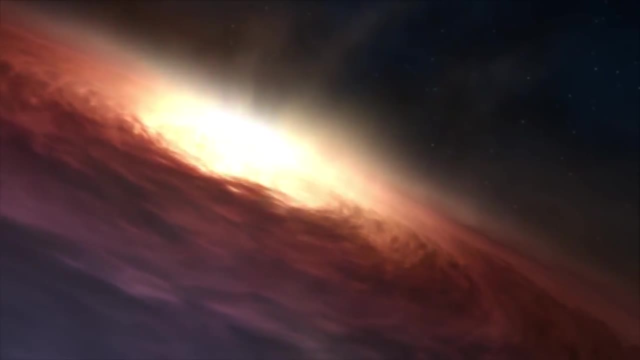 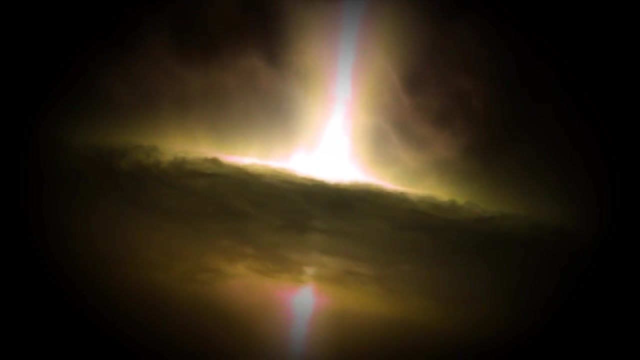 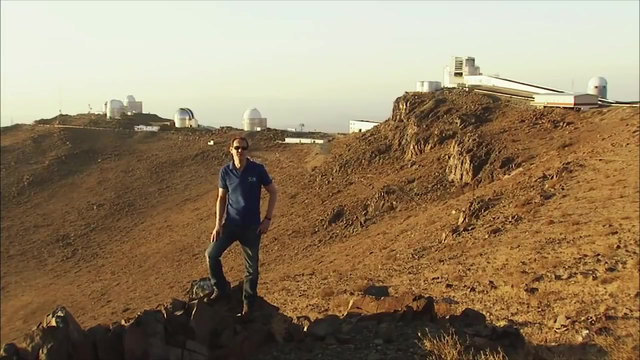 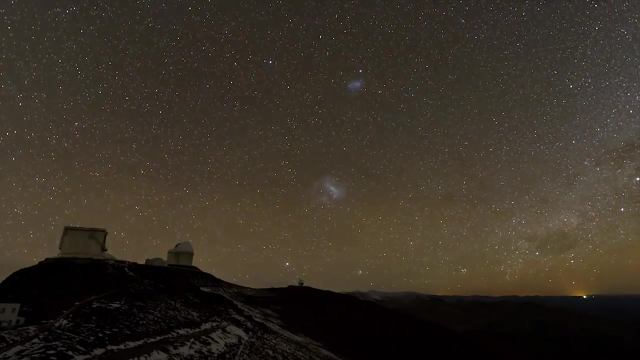 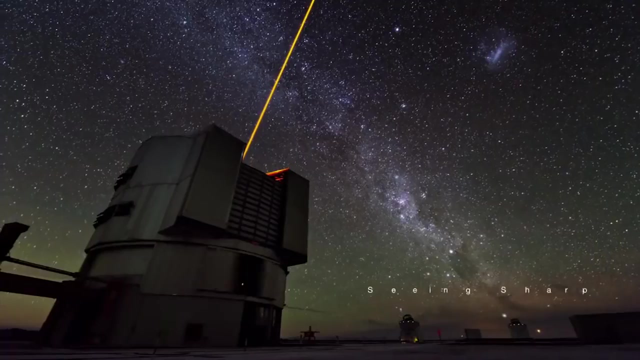 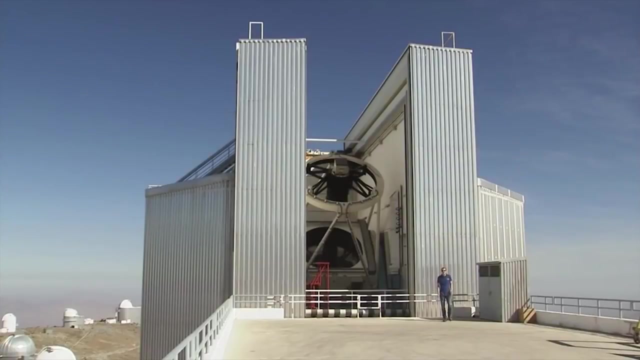 And what lurks in the dark heart of our Milky Way galaxy. Astronomers were clearly in need of more powerful telescopes, and ESO provided them with revolutionary new tools. Bigger is better, at least when it comes to telescope mirrors, But larger mirrors have. 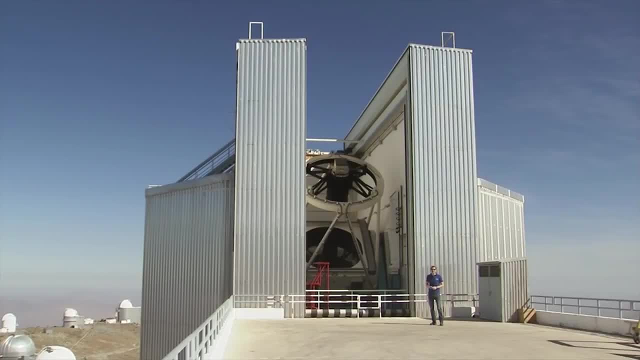 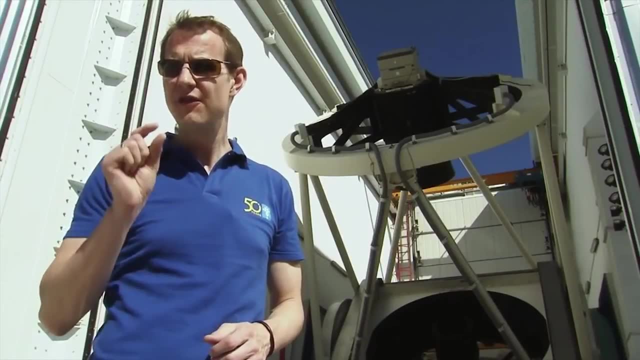 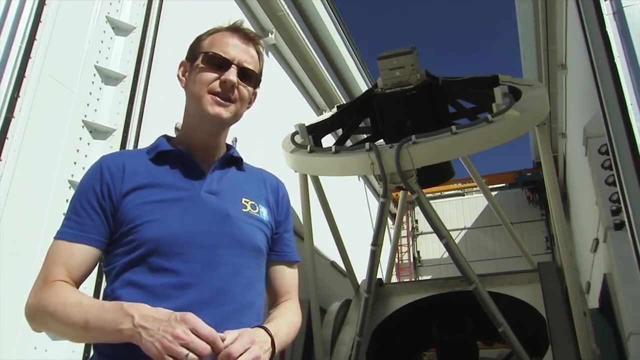 to be thick so that they don't deform under their own weight. And really large mirrors deform anyway, no matter how thick and heavy they are. The solution: Thin, lightweight mirrors and a magic trick called active optics. ESO pioneered this technology in the last century. 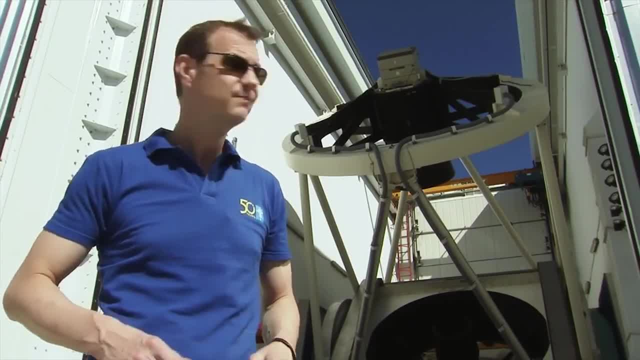 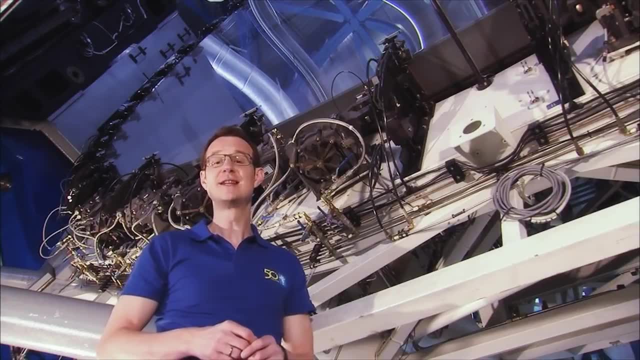 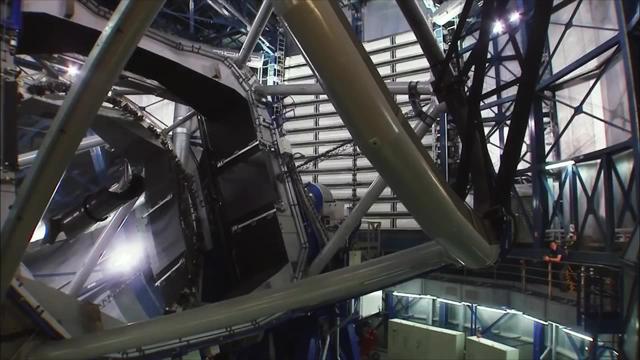 And this is the state of the art. The mirrors of the Very Large Telescope, the VLT, are 8.2 metres across, but only 20 centimetres thick. And here's the magic: A computer-controlled support system ensures that the mirror keeps. 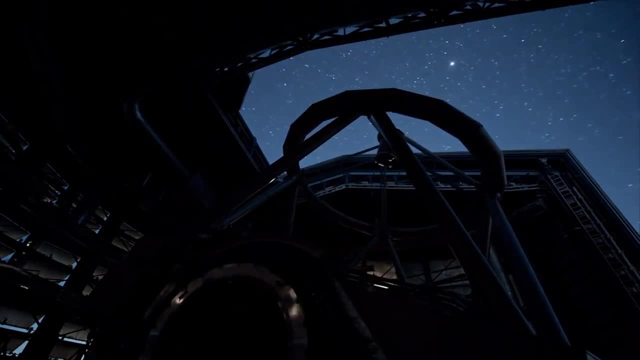 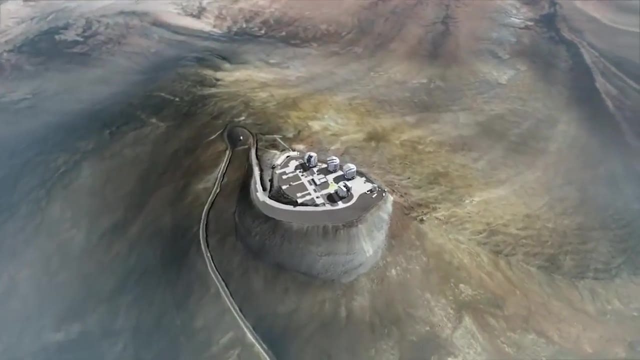 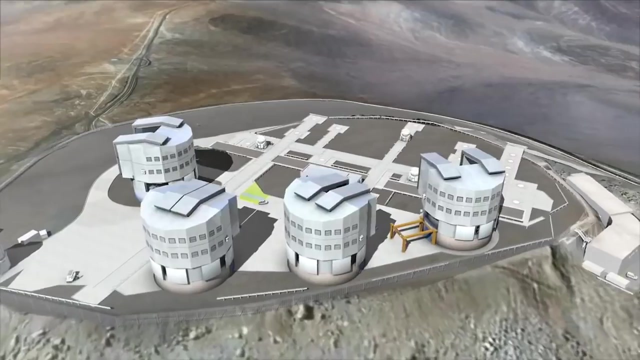 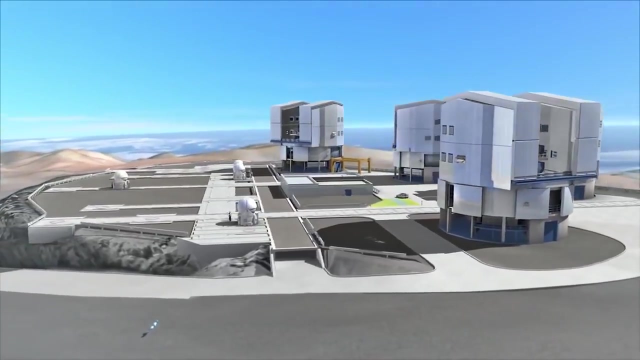 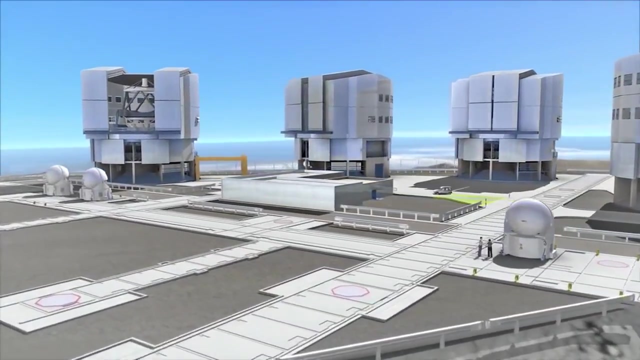 its desired shape at all times, to nanometre precision. The VLT is ESO's flagship facility: Four identical telescopes joining forces on top of Cerro Paranal in the north of Chile. Built in the late 1990s, they provided astronomers. 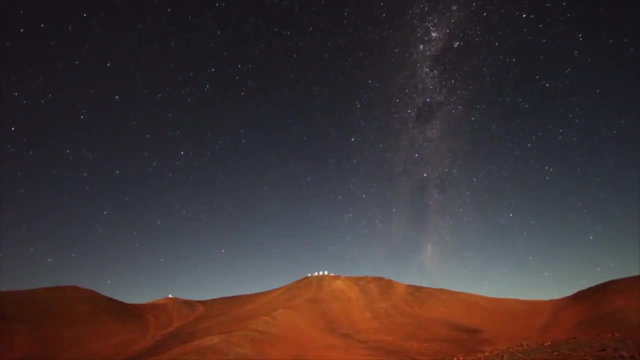 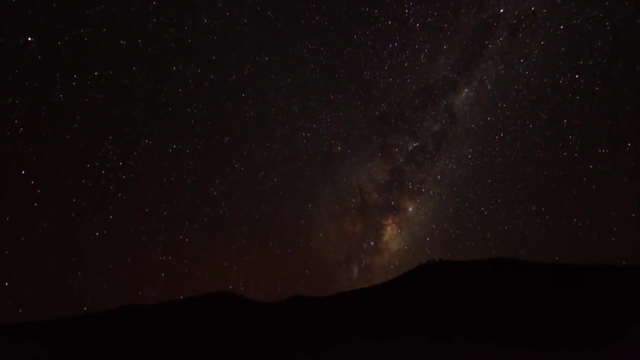 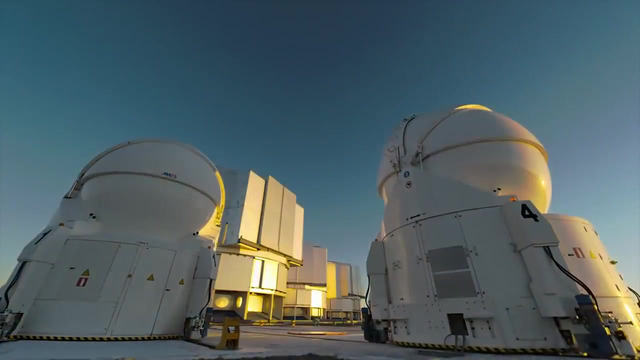 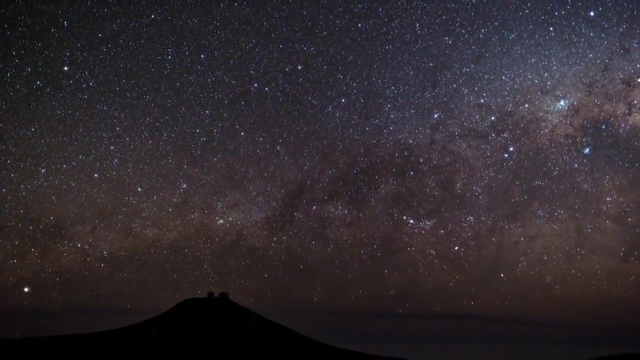 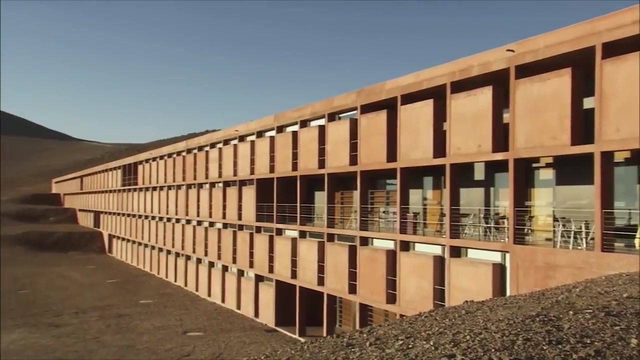 with the best available technologies. In the middle of the Atacama Desert, ESO created an astronomers' paradise. Scientists stay in La Residencia, a guest house partly built by scientists as part of buried under the dirt and rubble of one of the driest places on the planet. 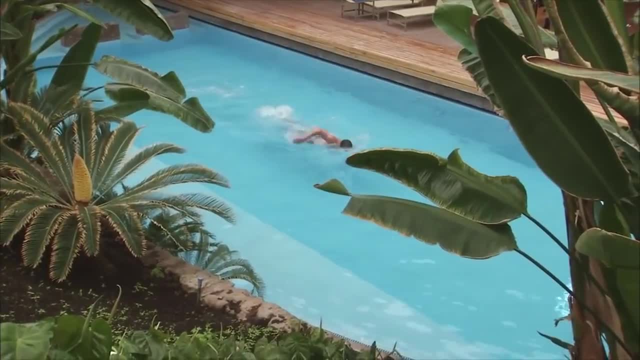 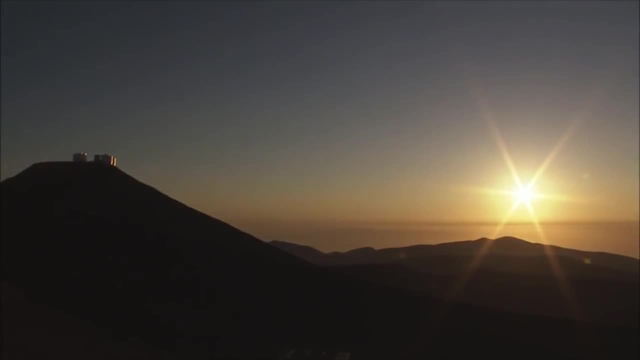 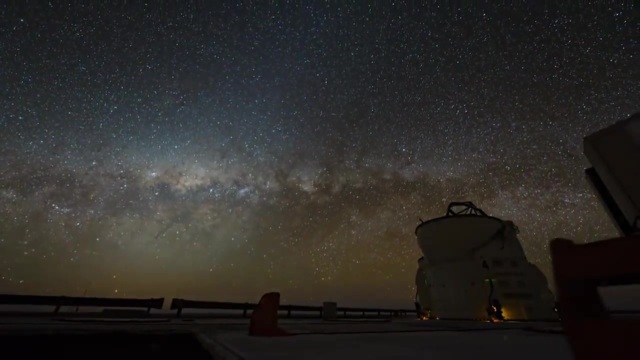 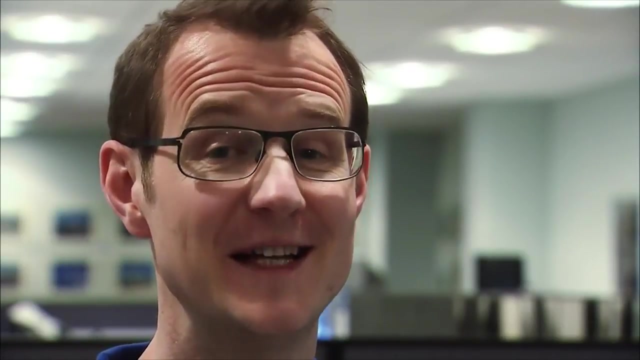 But inside are lush palm trees, a swimming pool and delicious Chilean sweets. Of course, the unique selling point of the Very Large Telescope is not its swimming pool, but its unequalled view of the Universe. Without thin mirrors and active optics, the VLT wouldn't be possible. 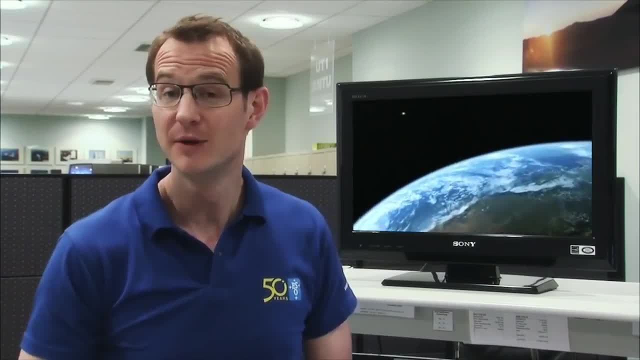 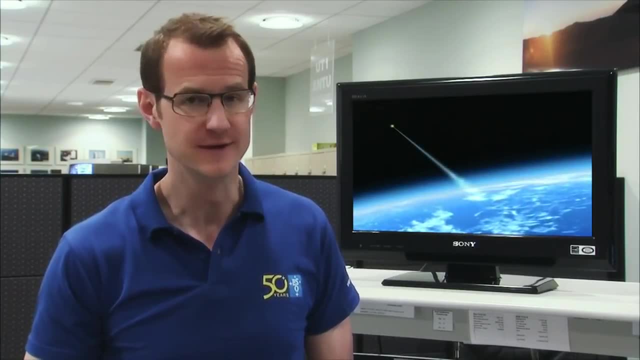 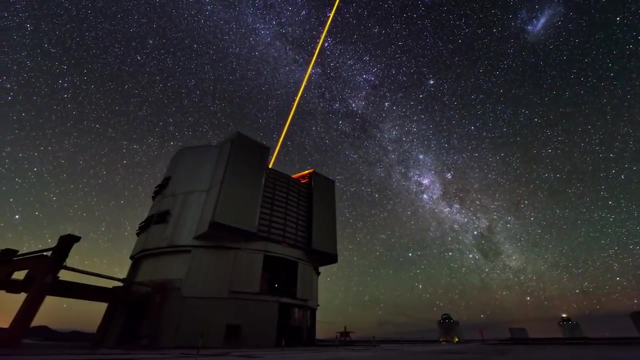 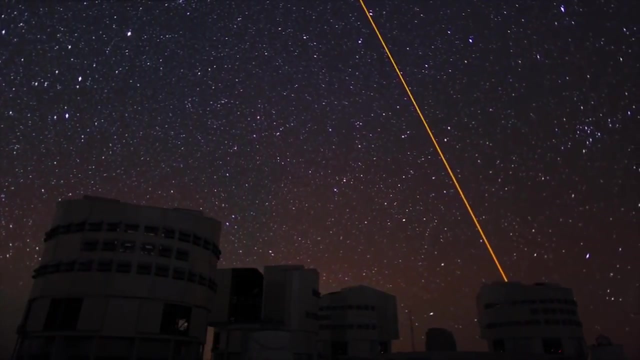 But there's more. Stars appear blurry even when observed with the best and largest telescopes. The reason: The Earth's atmosphere distorts the images. Enter the second magic trick: adaptive optics On. Paranal laser beams shoot out into the night sky to create artificial stars. 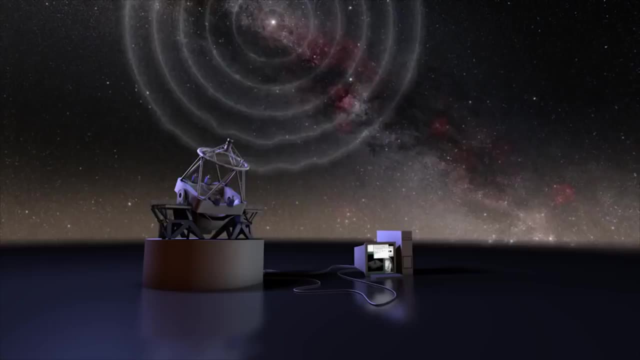 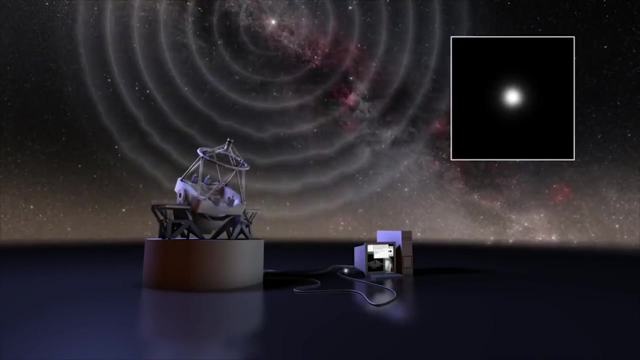 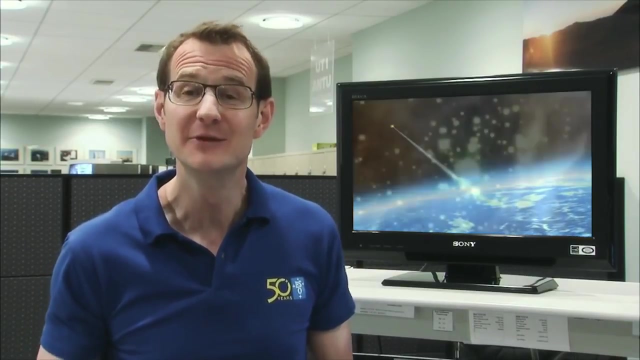 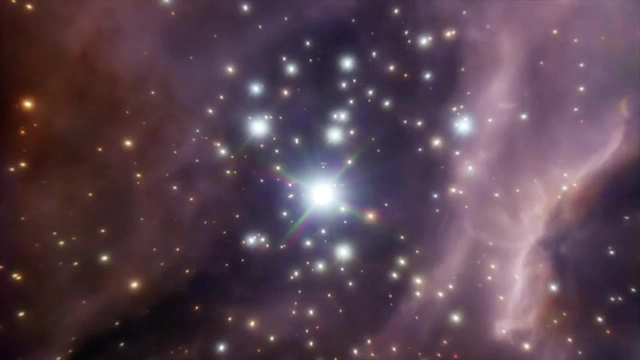 Sensors use these stars to measure the atmospheric distortions, And hundreds of times per second. the image is corrected by computer-controlled deformable mirrors, And the end effect? As if the turbulent atmosphere were completely removed. Just look at the difference. The Milky Way is a giant spiral galaxy. 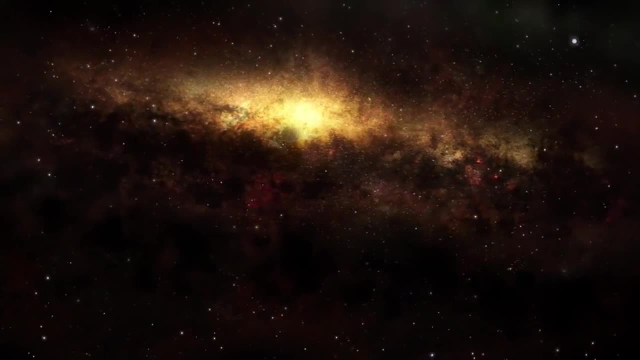 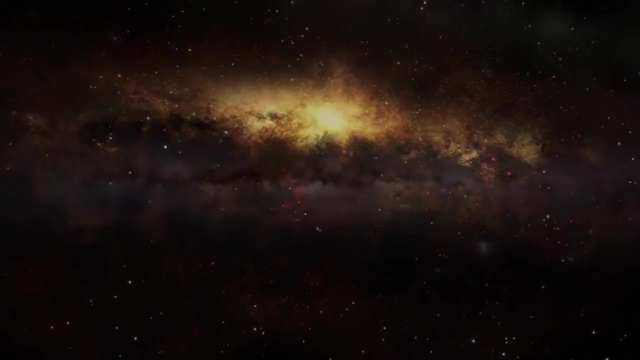 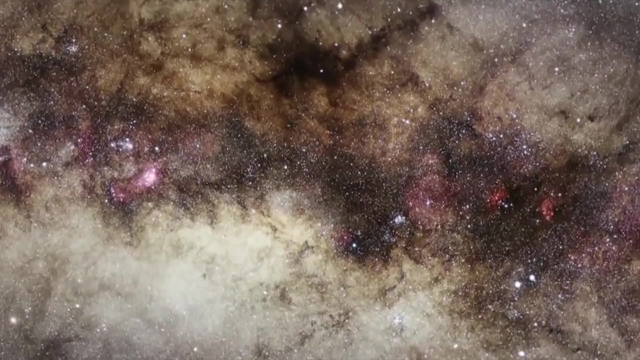 And at its core, 27,000 light-years away, lies a mystery that ESO's Very Large Telescope helped to unravel. Massive dust clouds block our view of the Milky Way's core, But sensitive infrared cameras can peer through the dust and uncover what lies behind. 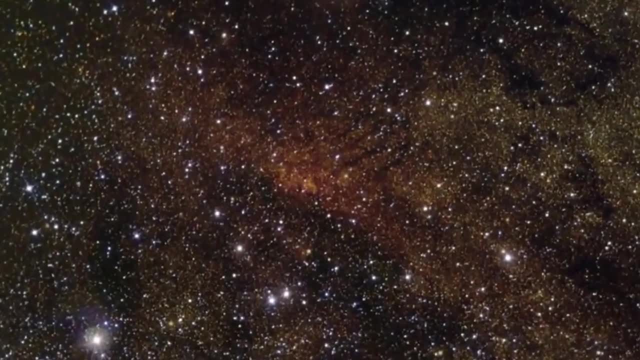 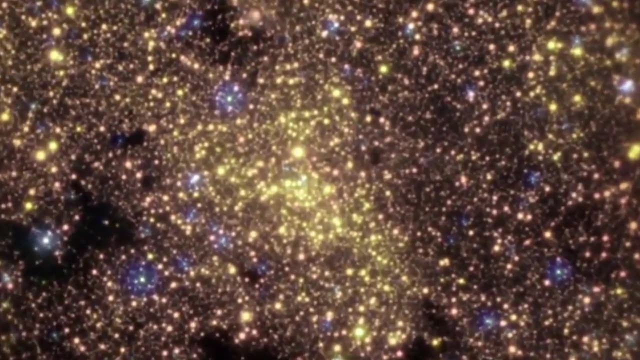 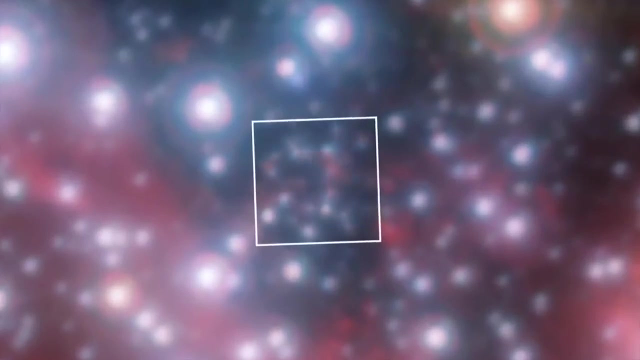 The Milky Way is a giant spiral galaxy And it's the largest star in the Universe. Assisted by adaptive optics, they reveal dozens of red giant stars And over the years, these stars are seen to move. They orbit an invisible object at the very centre of the Milky Way. 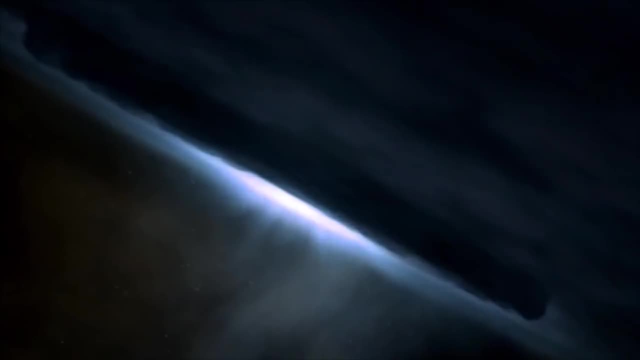 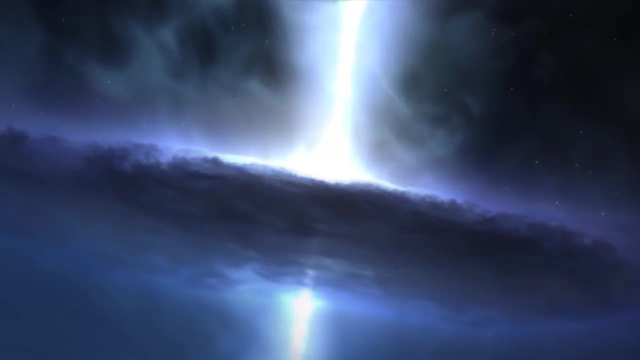 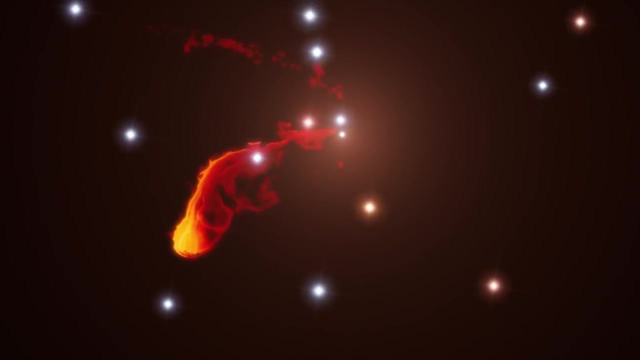 Judging from the stellar motions, the invisible object must be extremely massive, A monstrous black hole Weighing in at 4.3 million times the mass of our Sun. Astronomers have even observed energetic flares from gas clouds falling into the black hole. 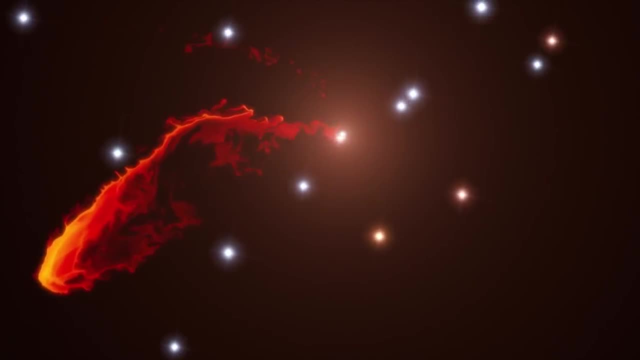 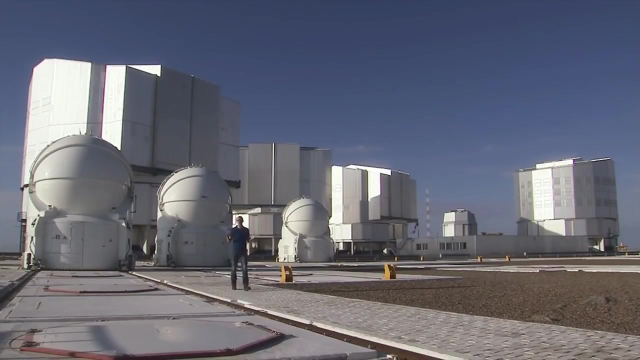 All exposed by the sheer power of adaptive optics. So thin mirrors and active optics make it possible to build giant telescopes, And the adaptive optics take care of the atmospheric turbulence, providing us with extremely sharp images. But we're not done yet with our magic tricks. 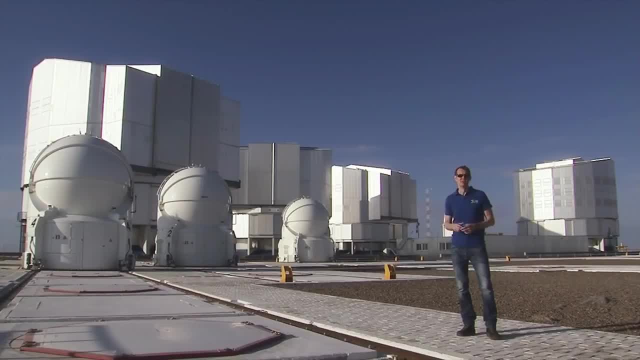 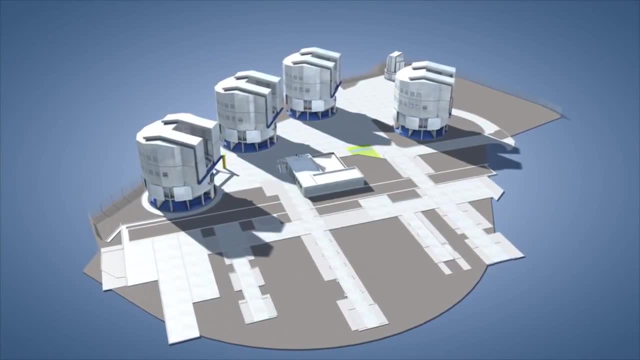 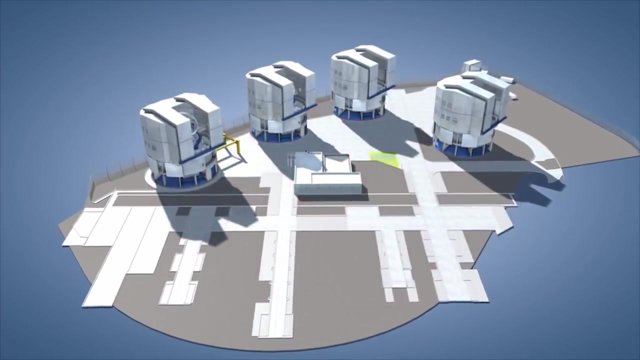 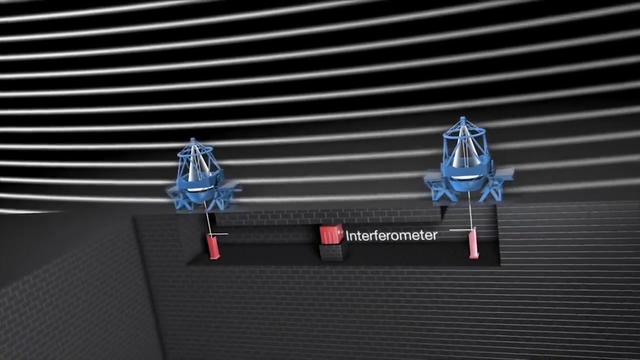 There's a third one, And it's called interferometry. The VLT consists of four telescopes. Together, they can act as a virtual telescope measuring 130 metres across. Light collected by the individual telescopes is channelled through tunnels and brought together in an underground laboratory. 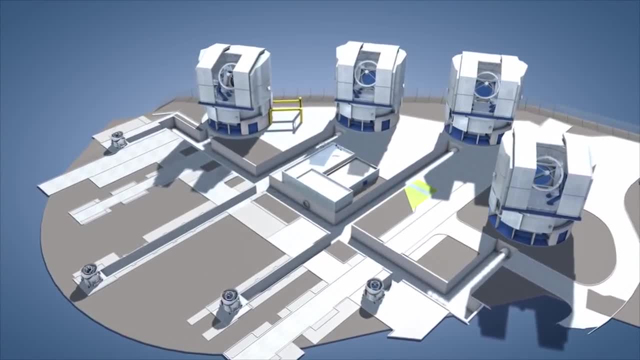 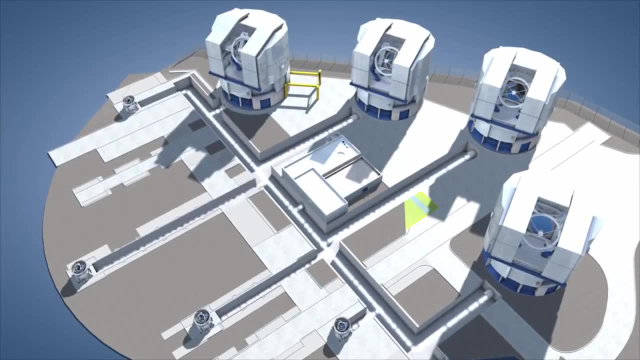 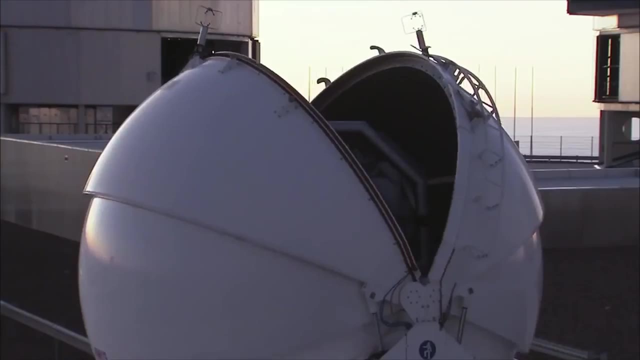 Here the light waves are combined using laser metrology and intricate delay lines. The net result is the light-gathering power of four 8.2 metre mirrors And the eagle-eyed vision of an imaginary telescope as large as 50 tennis courts. 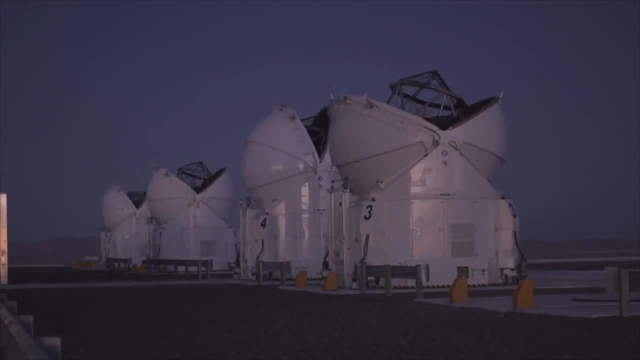 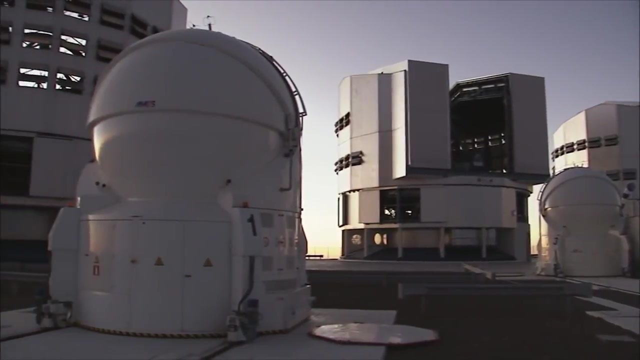 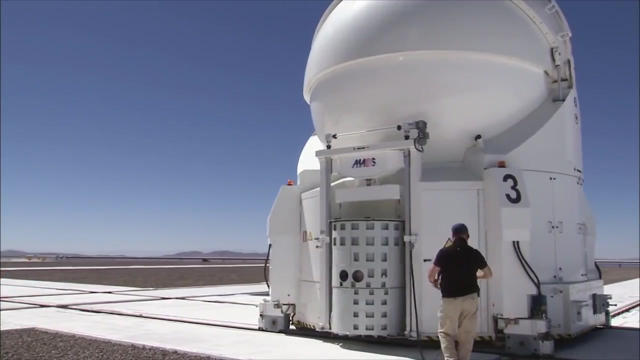 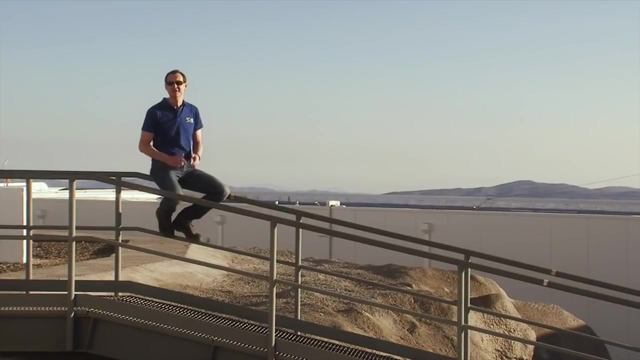 Four auxiliary telescopes give the network more flexibility. They may appear tiny next to the four giants, yet they sport mirrors 1.8 metres across. That's bigger than the largest telescope in the world just 100 years ago. Optical interferometry is something of a miracle. 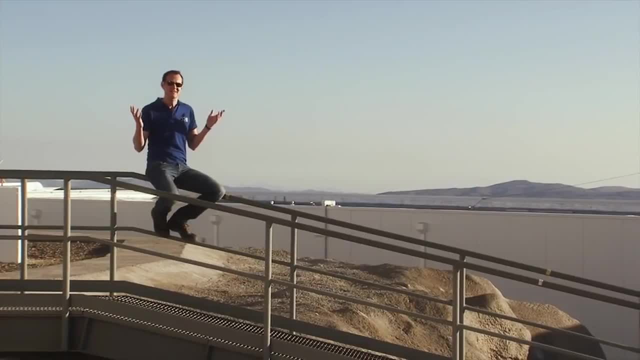 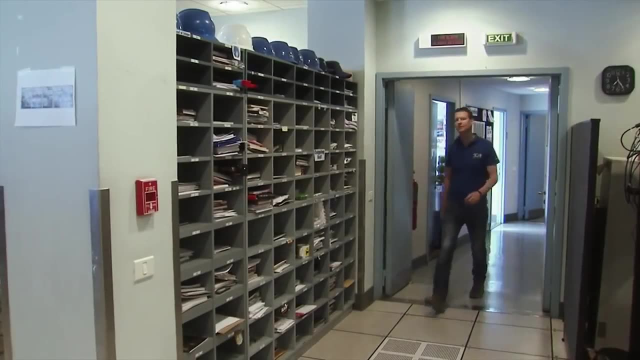 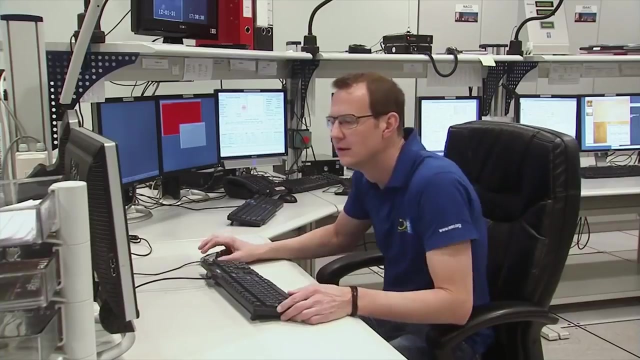 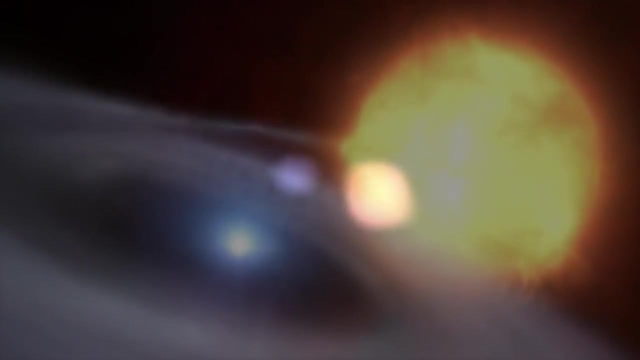 Starlight magic wielded in the desert, And the results are impressive. The Very Large Telescope interferometer reveals 50 times more detail than the Hubble telescope. For instance, it gave us a close-up of a vampire double star. One star is stealing material from its companion. 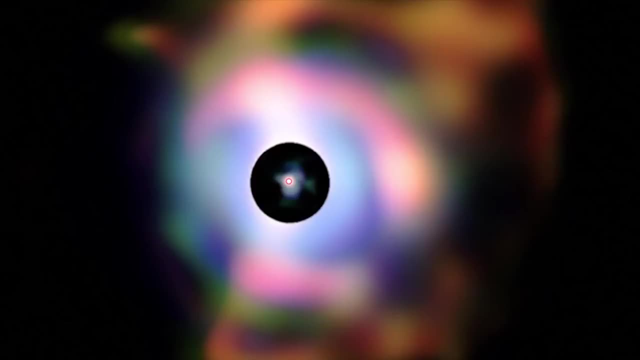 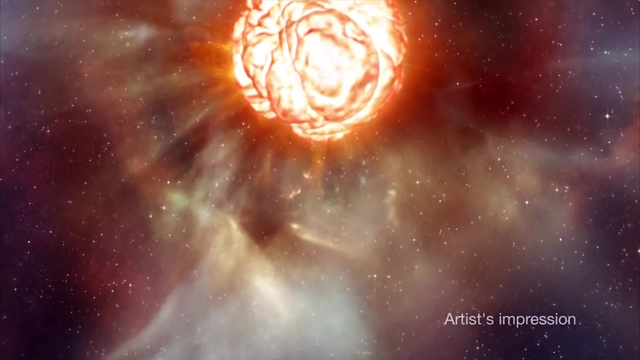 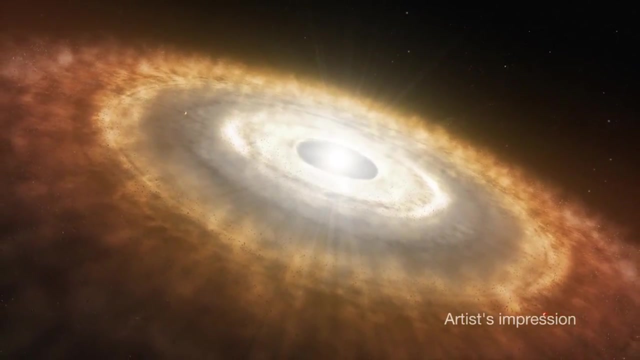 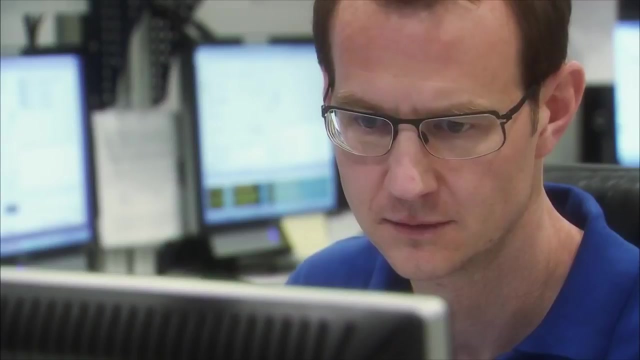 And one star is stealing material from its companion. Irregular paths of stardust have been detected around Betelgeuse, a stellar giant about to go supernova, And in dusty disks surrounding newborn stars, astronomers have found the raw material of future Earth-like worlds. 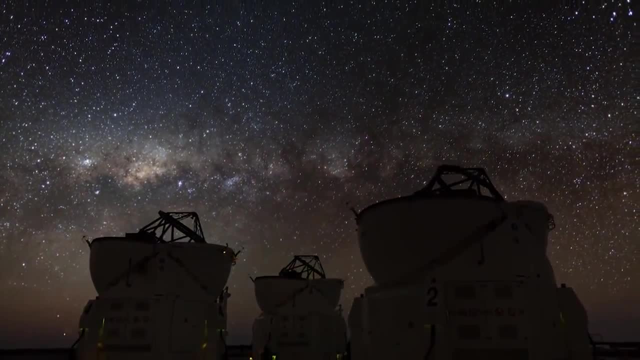 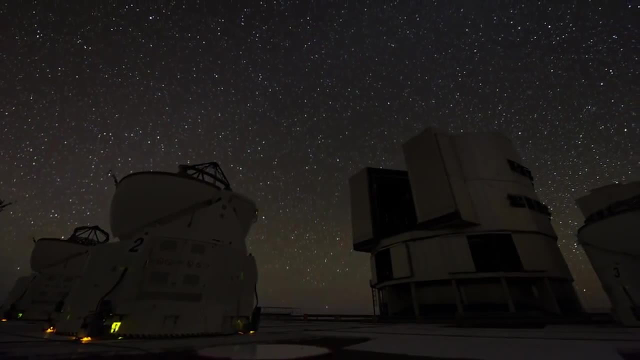 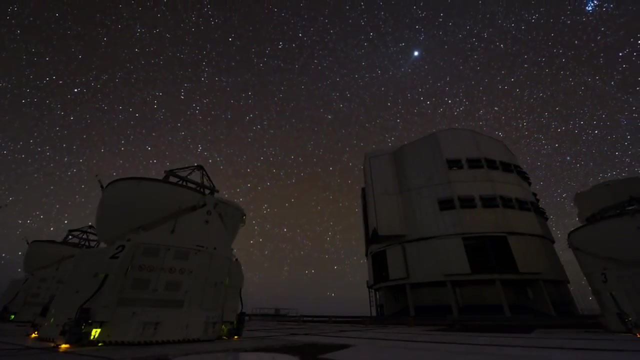 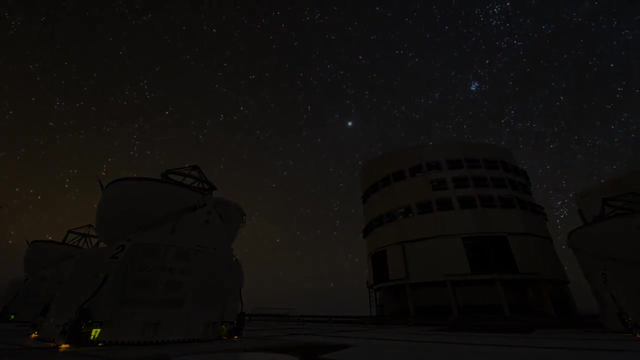 The Very Large Telescope is mankind's sharpest eye on the sky, But astronomers have other means to expand their horizons and broaden their views. At the European Southern Observatory, they have learned to see the Universe in a completely different kind of light. So where do we go? 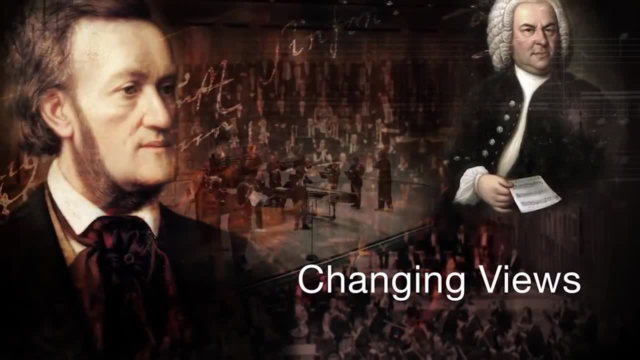 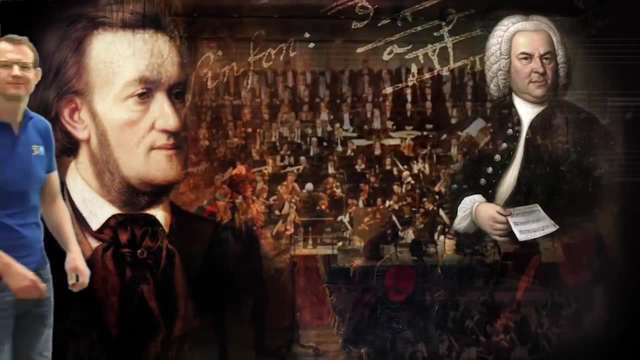 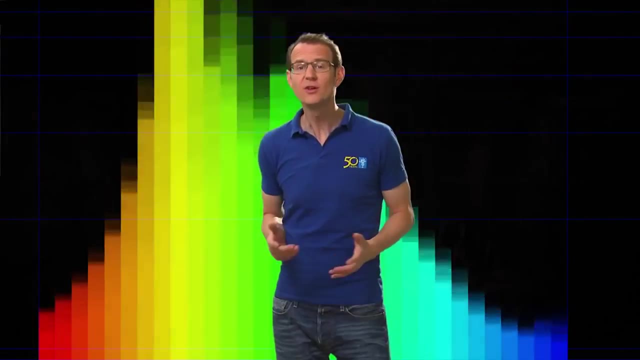 The mostatmospheric telescope of Earth's orbit. We're off to a great trip. It's only just a few days away in the system. Great music, isn't it? But suppose you had a hearing impairment. What if you couldn't hear the low frequencies? 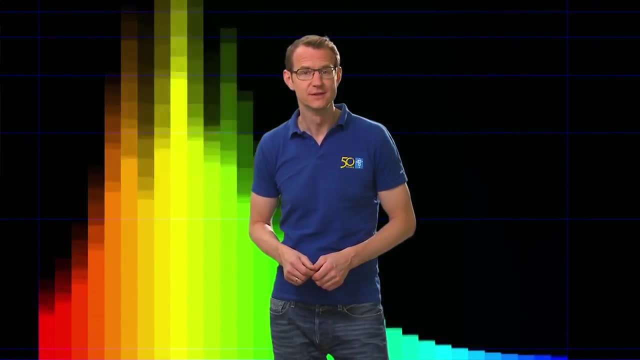 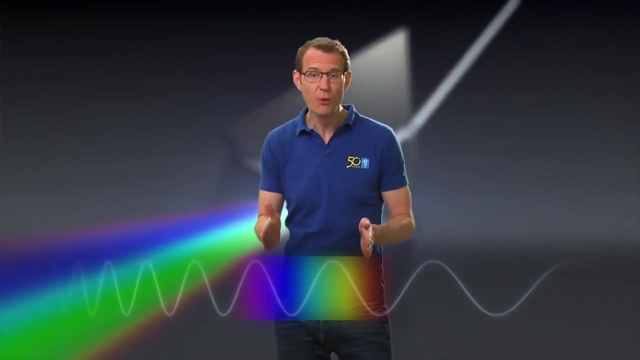 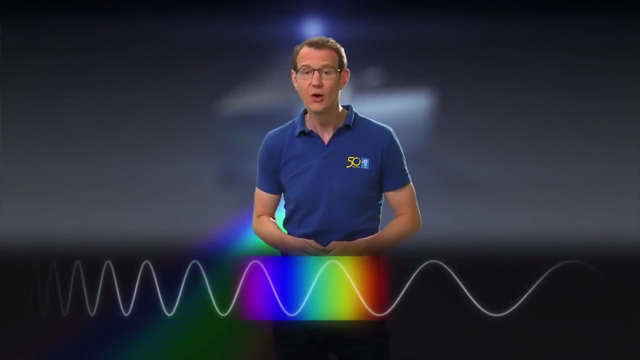 Or the high frequencies. Astronomers used to be in a similar situation. The human eye is only sensitive to a small part of all the radiation in the universe. We can't see light with wavelengths shorter than violet waves or longer than red waves. 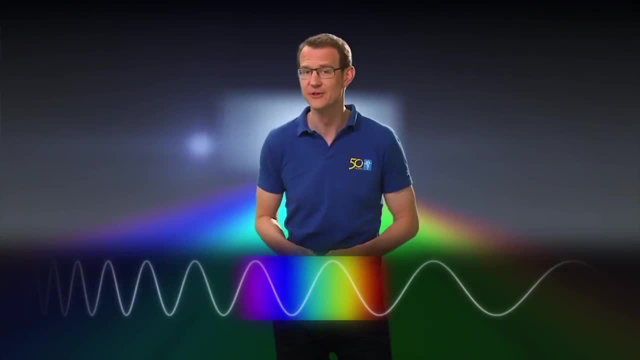 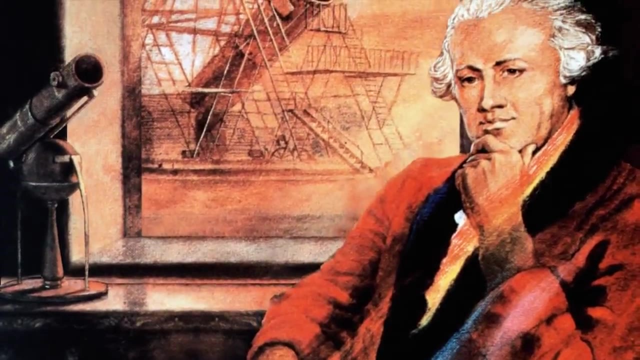 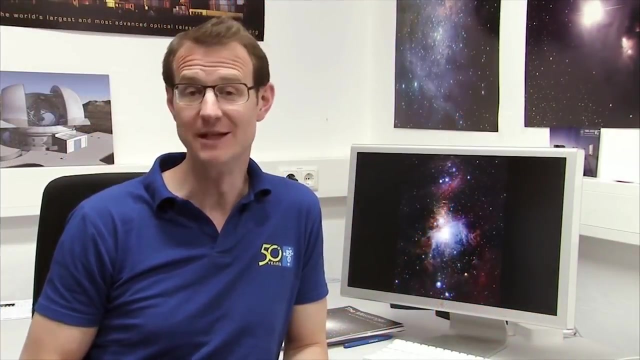 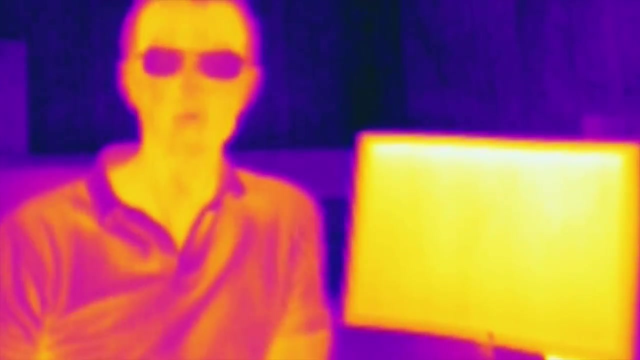 We just don't perceive the whole cosmic symphony. Infrared or heat radiation was first discovered by William Herschel in 1800.. In a dark room you can't see me, But put on infrared goggles and you can see my body warmth. 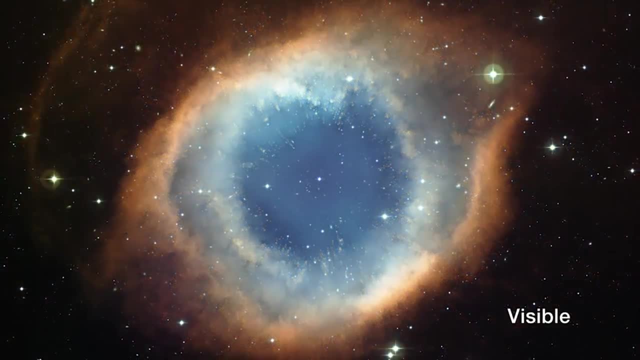 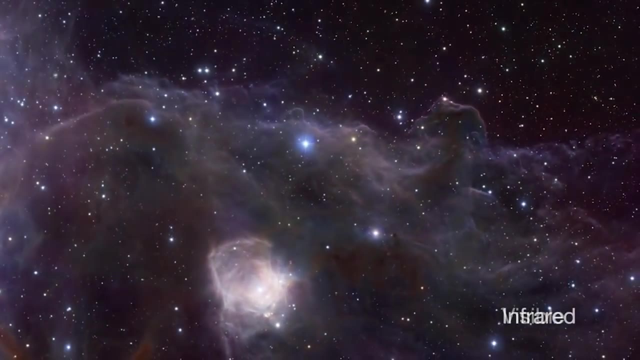 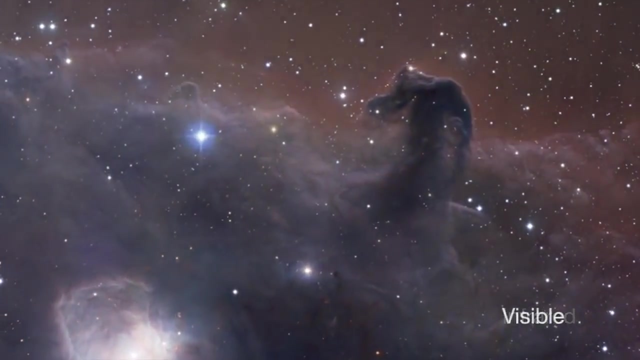 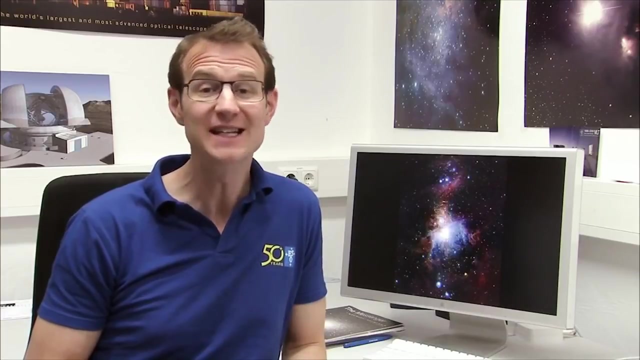 Likewise, infrared telescopes reveal cosmic objects too cool to give off visible light, like dark clouds of gas and dust where stars and planets are born. For decades, ESO astronomers have been keen to explore the universe at infrared wavelengths, But the first detectors were small and hence inefficient. 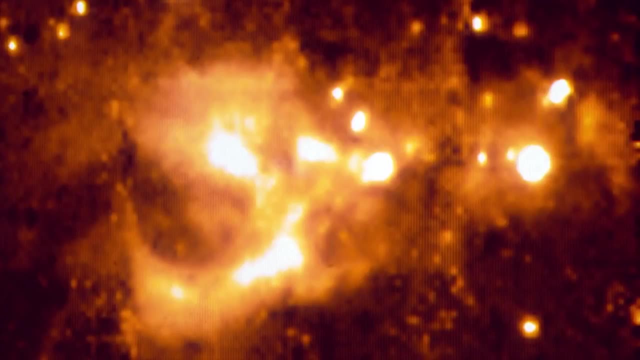 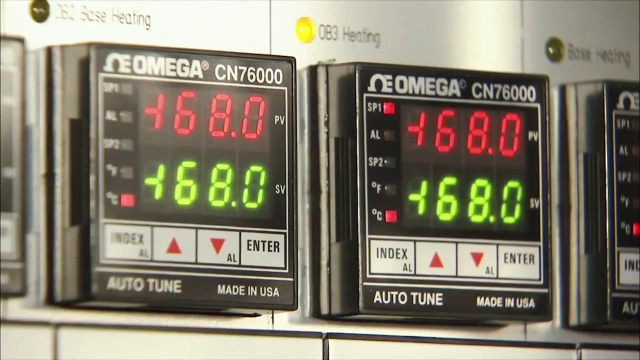 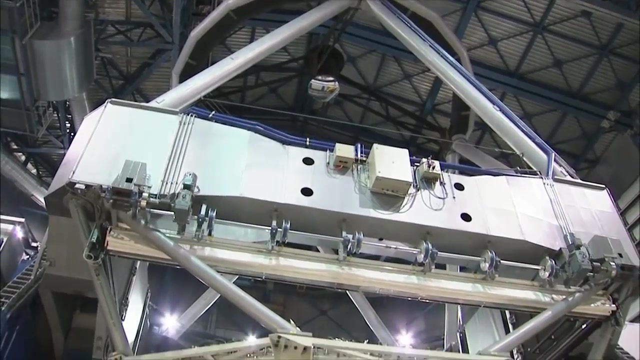 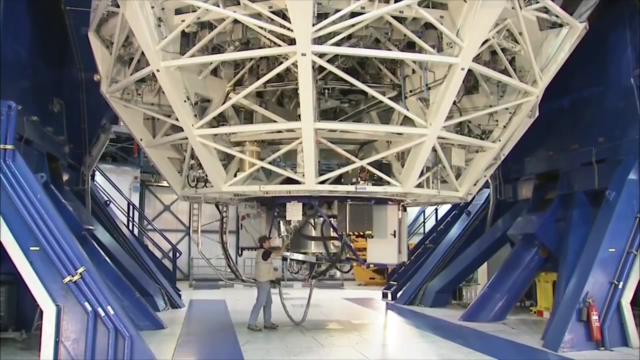 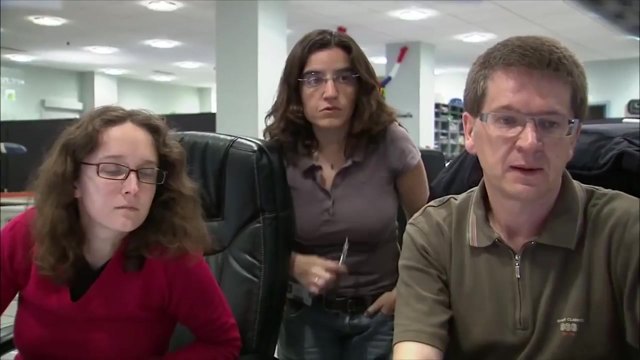 They gave us a blurry view of the infrared sky. Today's infrared cameras are huge and powerful. They're cooled to very low temperatures to increase their sensitivity, And ESO's Very Large Telescope is designed to make good use of them. In fact, some of its technological tricks, like interferometry, only work in the infrared. 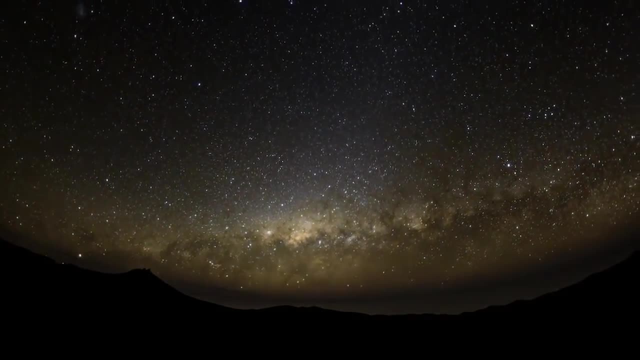 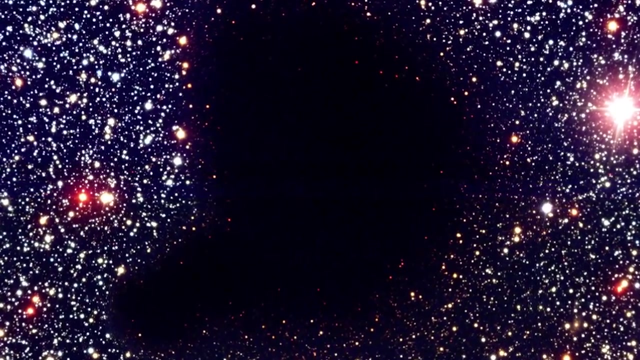 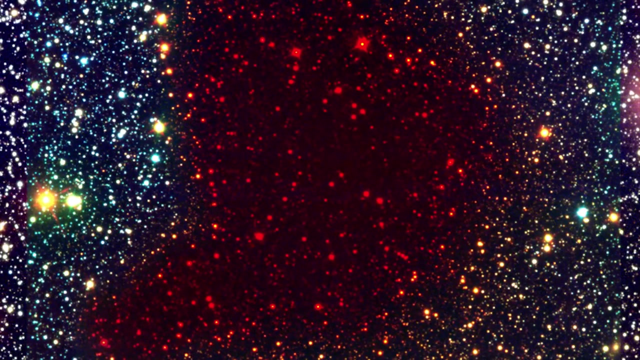 We've broadened our view to reveal the universe in a new light. This dark blob is a cloud of cosmic dust. It blots out the stars in the background, But in the infrared we can look straight through the dust, And here's the Orion Nebula, a stellar nursery. 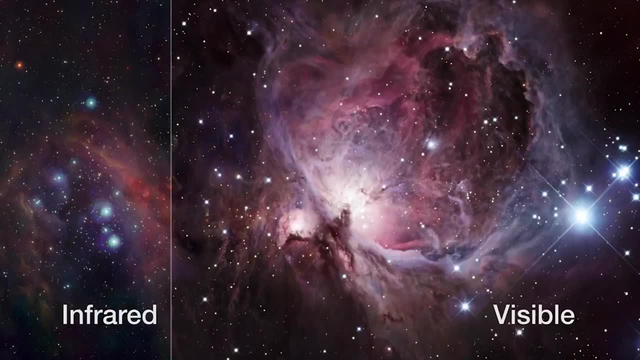 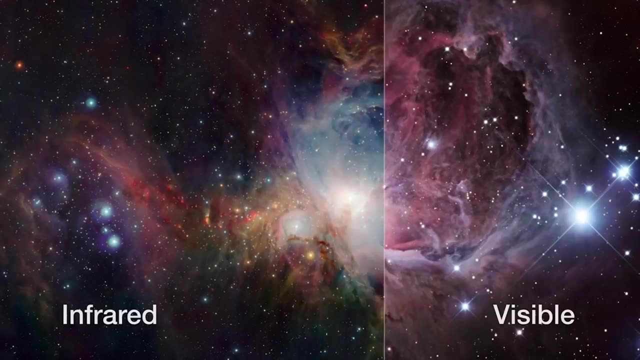 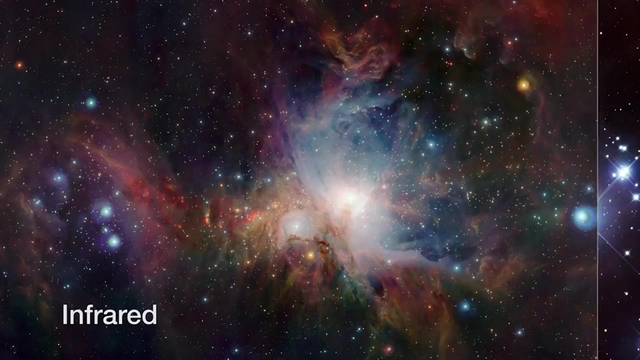 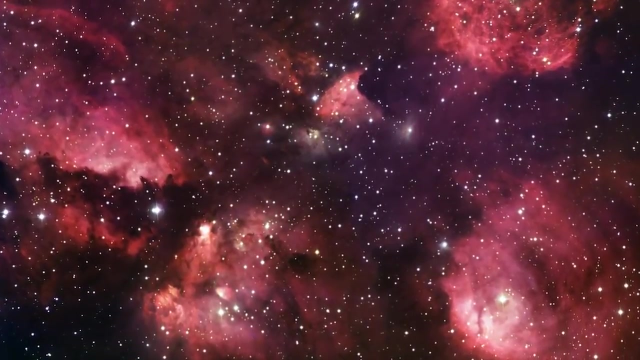 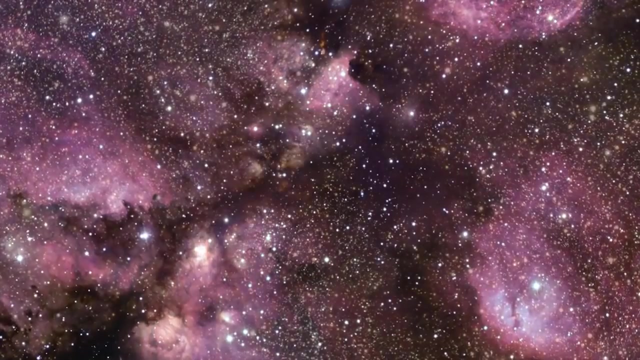 Most of the newborn baby stars are hidden by dust clouds. Again, infrared comes to the rescue, revealing stars in the making. At the end of their lives, stars blow out bubbles of gas, Cosmic showpieces at optical wavelengths. But the infrared picture shows much more detail. 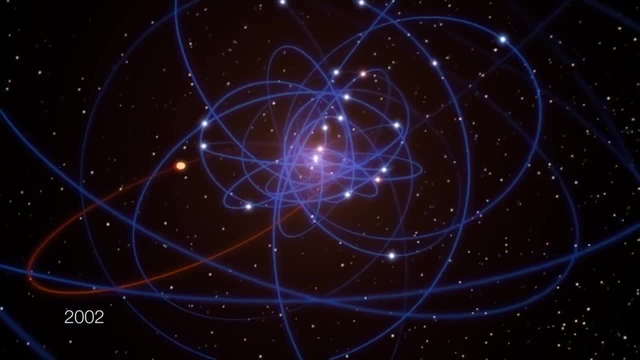 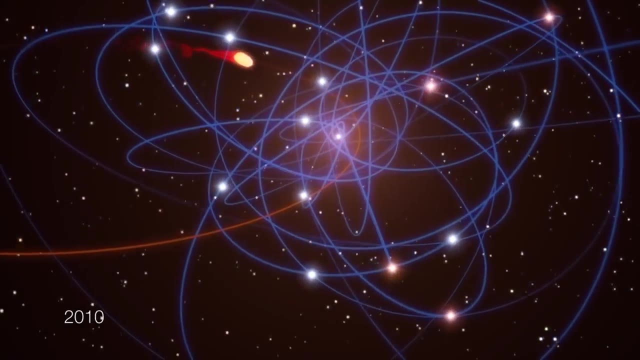 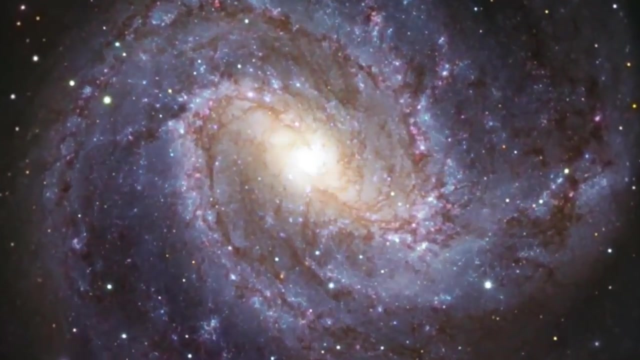 Don't forget the stars and gas clouds captured by the monstrous black hole in the core of our Milky Way galaxy. Without infrared cameras, we would never see them In other galaxies. infrared studies have revealed the true distribution of stars like our own sun. 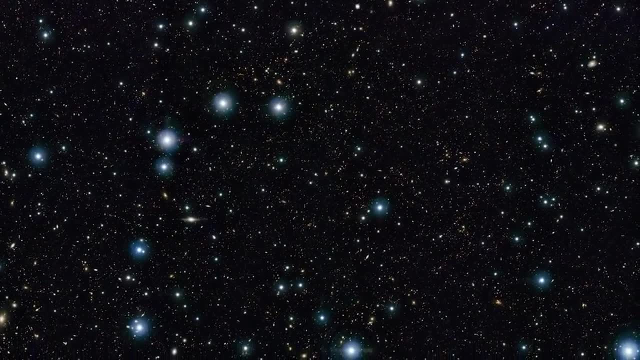 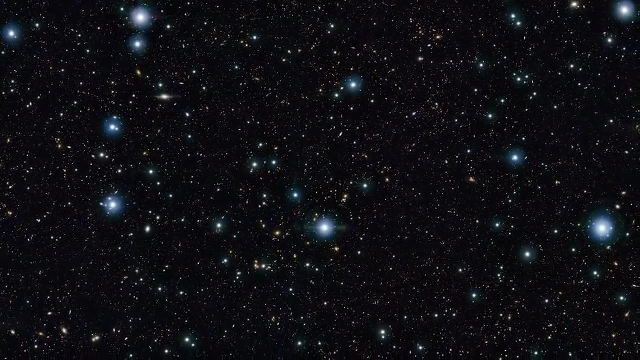 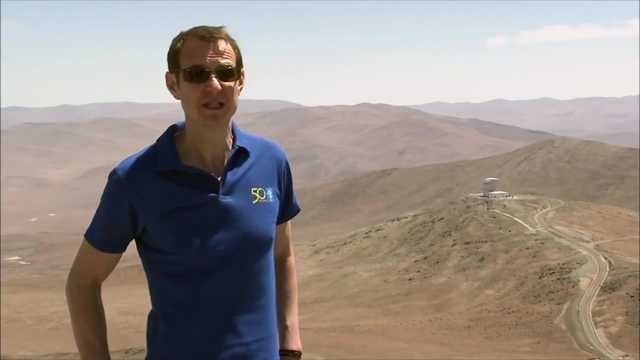 The farthest galaxies are best studied in the infrared. Their light has been shifted to these long wavelengths by the expansion of the universe. Close to Paranal is a small mountain peak with an isolated building on top. Inside this building is the 4.1-metre VISTA telescope. 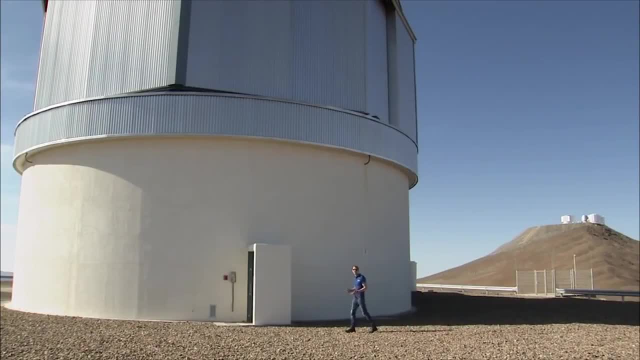 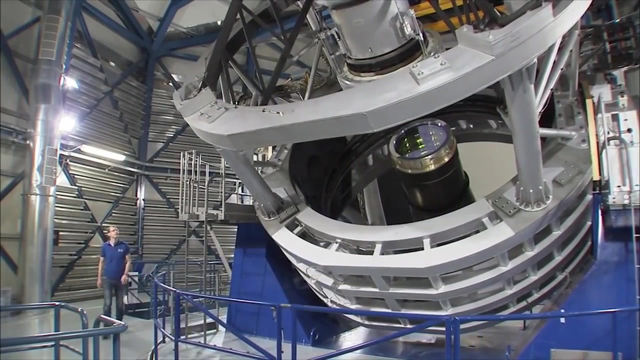 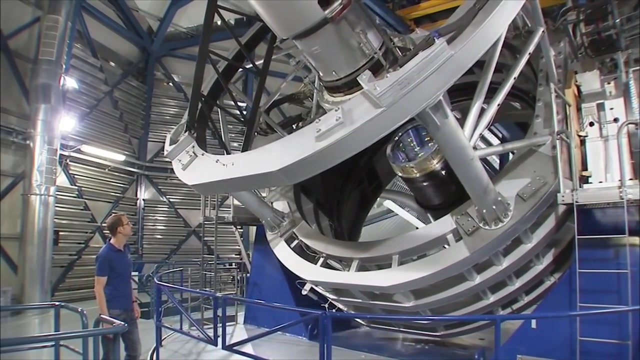 It was built in the United Kingdom, ESO's tenth member state. For now, VISTA only exists. It only does infrared. It uses a giant camera weighing as much as a pickup truck And, yes, VISTA offers unprecedented vistas of the infrared universe. 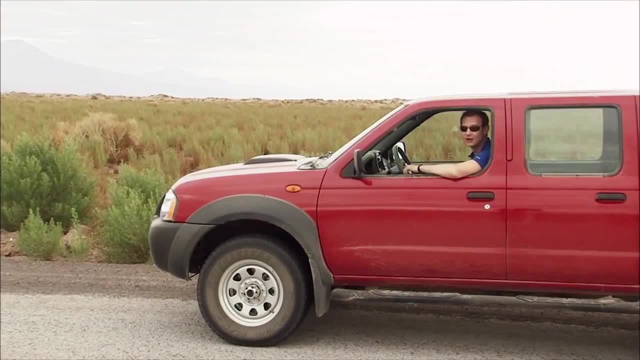 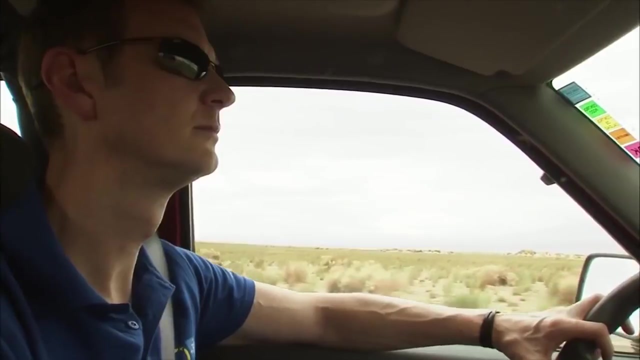 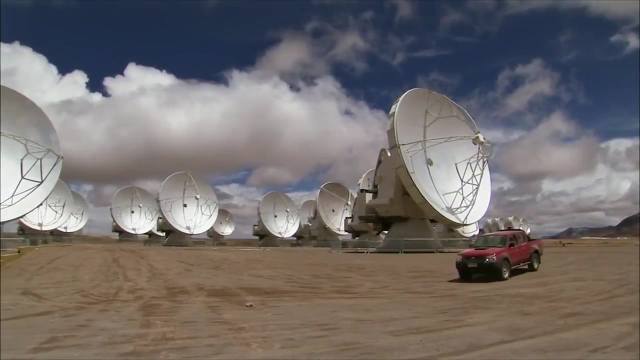 ESO's been doing optical astronomy since its birth 50 years ago And infrared astronomy for about 30 years, But there are more registers to the Cosmic Symphony. 5,000 metres above sea level, high in the Chilean Andes, is the Chajnantor Plateau. 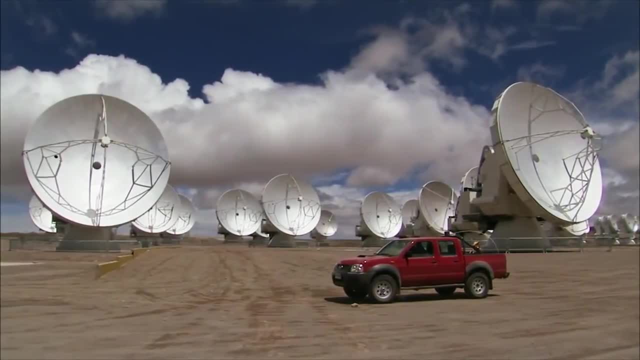 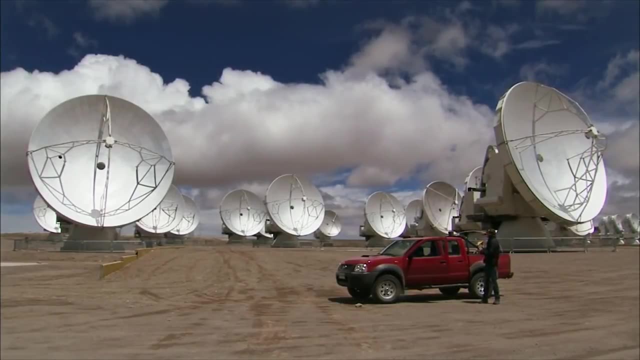 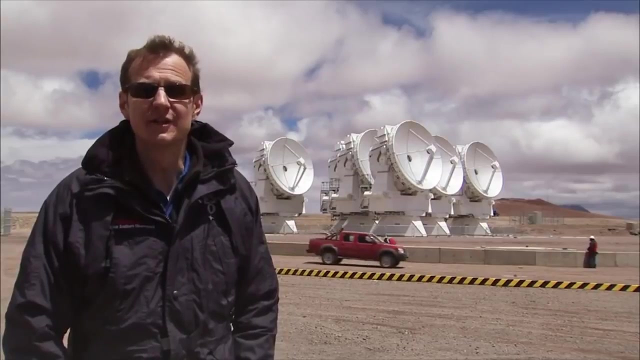 Astronomy doesn't go higher than this. Chajnantor is home to ALMA. The Atacama Large Millimetre Submillimetre Array ALMA is still under construction At a site that is so hostile that it's even hard to breathe. 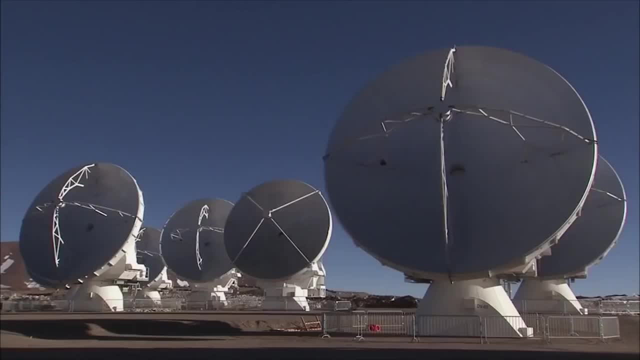 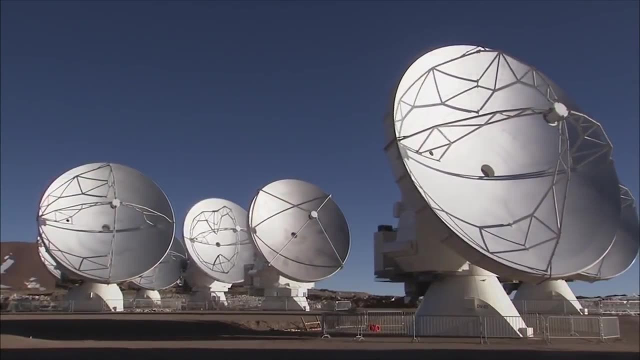 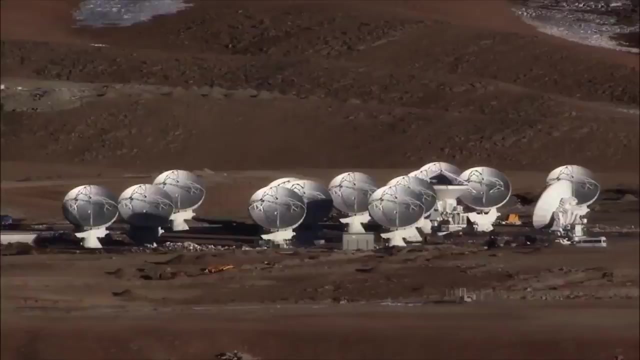 With just 10 of the 66 antennas in place. ALMA made its first observations in the autumn of 2011.. Millimetre waves from space. To observe them, you need to be high and dry. Chajnantor is one of the best places in the world for this. 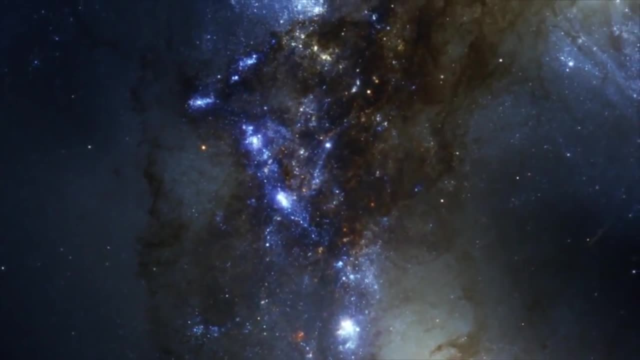 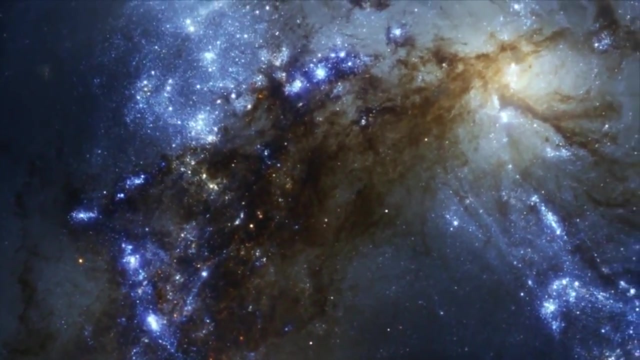 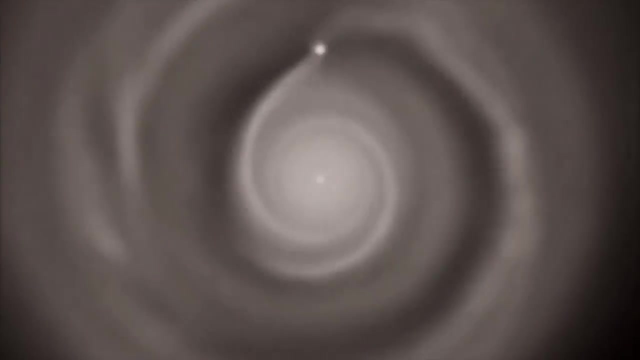 Clouds of cold gas and dark dust become visible in a pair of colliding galaxies. This is not where stars are born, but where they are conceived. And these spiral waves in the outflow of a dying star, could they be due to an orbiting planet? 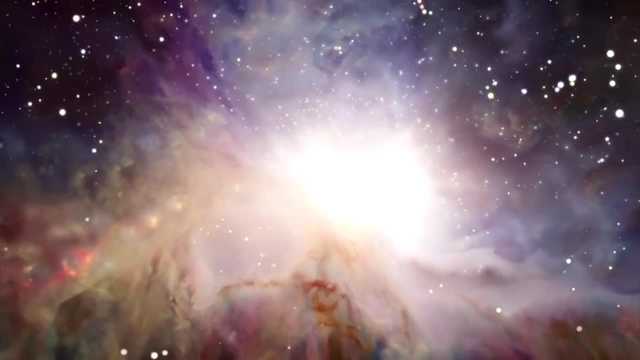 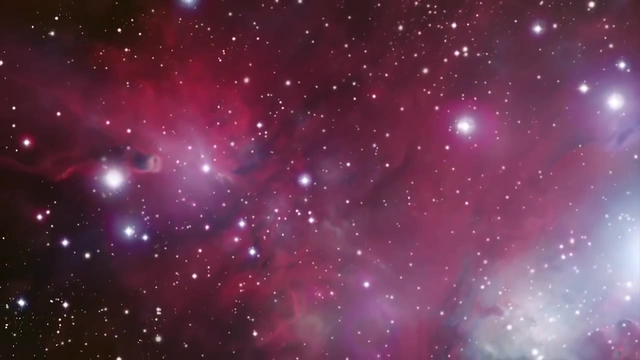 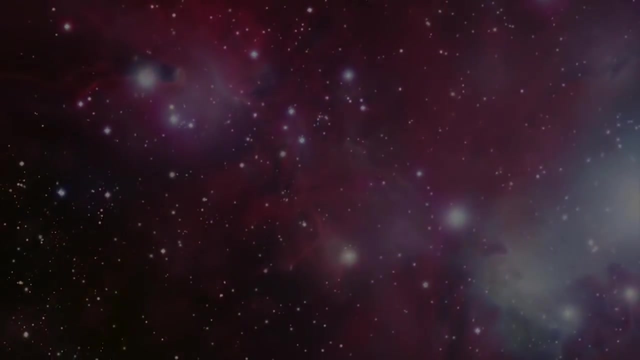 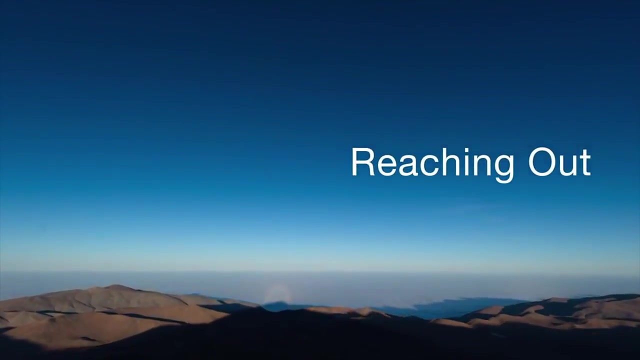 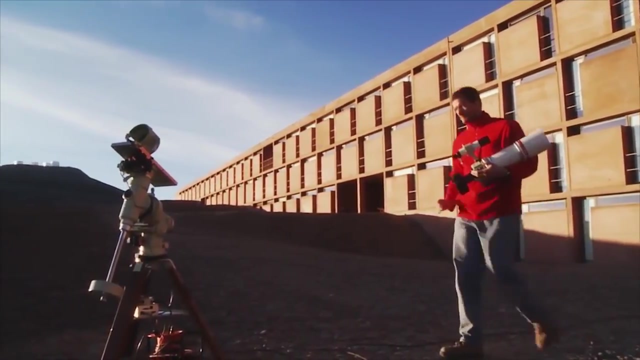 By changing the way we look, we're closing in on the origins of planets, stars and galaxies, On the full symphony of the cosmos, The Atacama, Large, Millimetre, Submillimetre Array. Stéphane Guisard loves the stars. 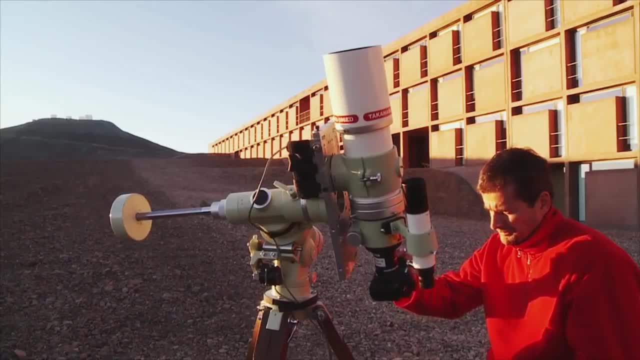 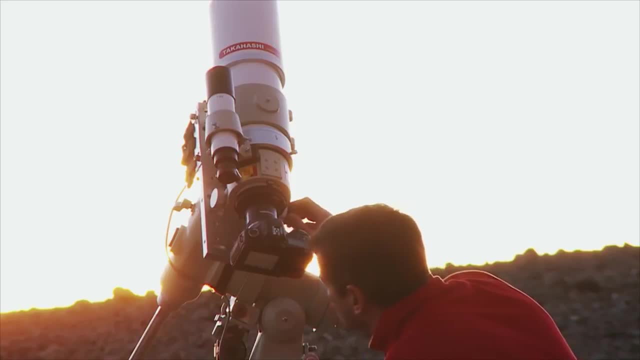 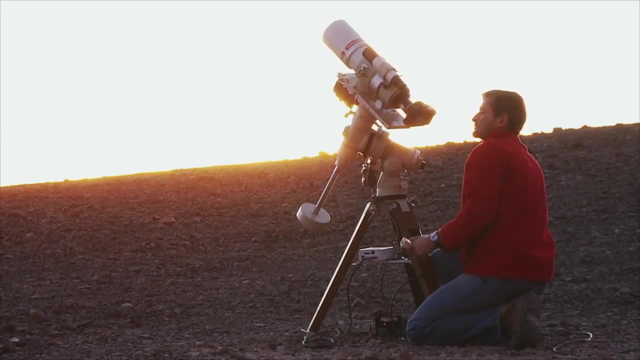 No wonder he loves Northern Chile too. Here, the view of the universe is amongst the best in the world. And no wonder he loves the European Southern Observatory, Europe's eye on the sky. Stéphane is a prize-winning French photographer and author. 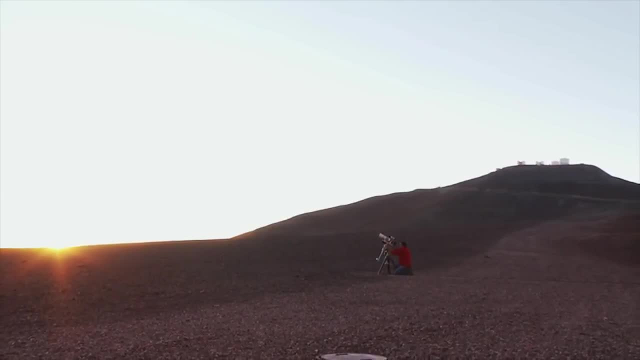 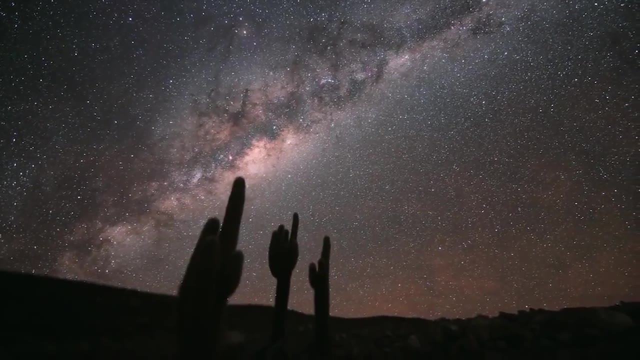 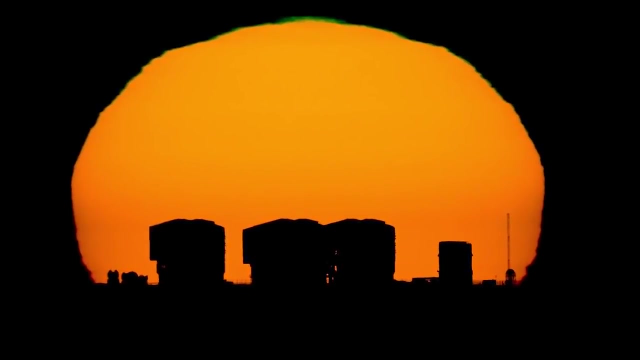 He is also one of ESO's photo ambassadors. In breathtaking pictures, he captures the solitude of the Atacama Desert, the high-tech perfection of giant telescopes and the magnificence of the night sky. He is also one of ESO's photo ambassadors. 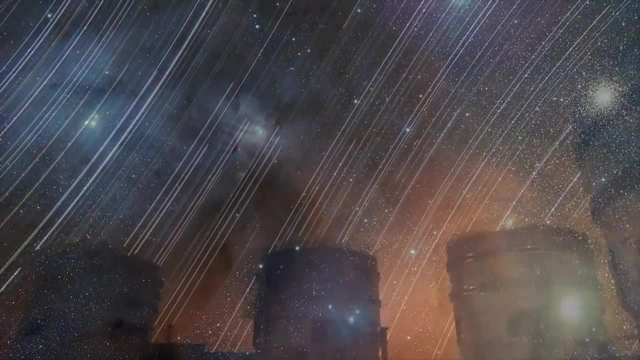 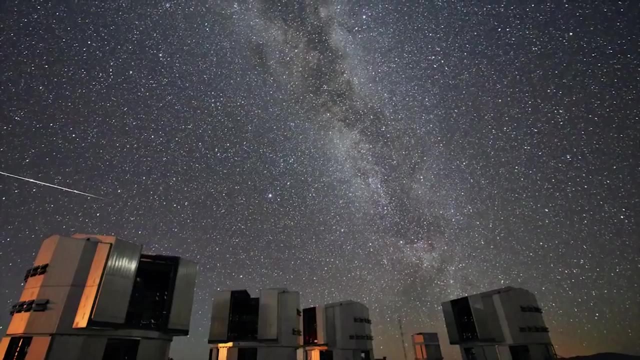 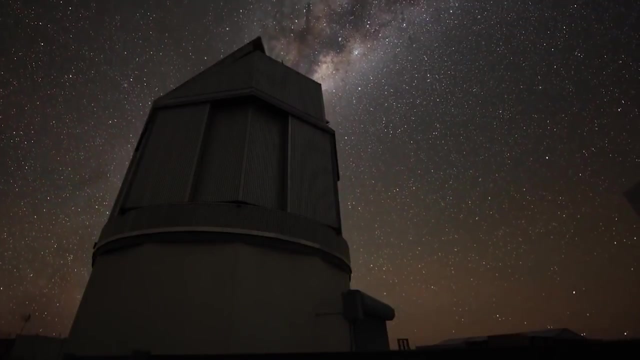 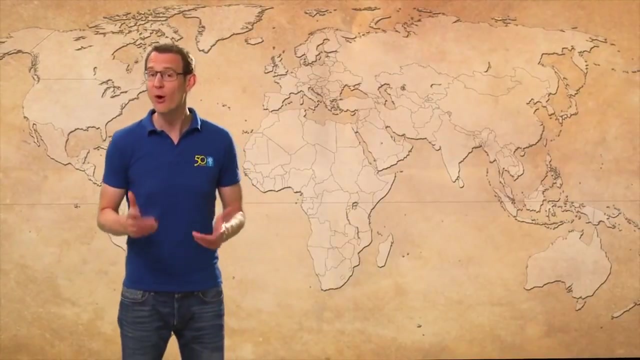 He is also one of ESO's photo ambassadors. Like his fellow photo ambassadors from all over the world, Stéphane helps in spreading ESO's message, A message of curiosity, wonder and inspiration proclaimed through cooperation and outreach. Cooperation has always been the basis of ESO's success. 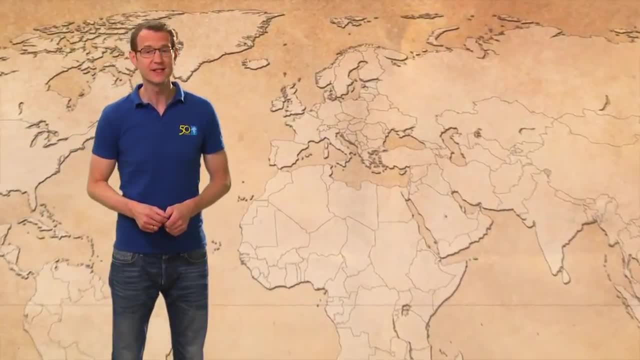 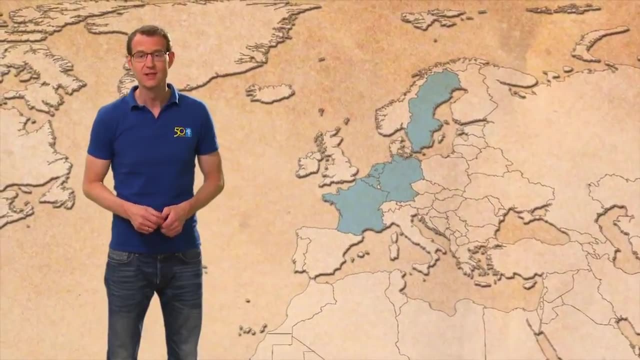 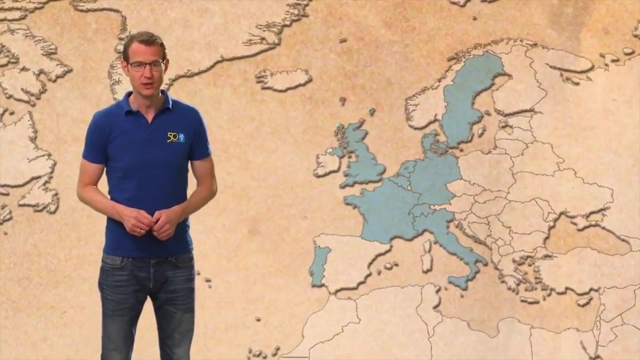 50 years ago, the European Southern Observatory started out with five founding member states: Belgium, France, Germany, the Netherlands and Sweden. Soon other European countries followed: Denmark in 1967, Italy and Switzerland in 1982, Portugal in 2001 and the United Kingdom in 2002.. 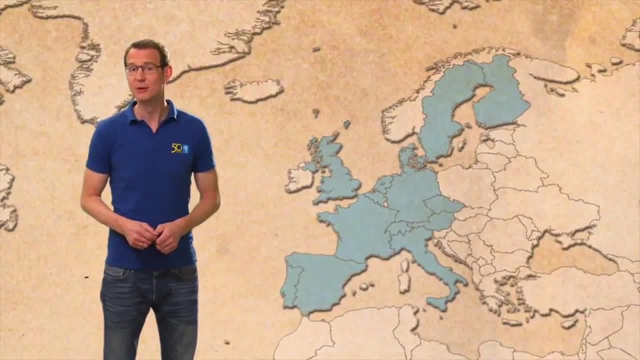 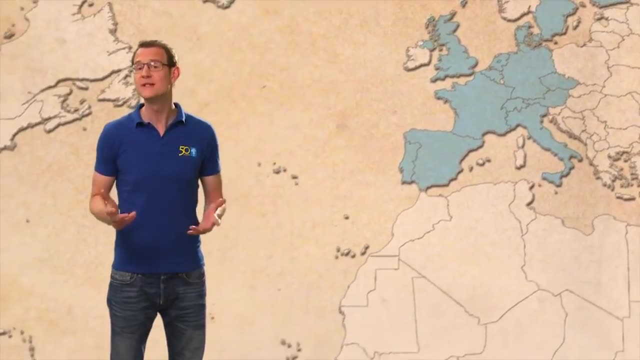 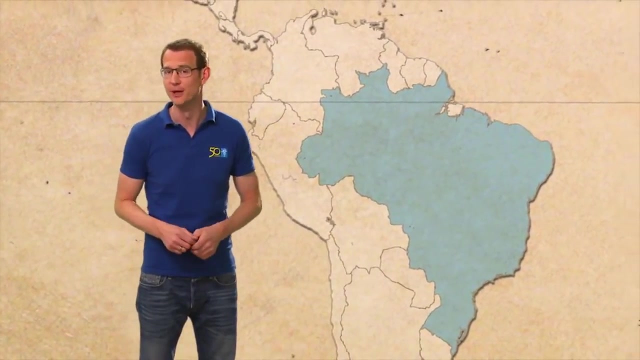 Over the past decade, Finland, Spain, the Czech Republic and Austria also joined Europe's largest astronomy organization. Most recently, Brazil became ESO's 15th member state and the first non-European country to join. Who knows what the future will bring? 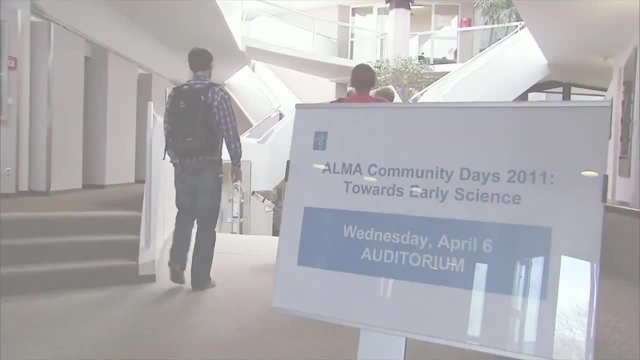 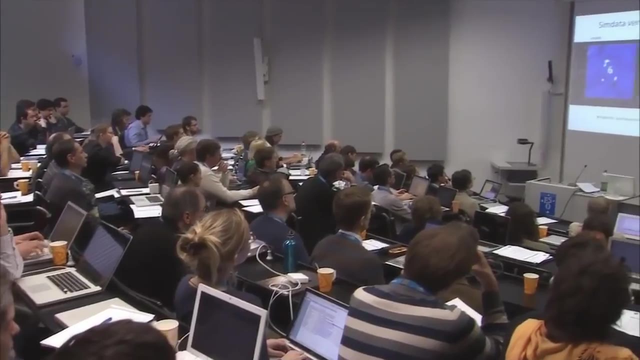 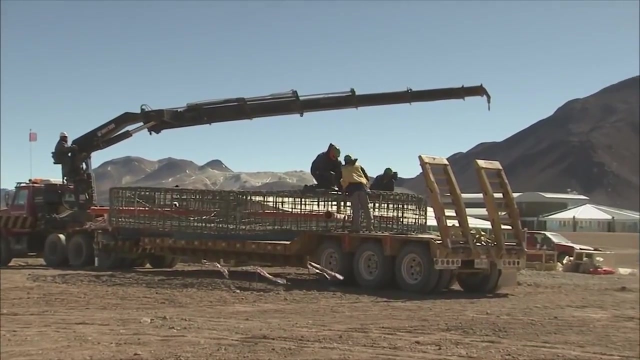 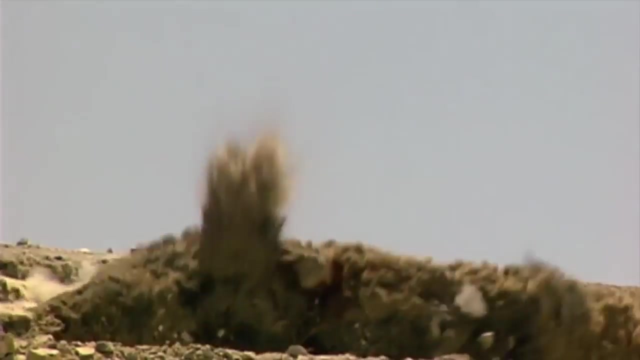 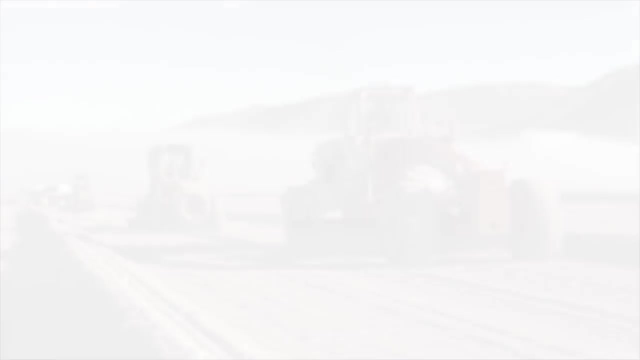 Together, the member states enable the best possible astronomical science at the world's largest observatories. It's good for their economies too. ESO closely cooperates with industry in both Europe and Chile. Access roads had to be constructed, Mountaintops had to be leveled. 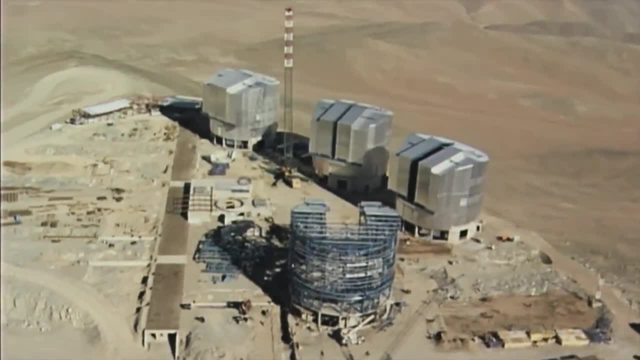 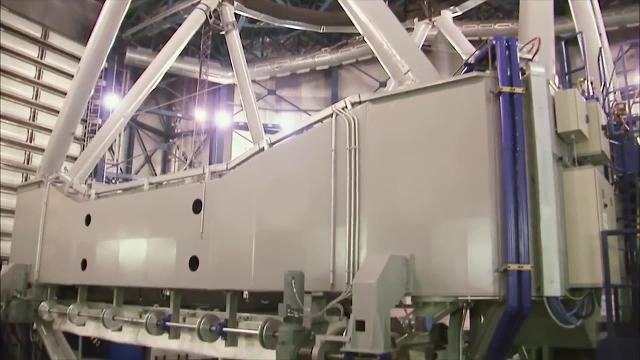 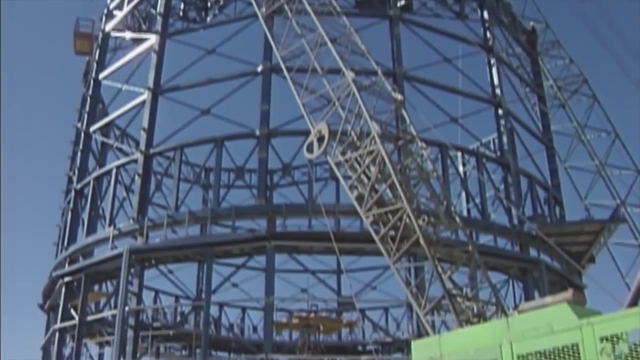 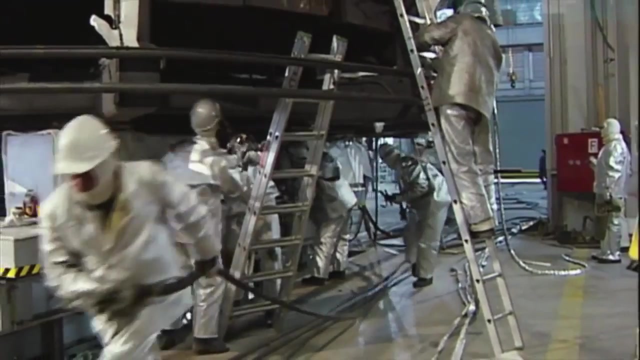 The Italian industrial consortium AES built the main structure of the four VLT telescopes. Each telescope weighs in at some 430 tonnes. They also constructed the giant enclosures, each as high as a 10-storey building. The German glass company Schott produced the delicate VLT mirrors. 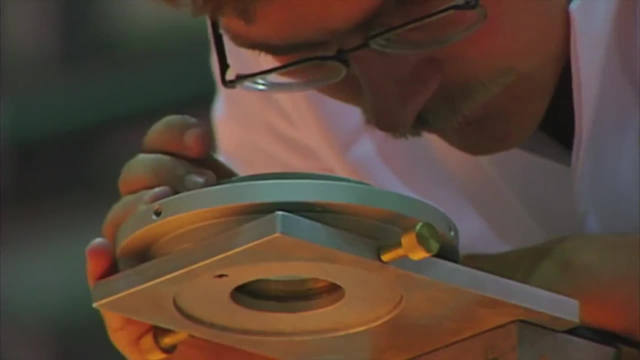 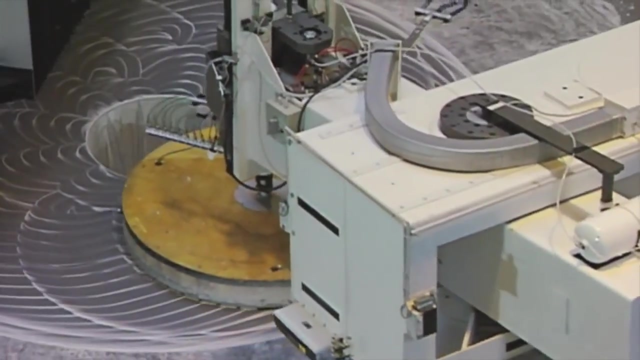 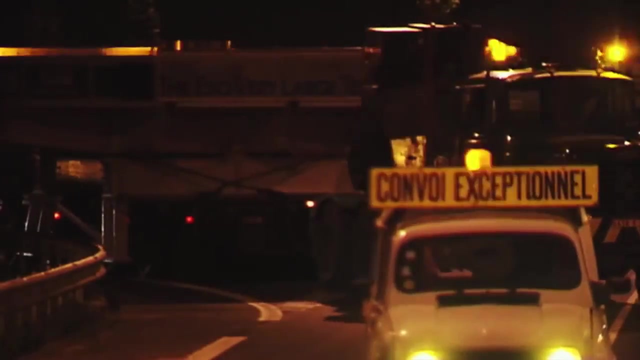 over 8 metres wide and just 20 centimetres thick. At Riosc in France, the telescopes were polished to a precision of a millionth of a millimetre before they made the long journey to Paranal, Meanwhile, universities and research institutes across Europe. 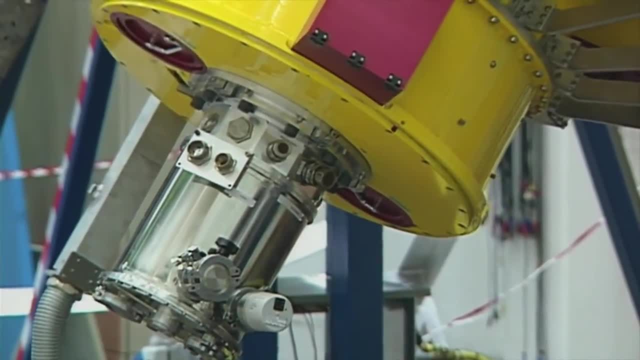 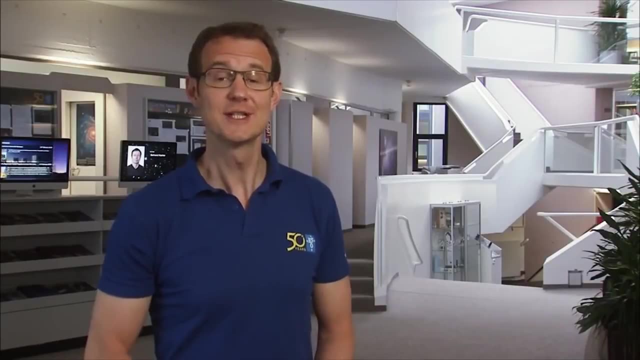 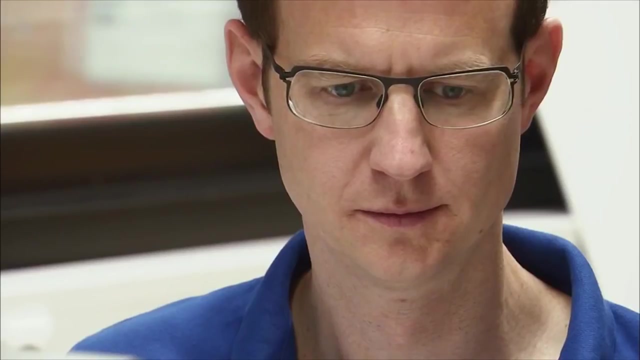 developed sensitive cameras and spectrometers. ESO's telescopes are built with taxpayers' money- your money- and so you can take part in the excitement. For example, ESO's website is a rich source of astronomical information, including thousands of beautiful pictures and videos. 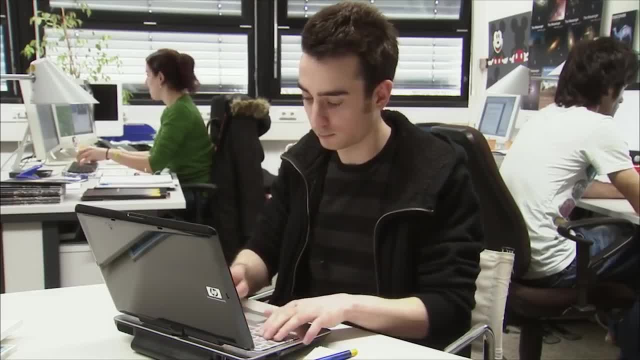 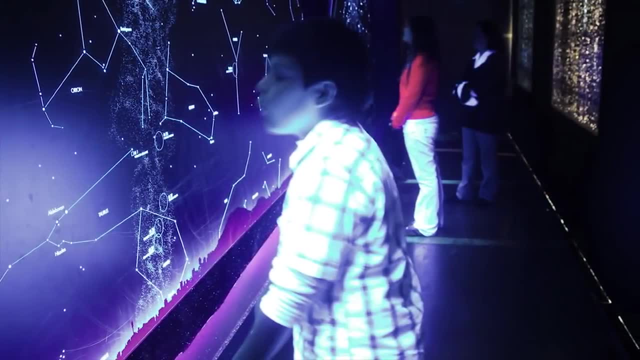 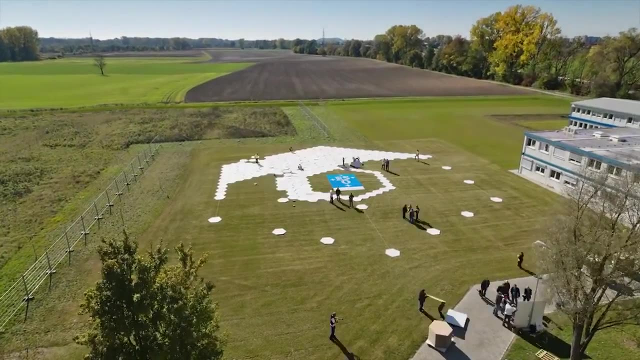 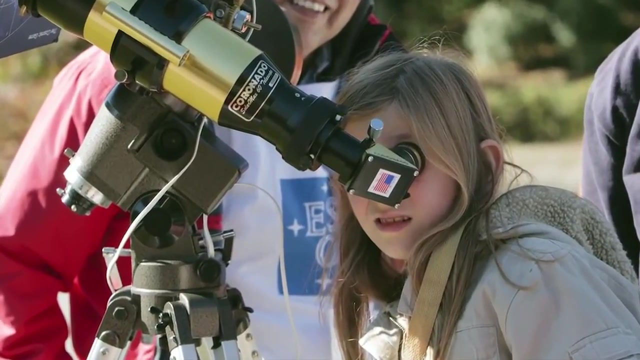 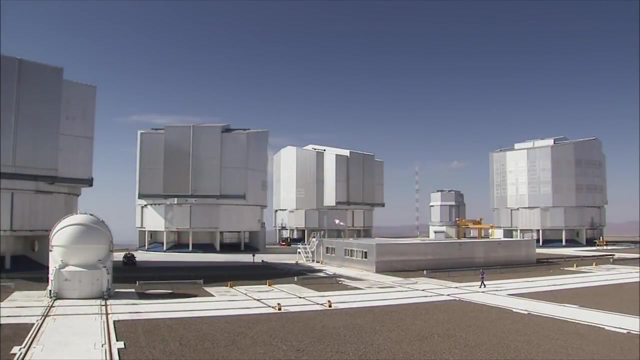 Also, ESO produces magazines, press releases and video documentaries, such as the one you're watching right now. And throughout the world, the European Southern Observatory contributes to exhibitions and science fairs, For example, ESO's, ESO's, ESO's. 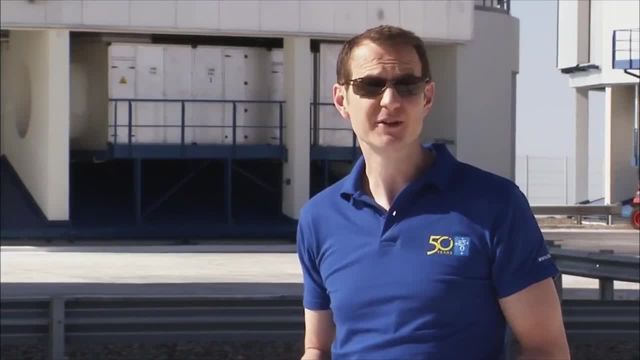 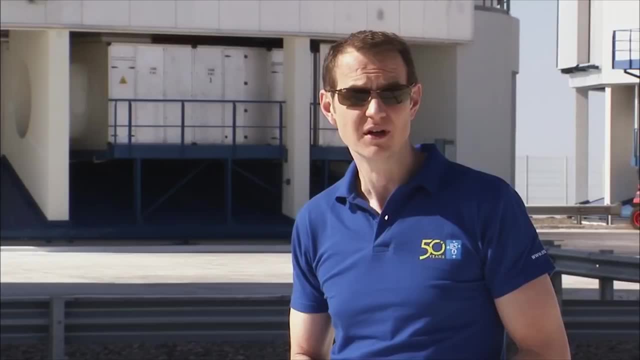 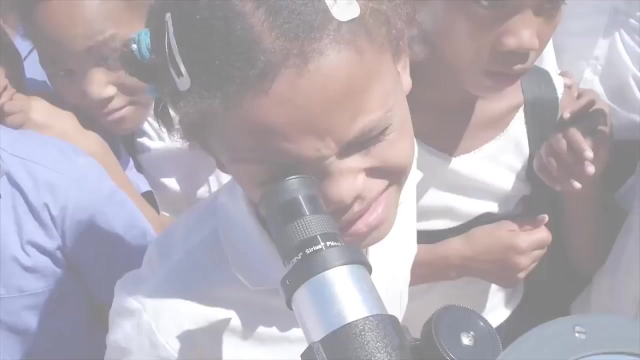 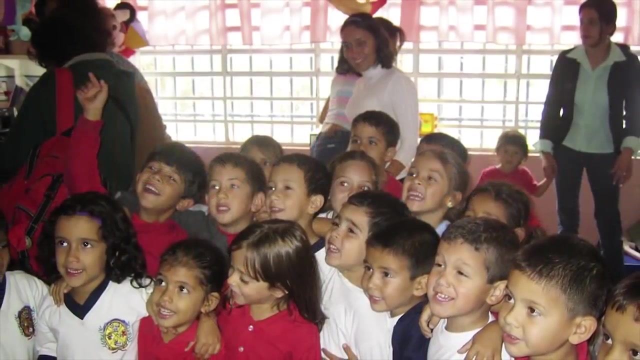 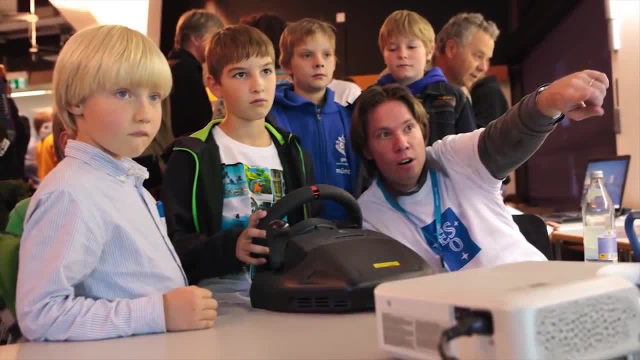 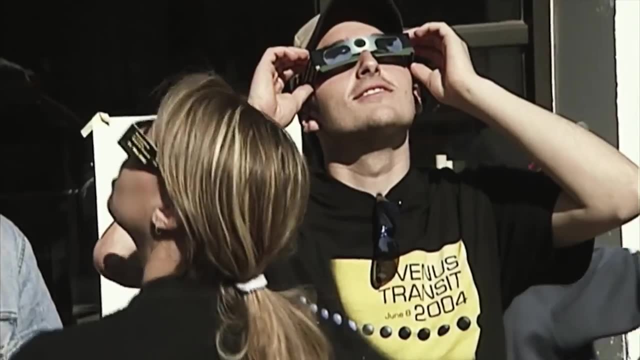 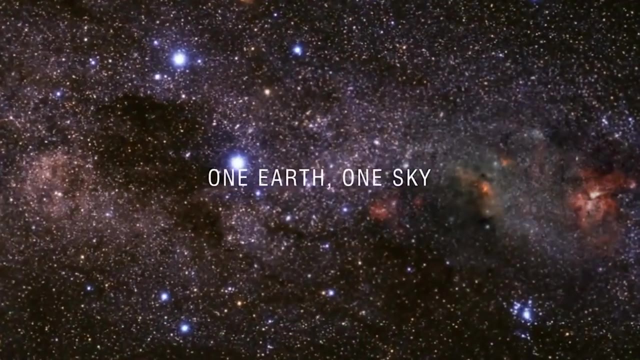 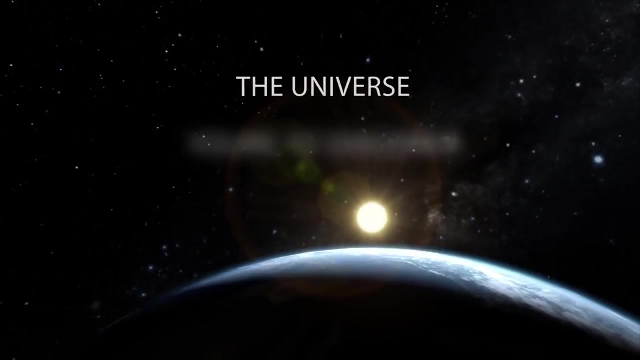 like student exercises and school lectures When the planet Venus passed in front of the Sun. in 2004,, a special programme was aimed at European students and teachers, And in 2009,, during the International Year of Astronomy, ESO reached millions of school children and students all over the world. 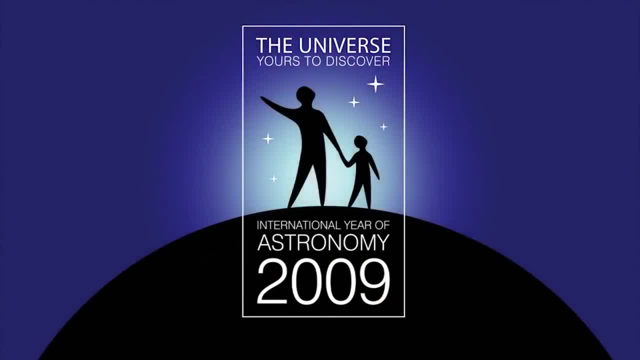 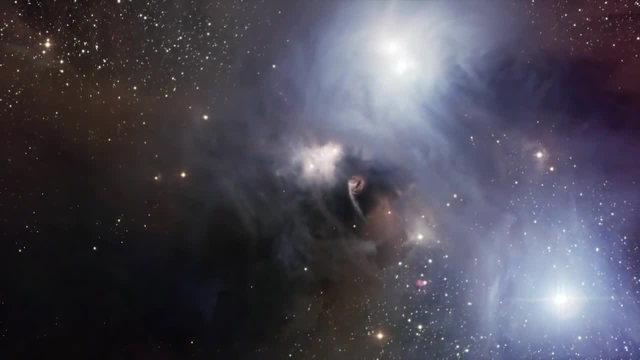 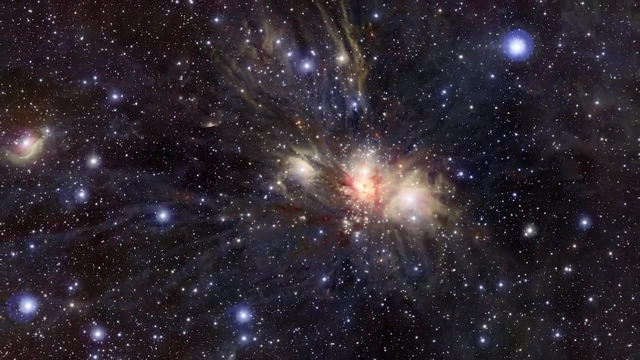 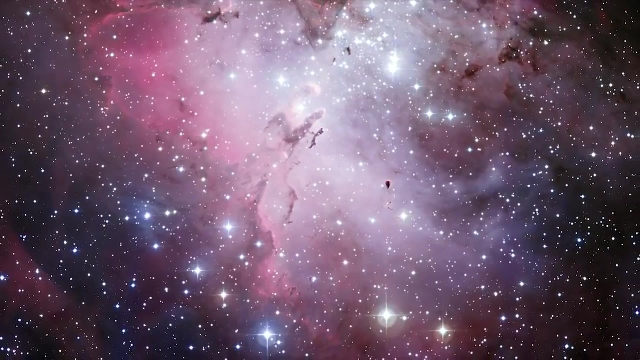 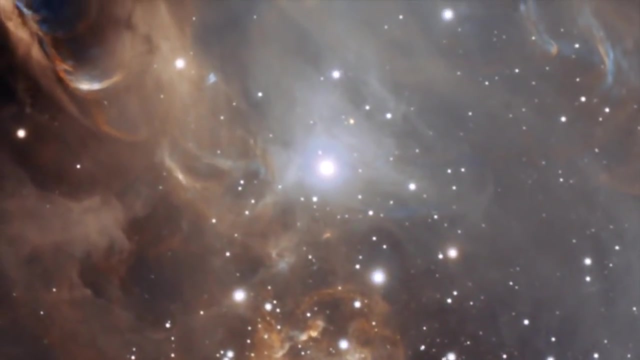 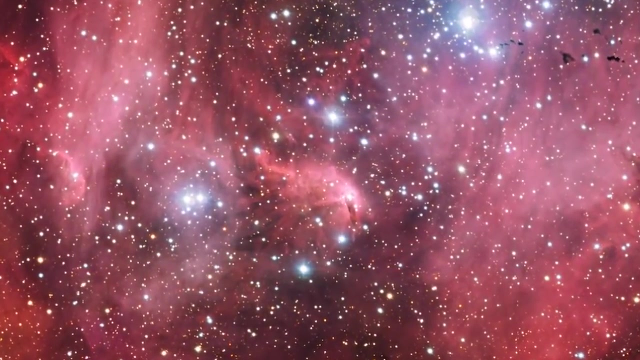 After all, today's children are tomorrow's astronomers. But in terms of outreach, nothing beats the Universe itself. Astronomy is a visual science. Images of galaxies, star clusters and stellar nurseries fire our imagination When not doing science. ESO's telescopes are sometimes used for the Cosmic Gems programme. 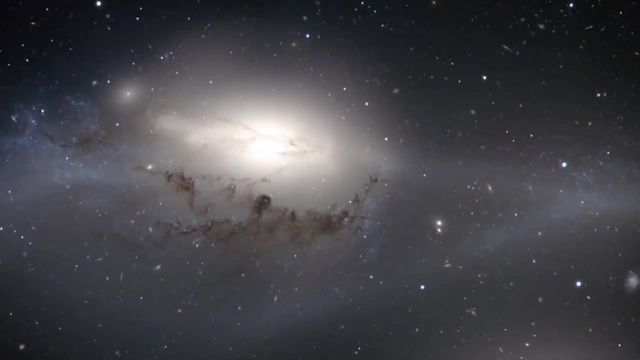 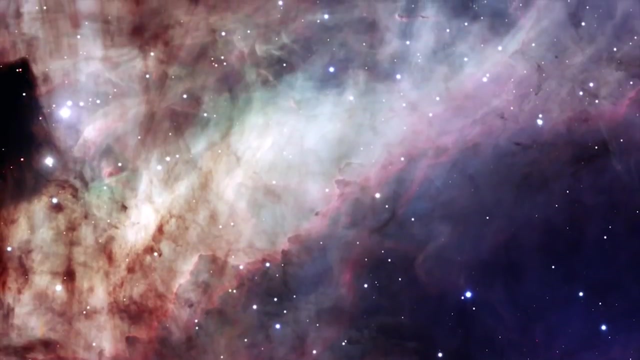 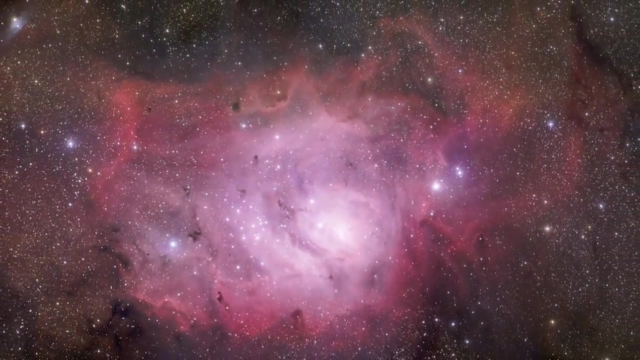 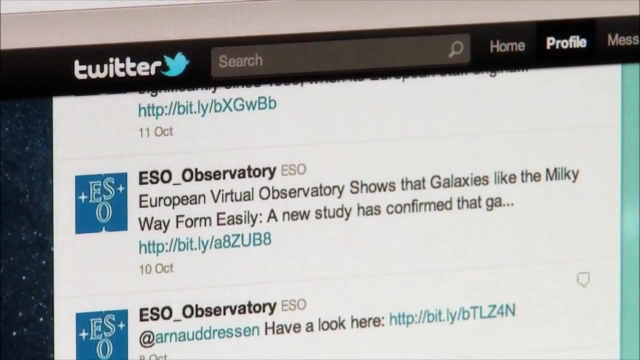 taking pictures just for the purpose of education and public outreach. After all, a picture is worth a thousand words. The general public can even take part in creating these staggering images through the Hidden Treasures competitions. Russian astronomy enthusiast Igor Chkalin won the competition in 2010.. 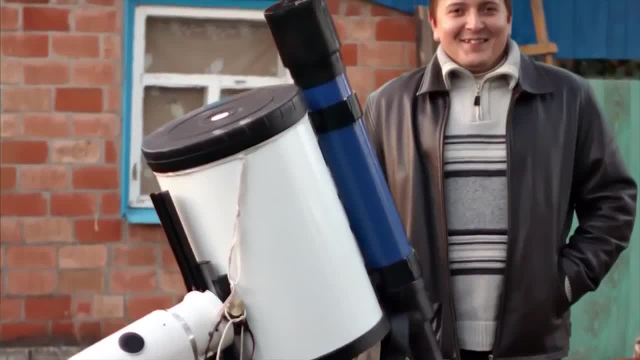 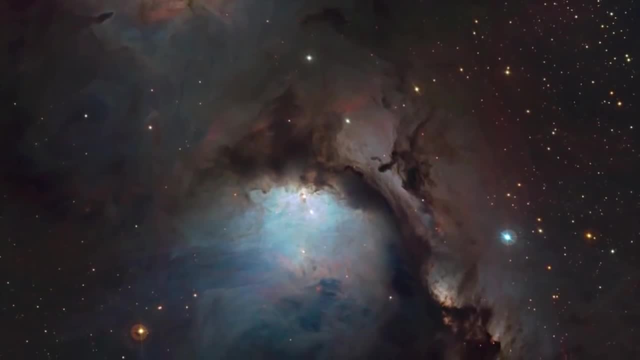 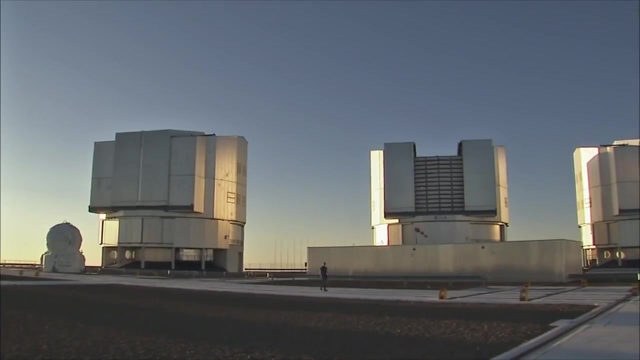 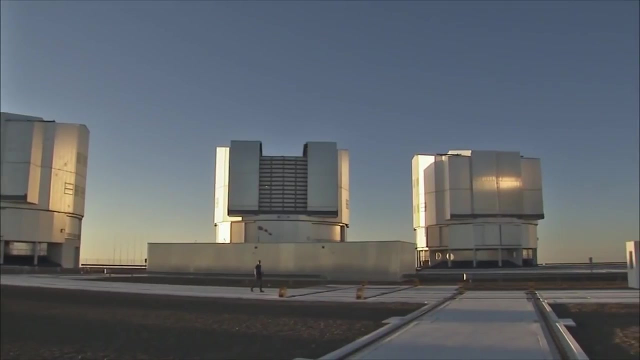 He was the first Russian astronomer to win the competition. His marvellous images are based on real science data, Member states, industry and universities. By cooperating on all possible levels, ESO has become one of the most successful astronomy organisations in the world. 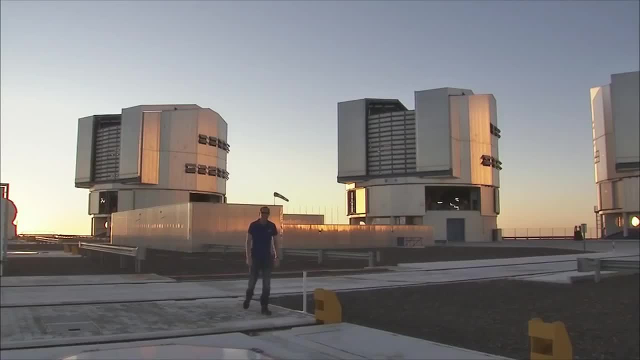 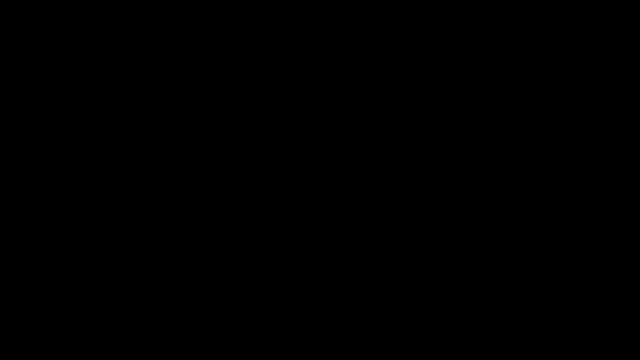 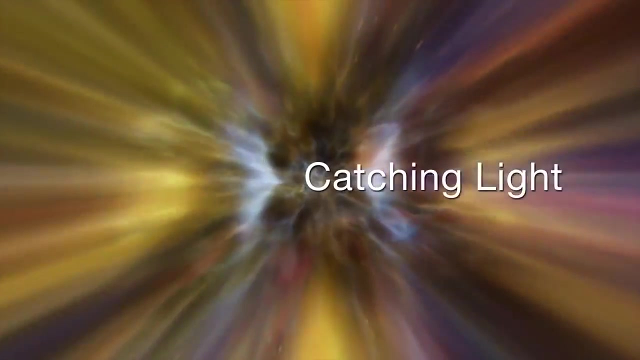 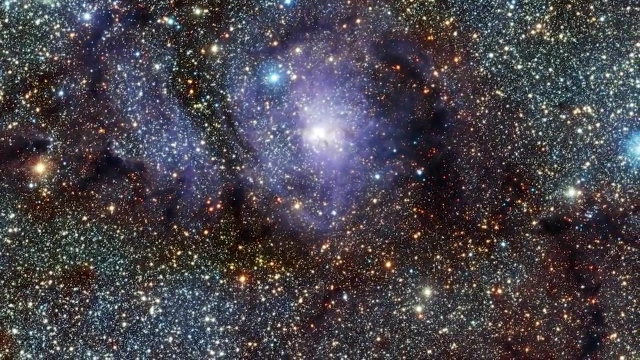 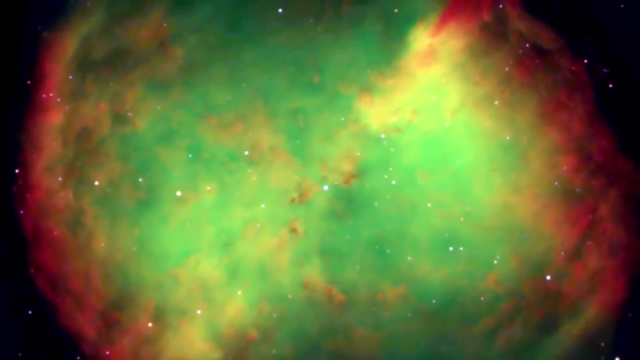 And through its engagement with the public, you are invited to join the adventure. ESO- the European Space Agency. The Universe is yours to discover. For half a century, the European Southern Observatory has showcased the splendour of the Universe: ESO- the European Space Agency. 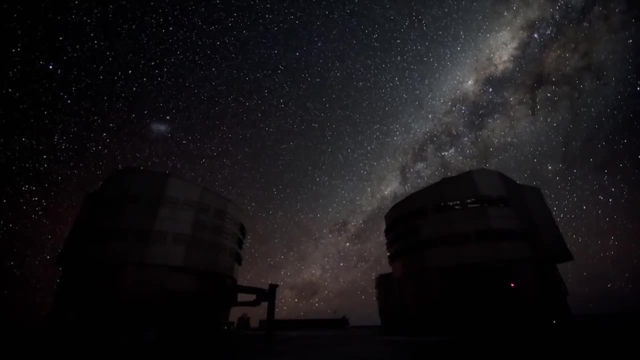 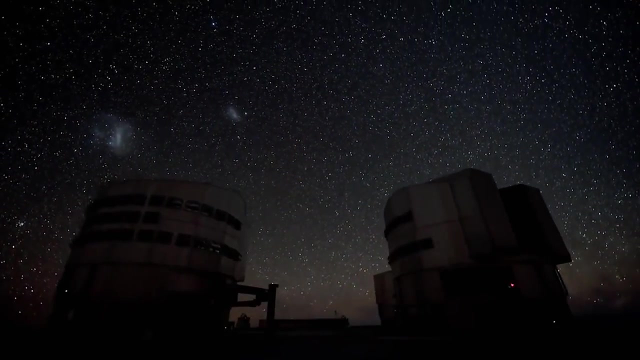 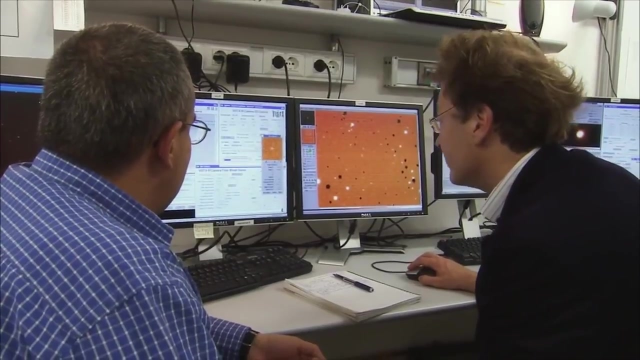 Starlight rains down on the Earth. Giant telescopes catch the cosmic photons and feed them to state-of-the-art cameras and spectrographs. Today's astronomical images are very different from those of the 1960s, When ESO began back in 1962,. 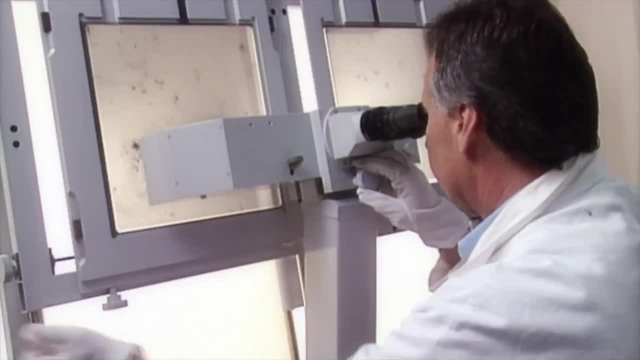 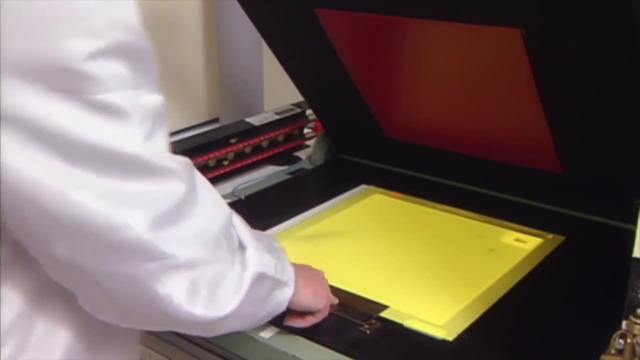 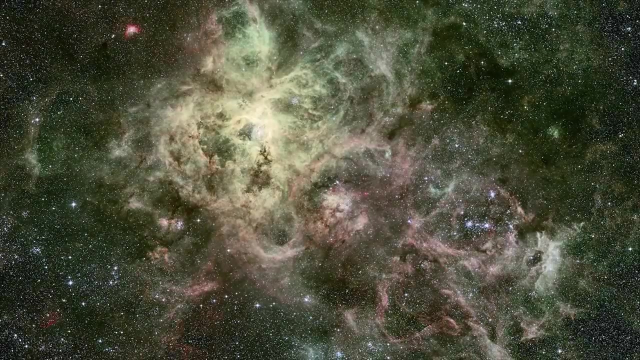 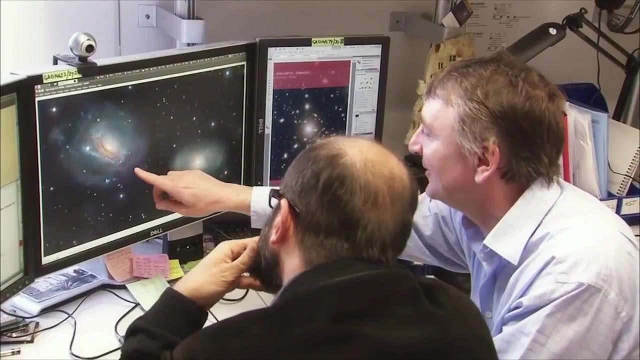 astronomers used large photographic glass plates, Not very sensitive, imprecise and hard to handle. What a difference today's electronic detectors have made. They catch almost every photon, The images are available instantaneously and, most importantly, they can be processed and analysed by computer software. 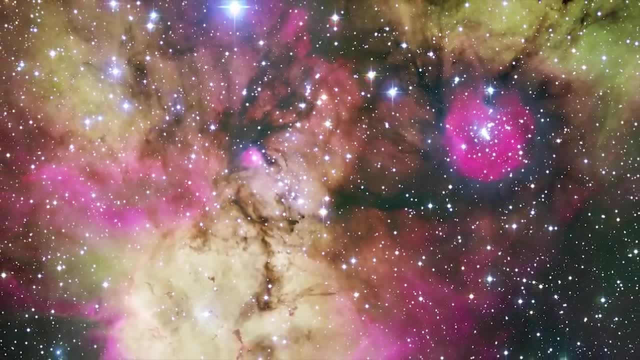 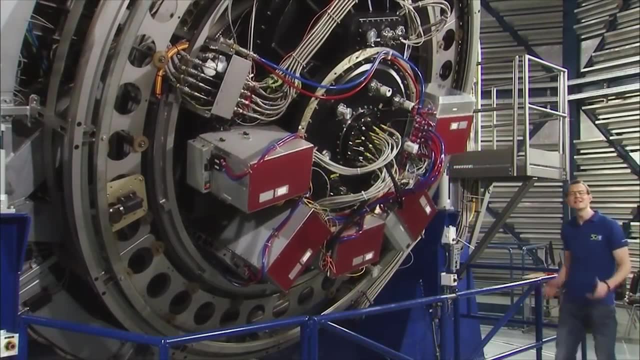 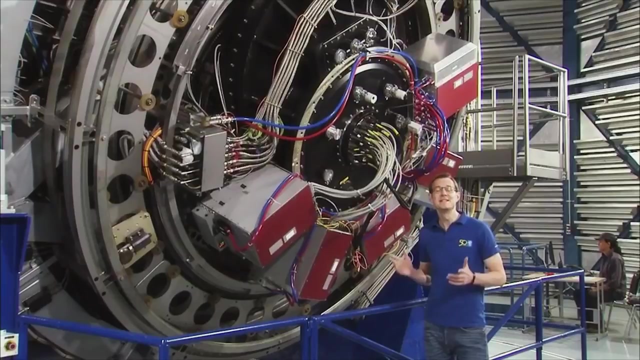 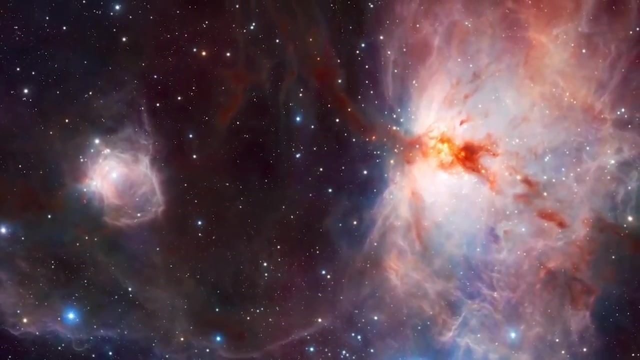 Astronomy has truly become a digital science. ESO telescopes use some of the largest and most sensitive detectors in the world. The Vista camera has no less than 16 of them, for a total of 67 million pixels. This huge instrument catches infrared light. 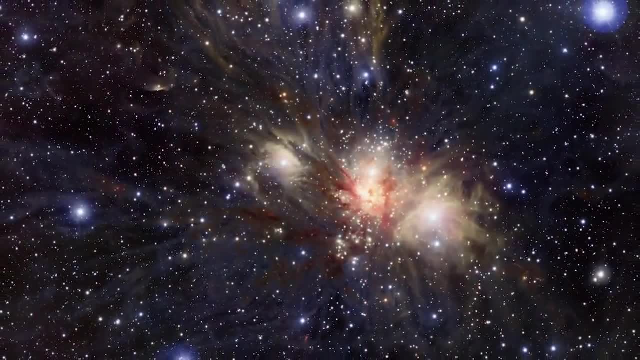 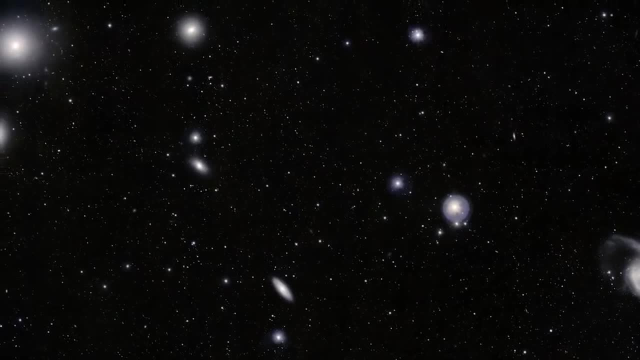 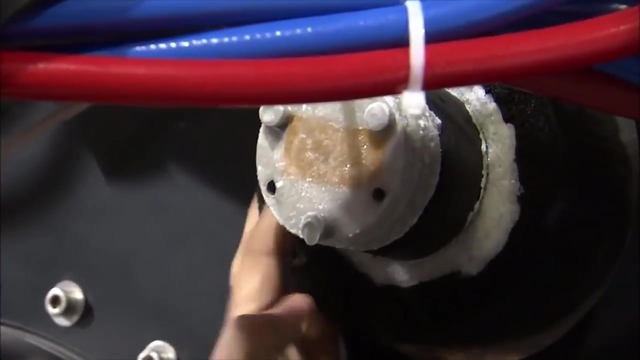 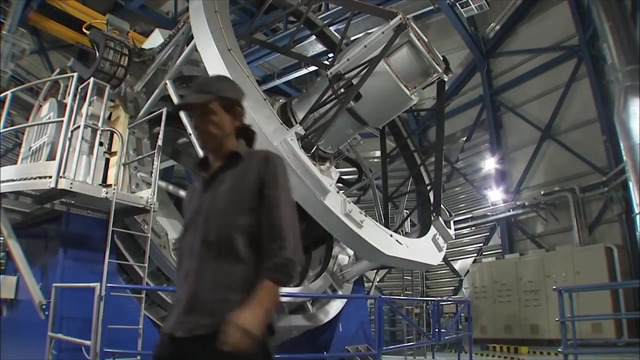 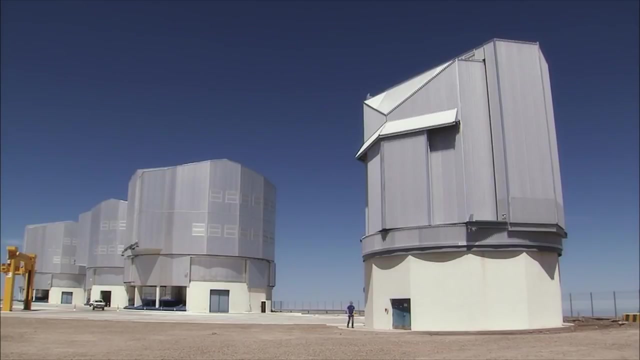 from cosmic dust clouds, newborn stars and distant galaxies. Liquid helium keeps the detectors at minus 269 degrees. Vista takes an inventory of the southern sky like an explorer surveying an unknown continent. The VLT survey telescope is another discovery machine, but this one works at visible wavelengths. 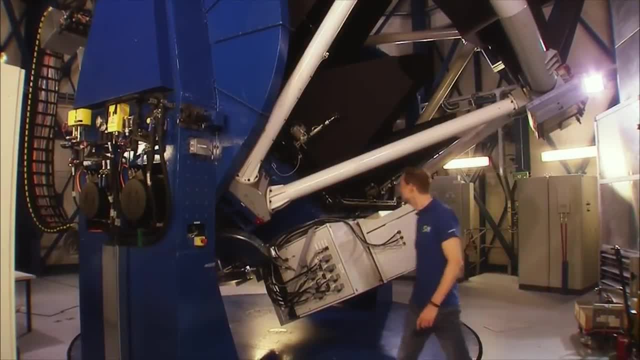 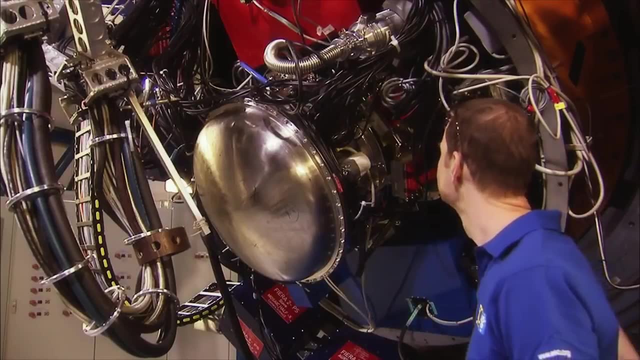 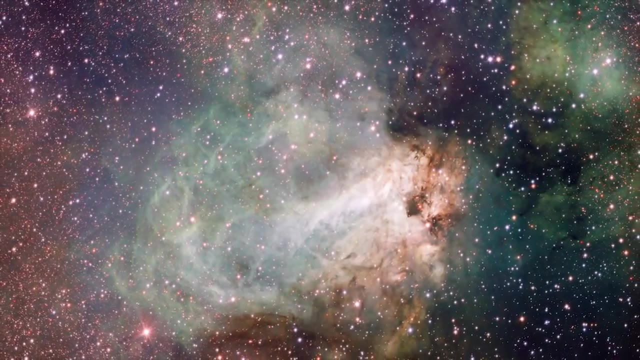 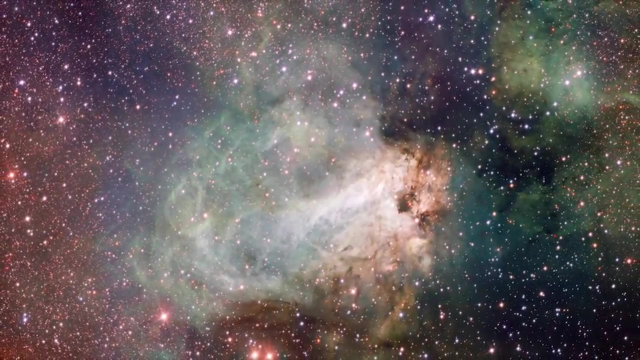 Its camera, called OmegaCam, is even larger: 32 CCDs team up to produce spectacular images with a mind-boggling 268 million pixels. The field of view is one square degree, four times as large as the full moon. OmegaCam generates 50 gigabytes of data every night. 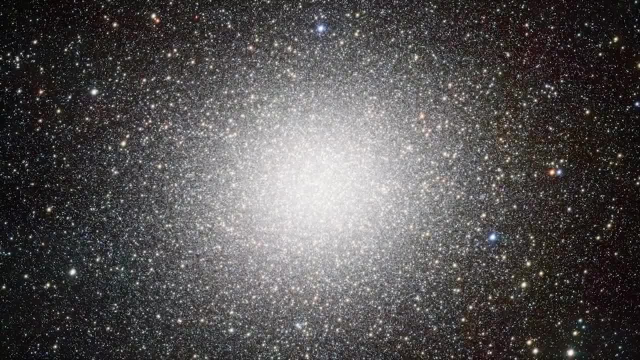 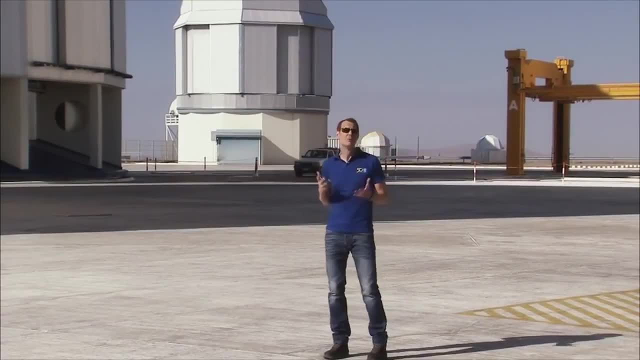 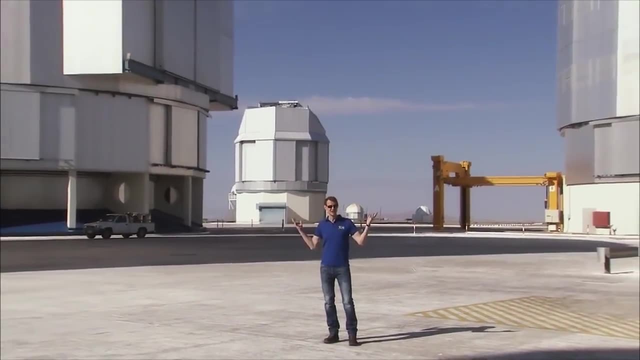 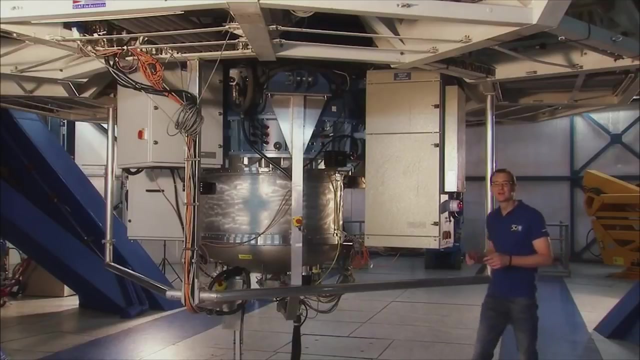 And these are just gorgeous. gigabytes Survey telescopes like Vista and the VST also mine the sky for rare and interesting objects. Astronomers then use the sheer power of the VLT to study these objects in exquisite detail. Each of the VLT's four telescopes has its own set of unique instruments. 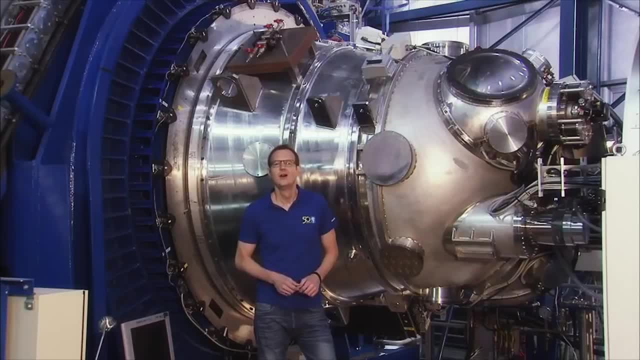 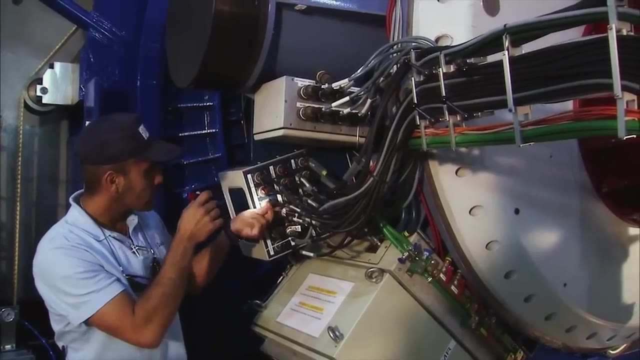 each with its own particular strengths. Without these instruments, ESO's giant eye on the sky would be well blind. They have fanciful names like Isaac Flames, Hawkeye and Symphony Giant high-tech machines, each the size of a small car. 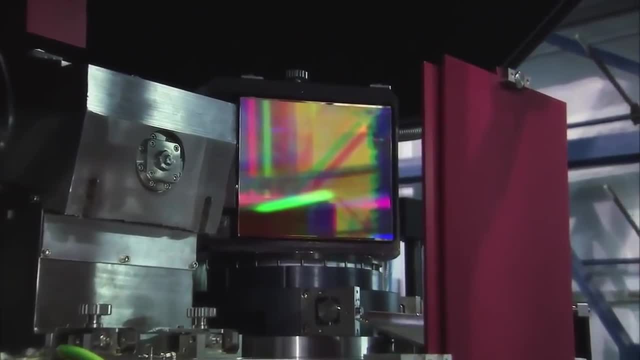 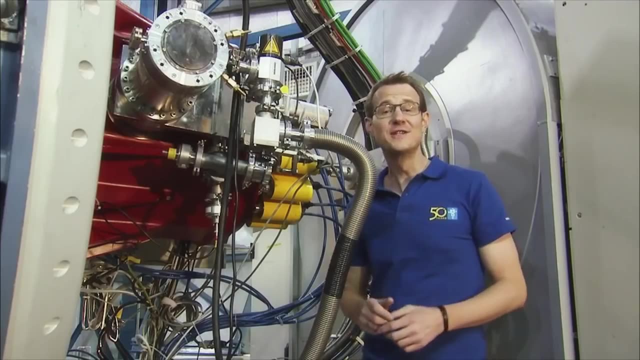 Their purpose: To record the cosmic photons and recover every possible bit of information. All of the instruments are unique, but some are a little more special than others. For example, NACO here and Symphony use the VLT's adaptive optics system. 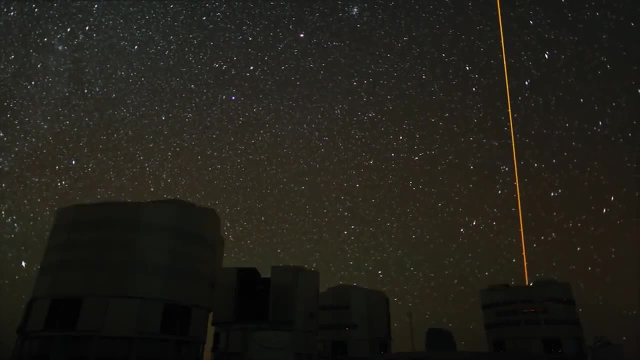 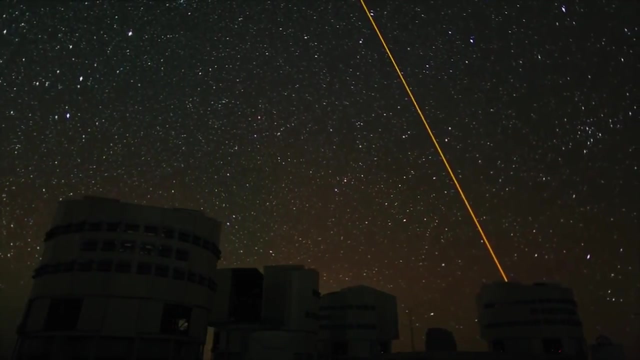 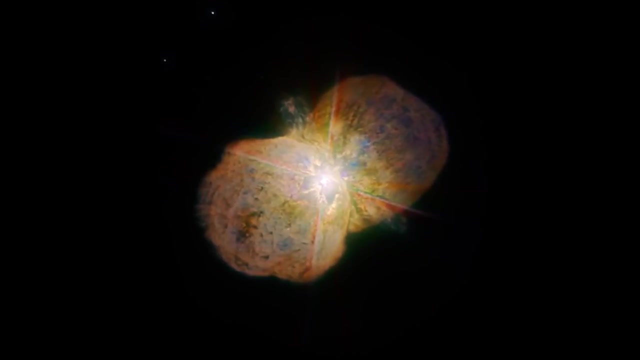 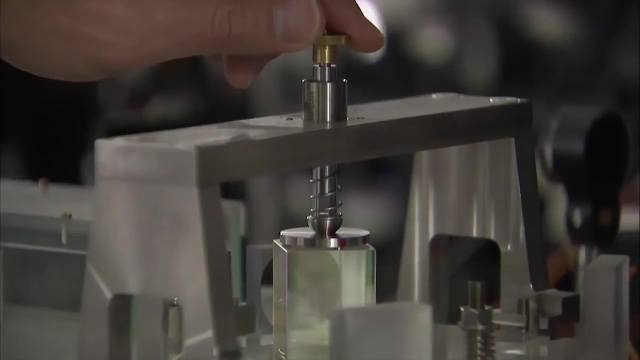 Lasers produce artificial stars that help astronomers to correct for atmospheric blurring. NACO's images are as sharp as if they were taken from outer space. And then there's MIDI and AMBER, two interferometric instruments. Here light waves from two or more telescopes. 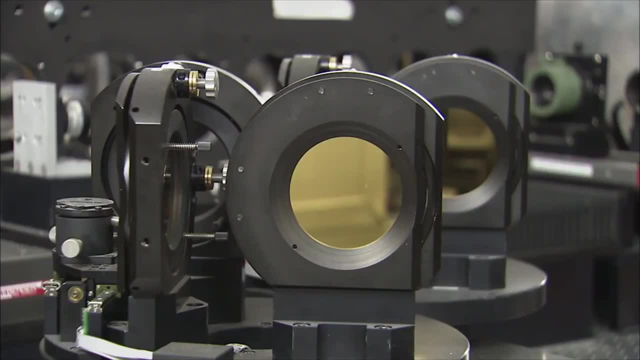 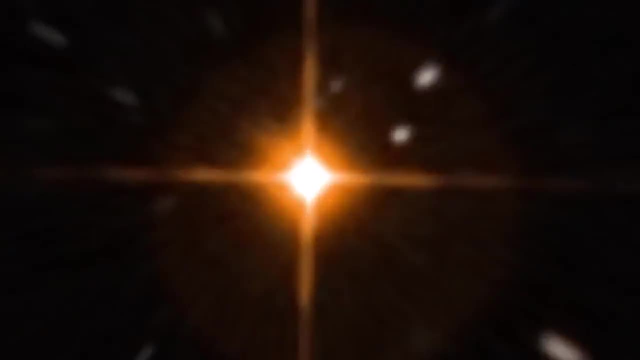 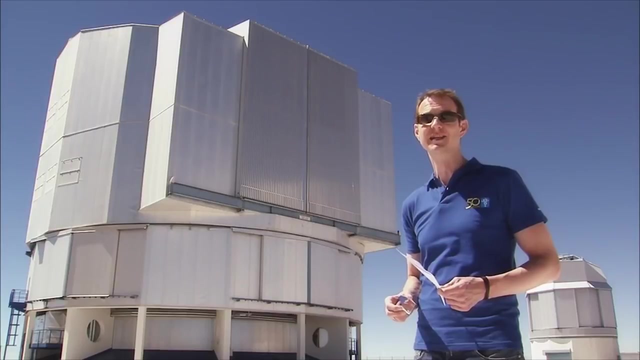 are brought together as if they were captured by one giant single mirror. The result: The sharpest views you can imagine. But astronomy is not only about taking images. If you're after the details, you have to dissect the starlight and study its composition. 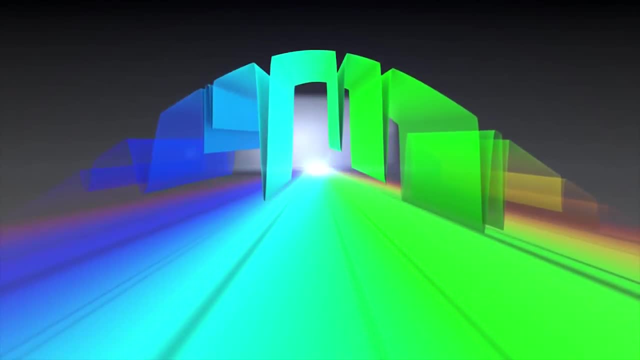 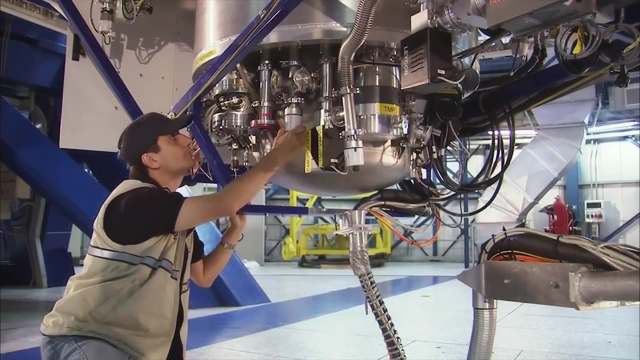 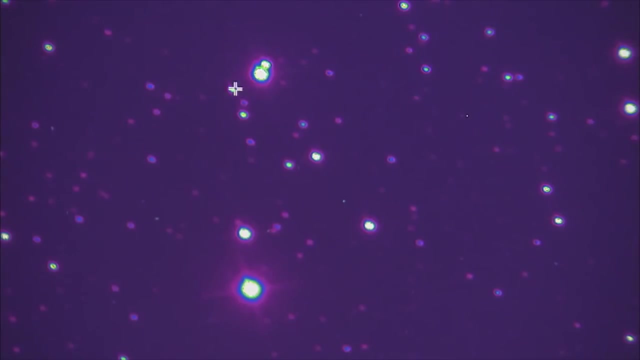 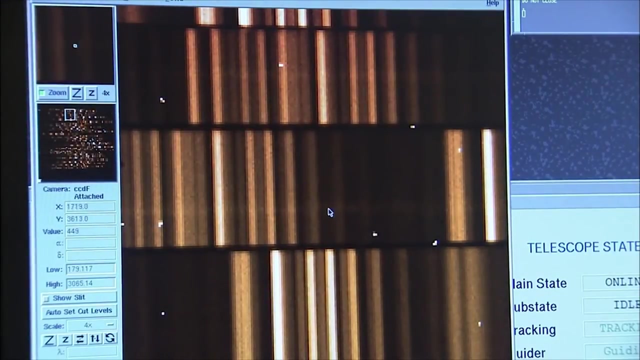 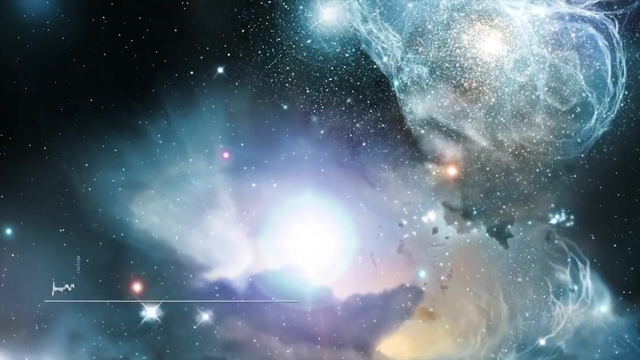 Spectroscopy is one of astronomers' most powerful tools. No wonder ESO boosts some of the world's most advanced spectrographs, like the powerful X-shooter. Images carry more beauty, but spectra reveal more information. Composition, Motions, Ages. 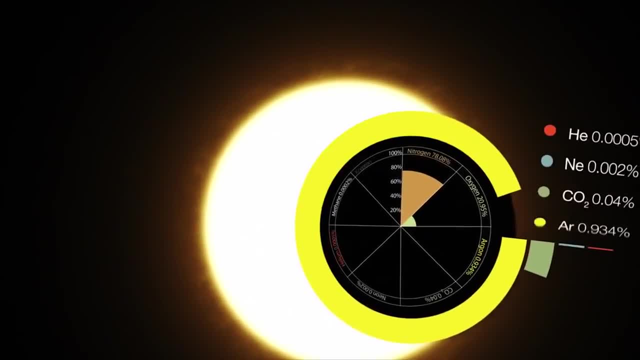 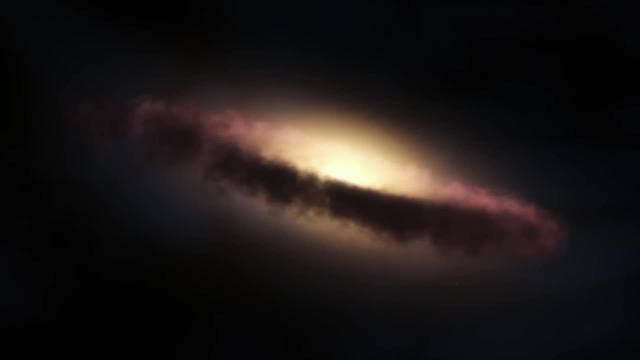 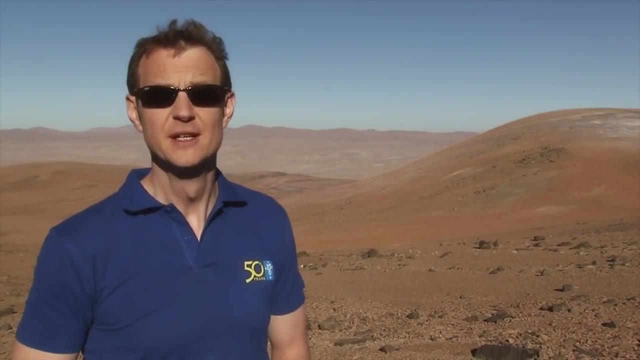 The atmospheres of exoplanets, orbiting distant stars Or newborn galaxies at the edge of the observable universe. Without spectroscopy, we would just be explorers staring at a beautiful landscape. With spectroscopy, we learn about the landscape's topography. 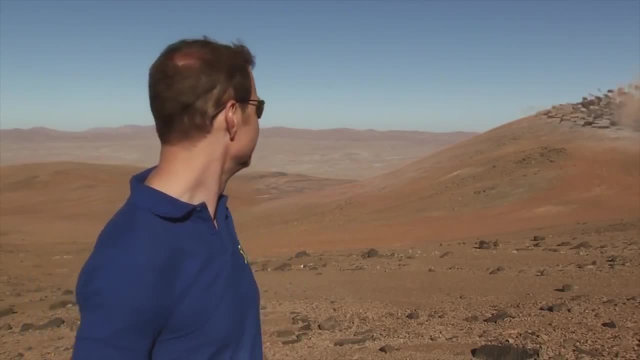 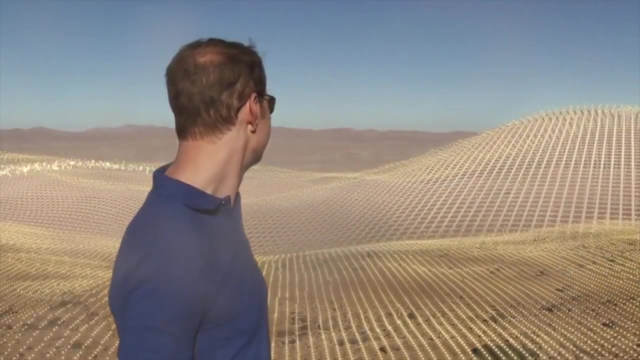 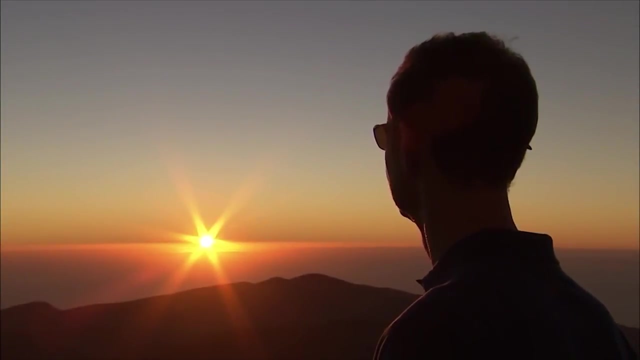 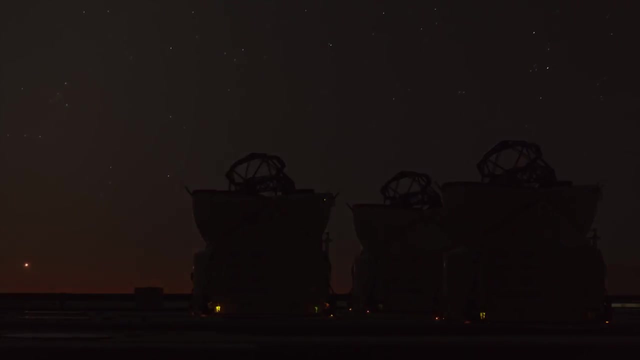 geology, evolution and composition. And there's one more thing: The universe is a violent place. Despite its serene beauty, the universe is a violent place. Things go bump in the night and astronomers want to catch each and every event. 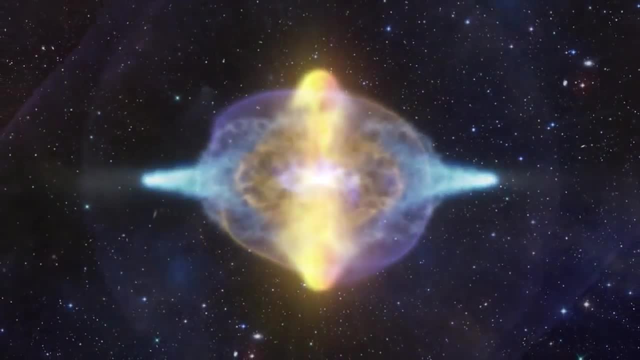 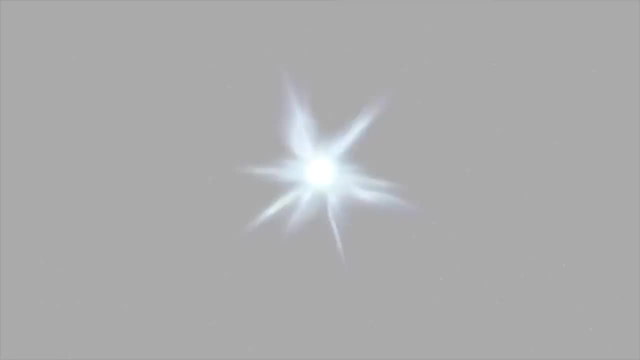 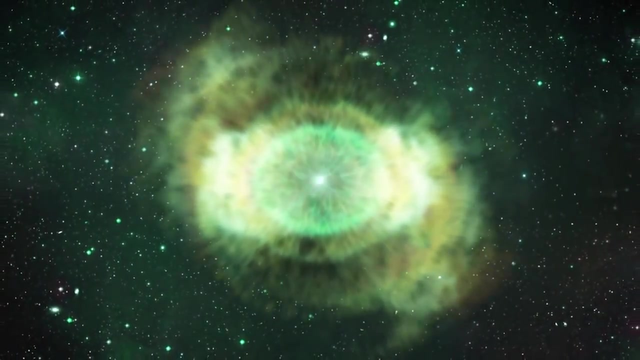 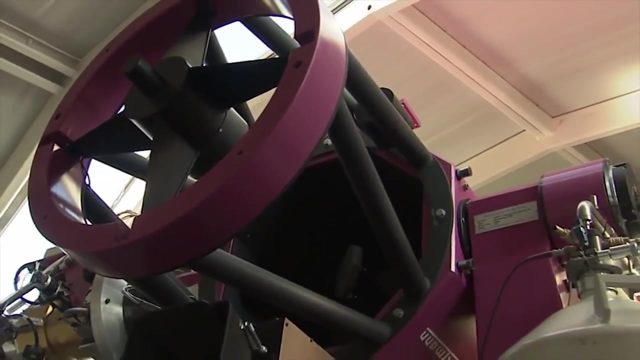 Massive stars end their lives in titanic supernova explosions. Some cosmic detonations are so powerful that they briefly outshine their parent galaxy, flooding intergalactic space with invisible high-energy gamma rays. Small robotic telescopes respond to automatic alerts from satellites. 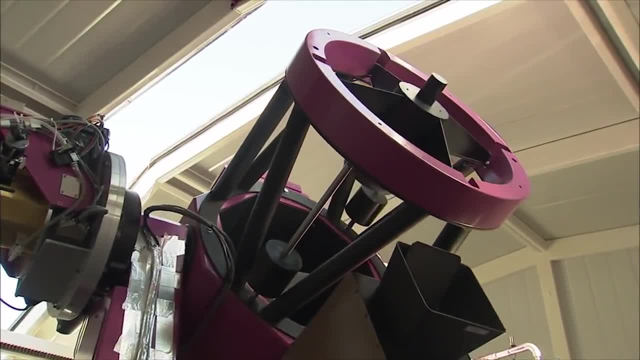 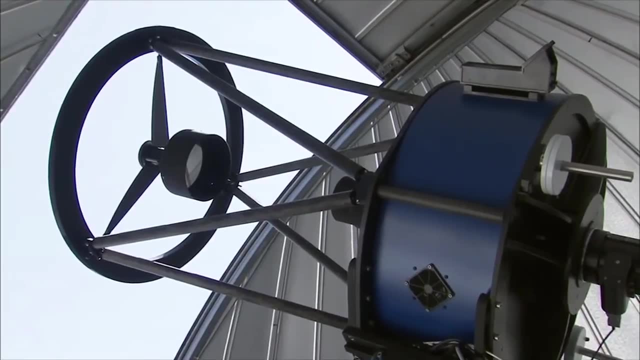 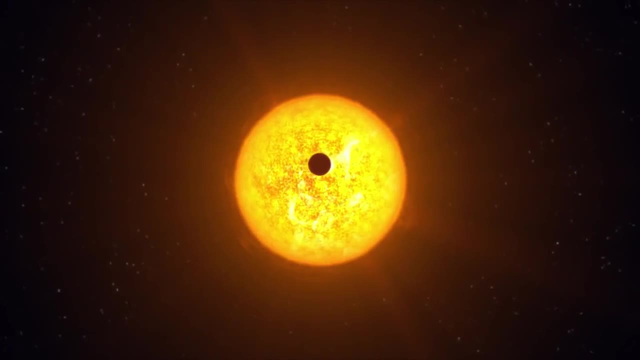 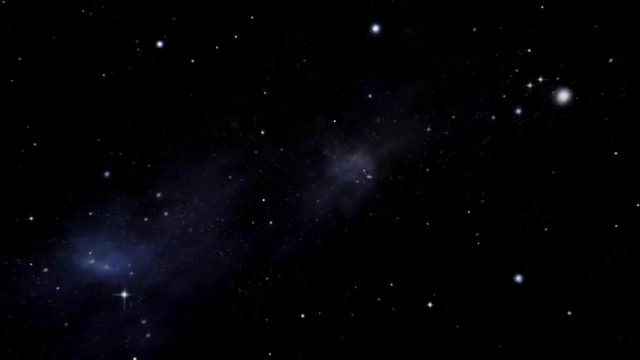 Within seconds, they swing into position to study the aftermaths of these explosions. Other roboscopes focus on less dramatic events, such as distant planets that pass in front of their mother stars. The cosmos is in a constant state of flux. ESO tries not to miss a single heartbeat. 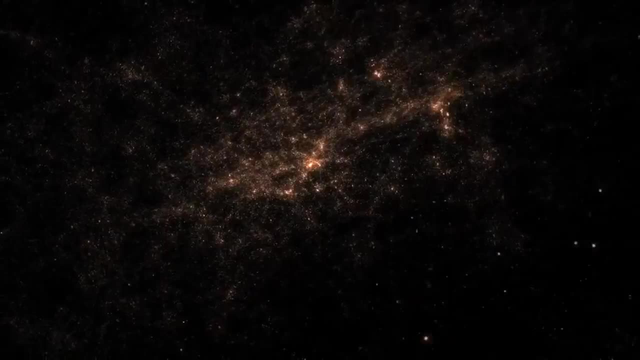 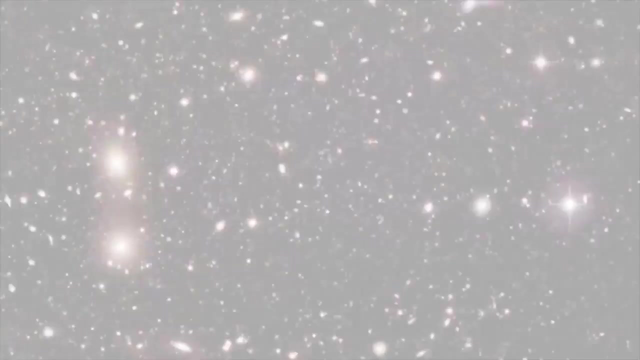 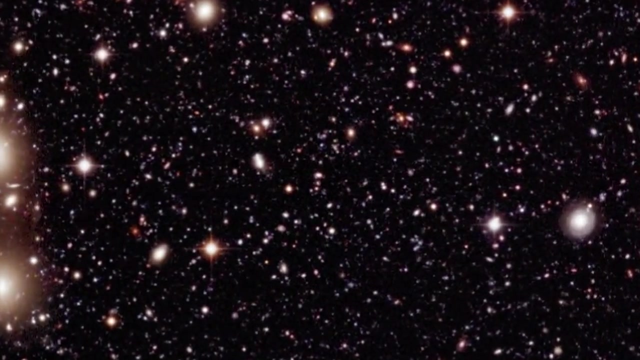 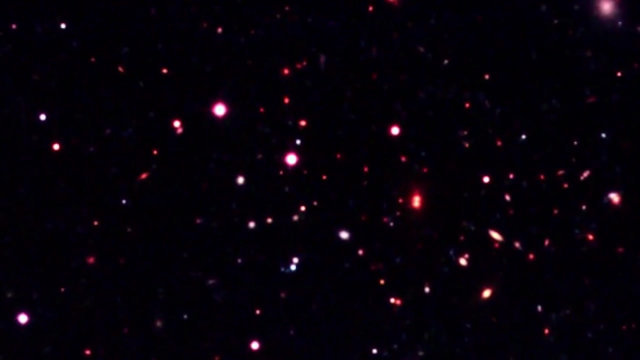 Cosmology is the study of the universe as a whole, its structure, evolution and origin. Here, catching as much light as possible is of the essence. These galaxies are so far away that only a handful of photons reach the Earth, But these photons hold clues to the cosmic past. 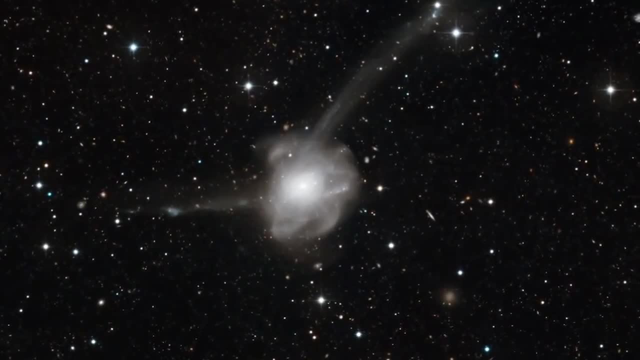 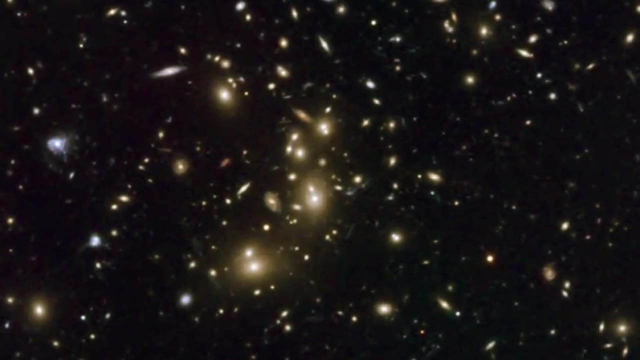 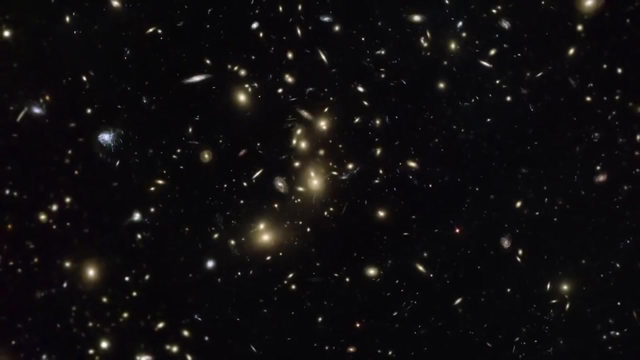 They have travelled for billions of years. They paint a picture of the early days of the universe. That's why the cosmic universe is so important to us. Big telescopes and sensitive detectors are so important. Over the past 50 years, ESO telescopes have revealed: 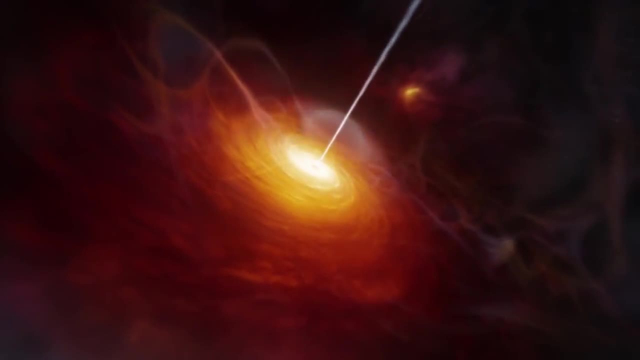 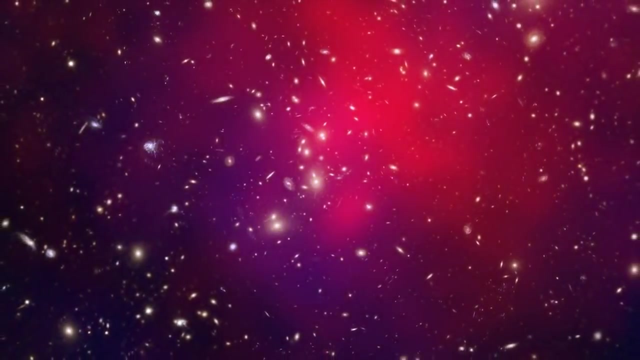 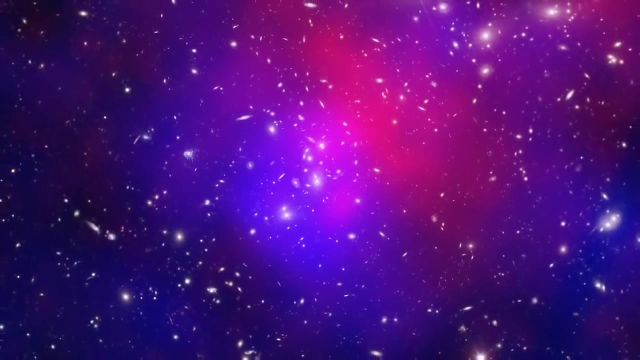 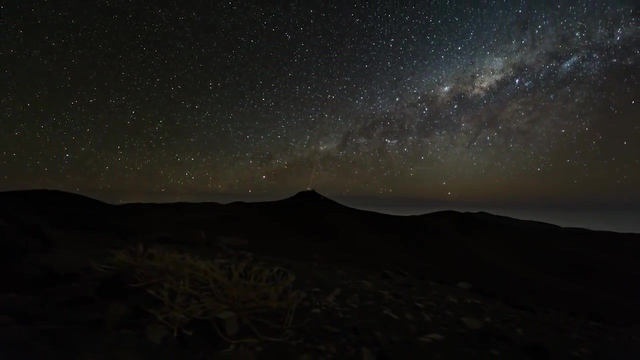 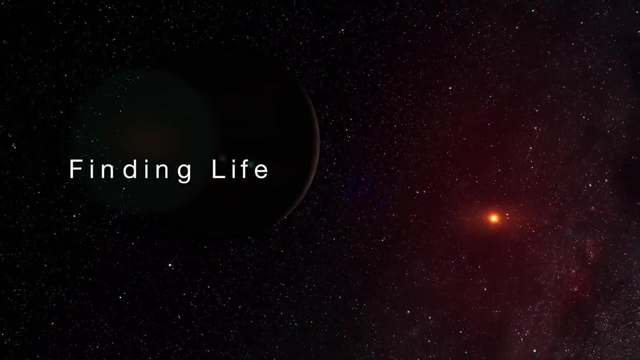 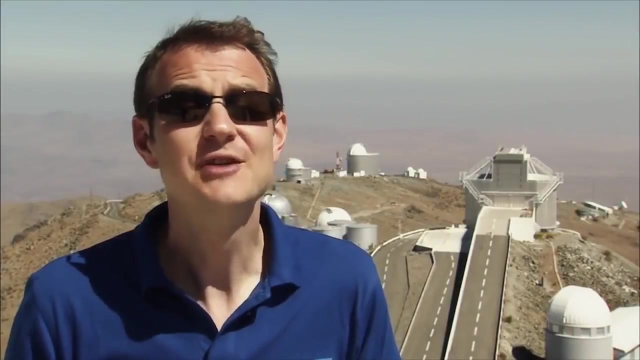 some of the most distant galaxies and quasars ever observed. They even helped to uncover the distribution of dark matter, the nature of which is still a mystery. Who knows what the next 50 years will bring? Have you ever wondered about life in the universe? 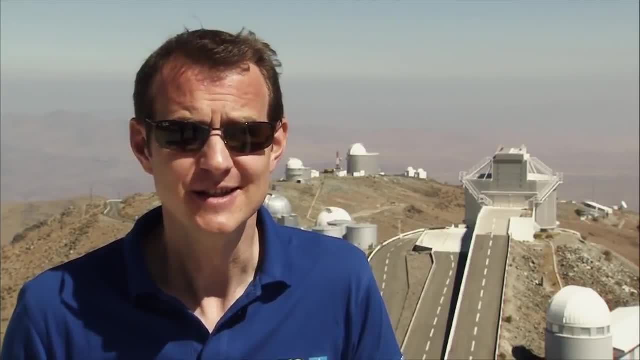 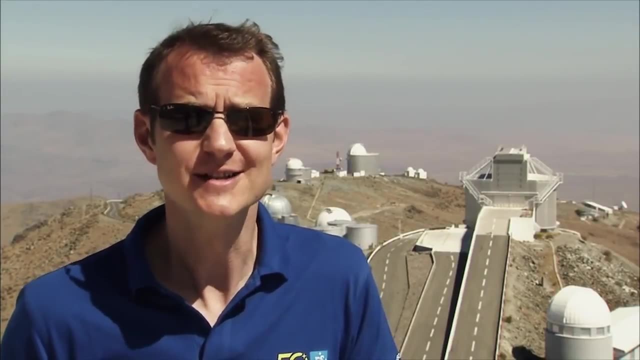 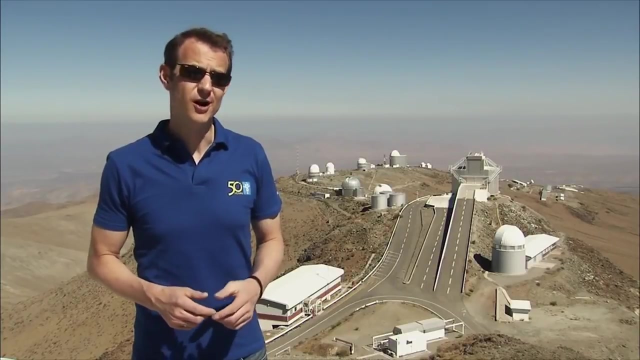 Inhabited planets orbiting distant stars? Well, astronomers have for centuries. After all, with so many galaxies and each with so many stars, how could the Earth be unique? In 1995, Swiss astronomers Michel Mayor and Didier Queloz, were the first to discover an exoplanet orbiting a normal star. Since then, planet hunters have found many hundreds of alien worlds, large and small, hot and cold and in a wide variety of orbits. Now we are on the brink. 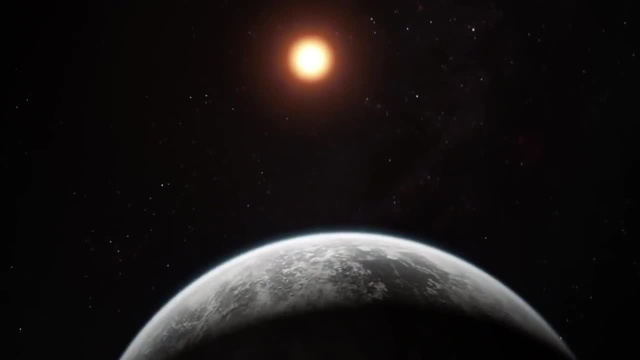 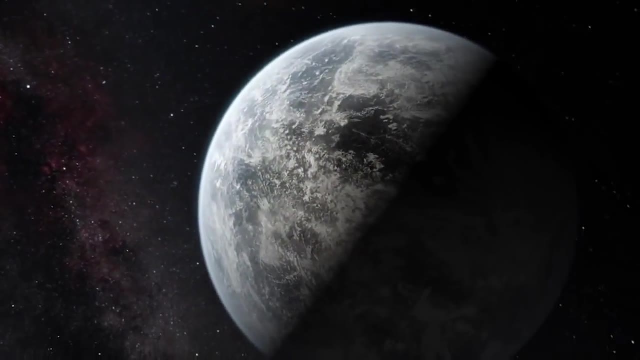 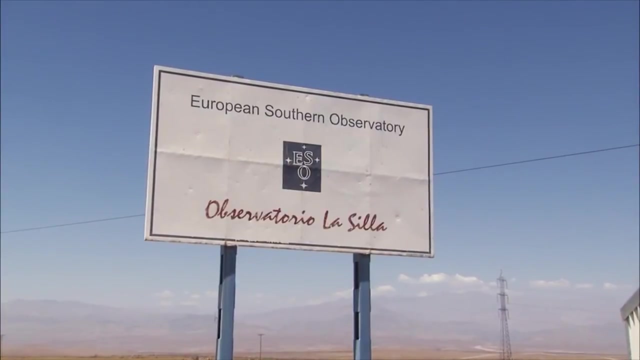 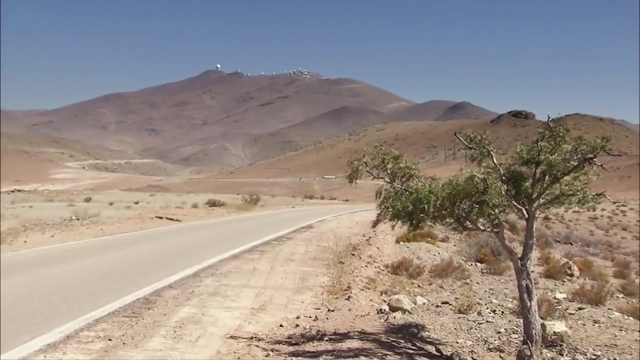 of discovering Earth's twin sisters And, in the future, a planet with life. The Holy Grail of astrobiologists, The European Southern Observatory plays an important role in the search for exoplanets. Michel Mayor's team found hundreds of them from Cerro La Silla. 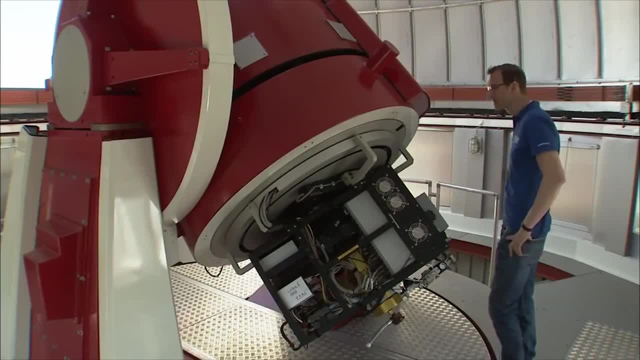 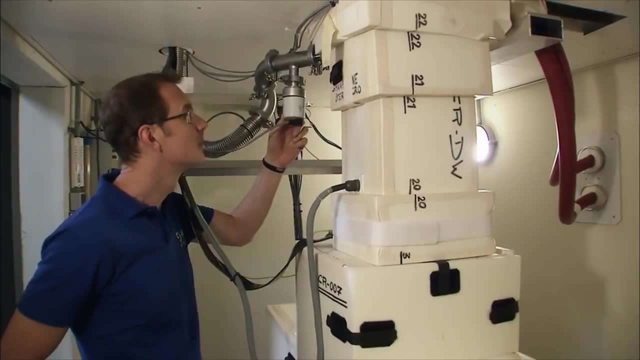 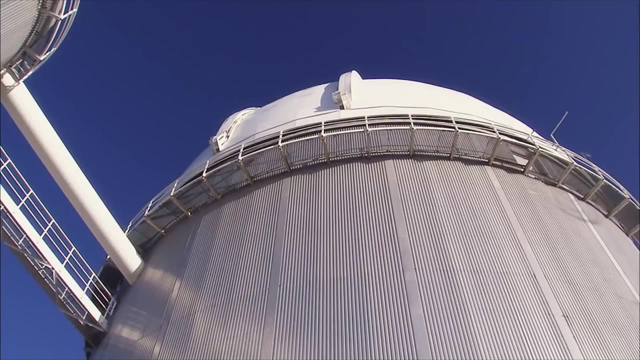 ESO's first Chilean foothold. Here's the Coralie spectrograph. mounted on the Swiss-Leonard Euler telescope, It measures the tiny wobbles of stars caused by the gravity of orbiting planets. ESO's venerable 3.6-meter telescope. 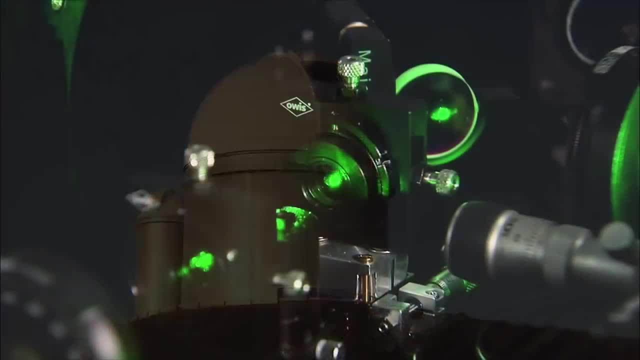 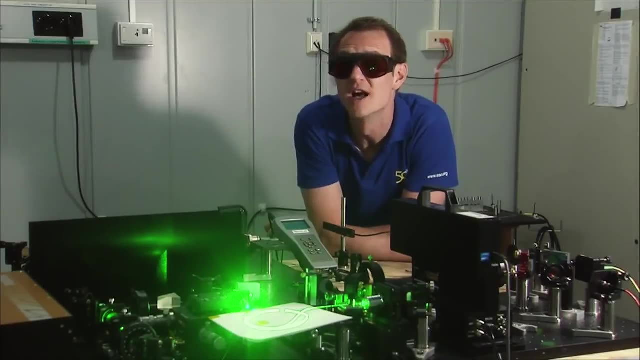 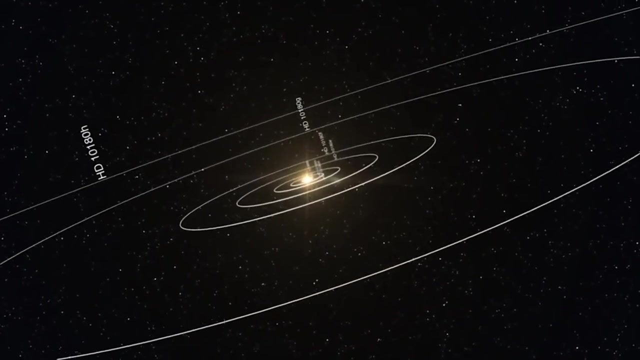 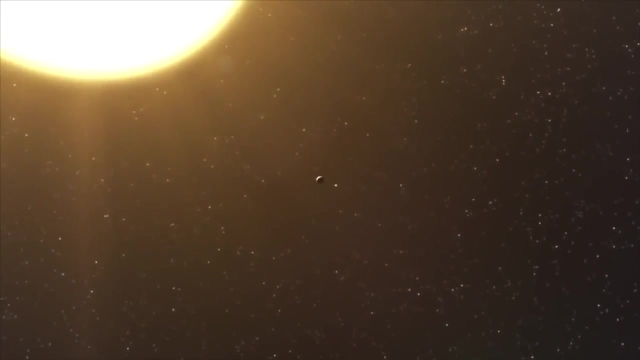 is also hunting for exoplanets. The HAARP spectrograph is the most accurate in the world. So far it's discovered more than 150 planets. It's biggest trophy, A rich system containing at least five and maybe as many as seven alien worlds. 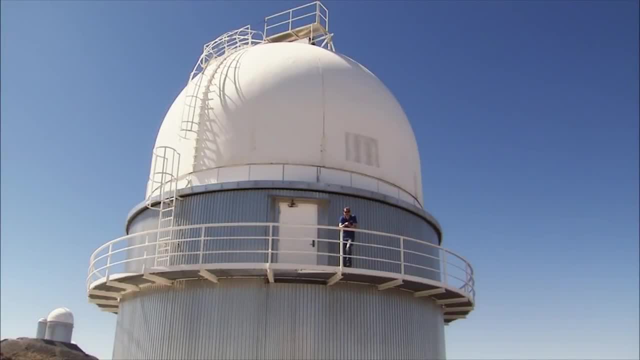 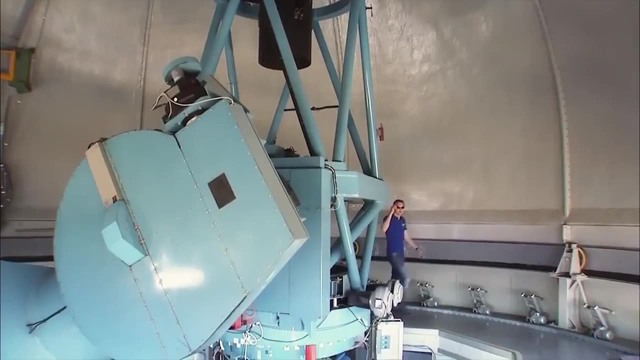 But there are other ways to find exoplanets. In 2006,, the 1.5-meter Danish telescope helped to discover a distant planet that is just five times more massive than the Earth. The trick: Gravitational microlensing. 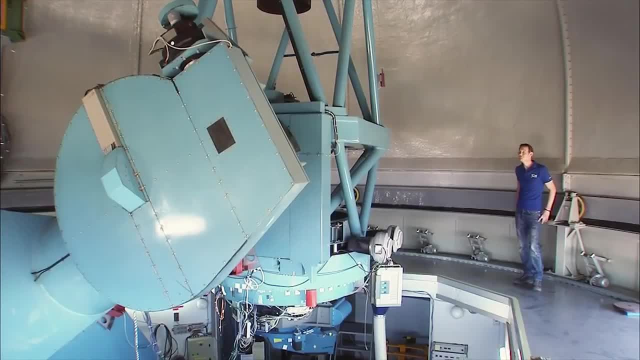 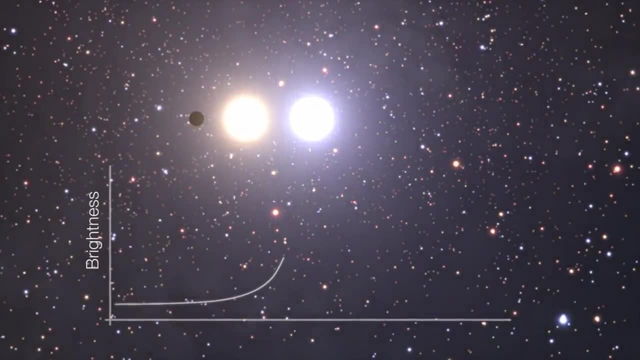 The planet and its parent star passed in front of a brighter star in the background, But the star itself was only five times larger than the Earth. The trick: Gravitational microlensing: The planet and its parent star passed in front of a brighter star. 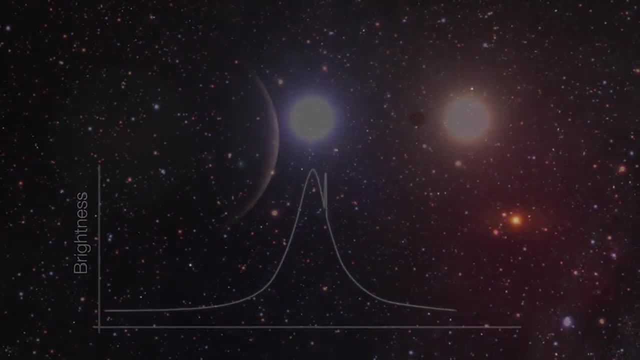 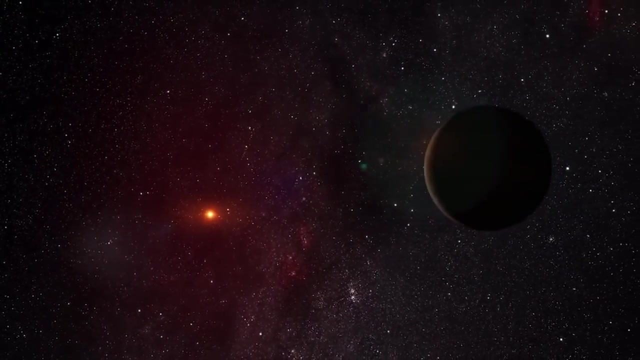 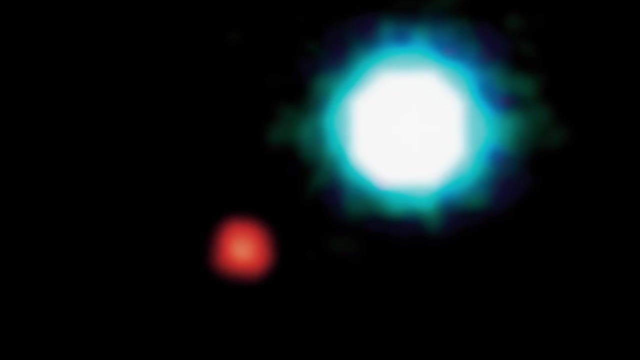 in the background, magnifying its image, And in some cases you can even capture exoplanets on camera. In 2004, NACO, the adaptive optics camera on the Very Large Telescope, took the first image ever of an exoplanet. 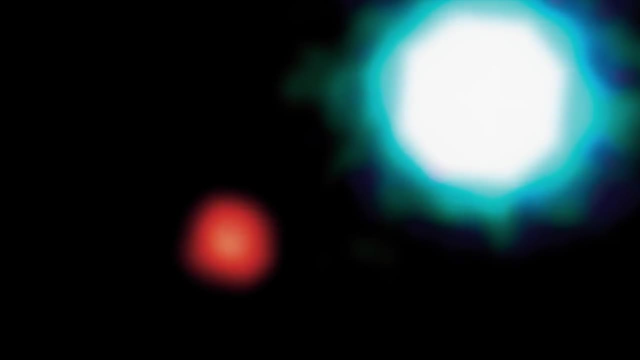 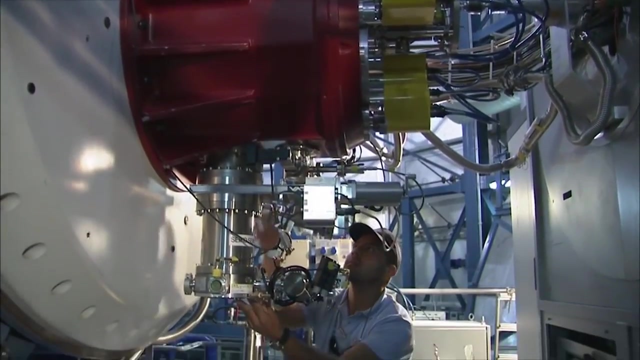 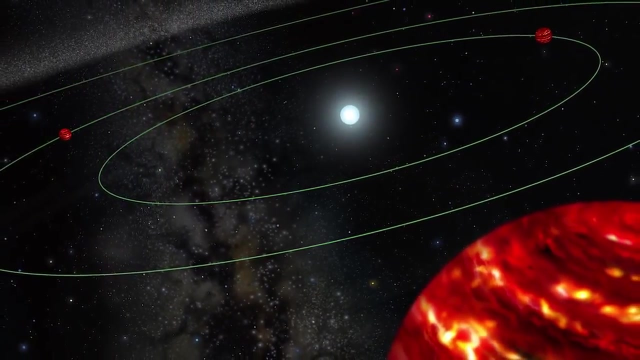 The red dot in this image is a giant planet orbiting a brown dwarf star. In 2010,, NACO went one step further. This star is 130 light-years away from Earth. It is younger and brighter than the Sun, and four planets circle around it. 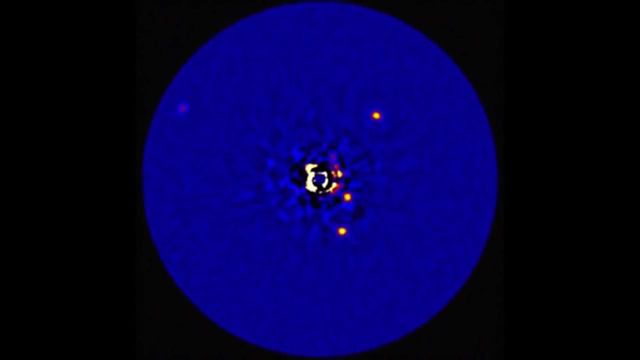 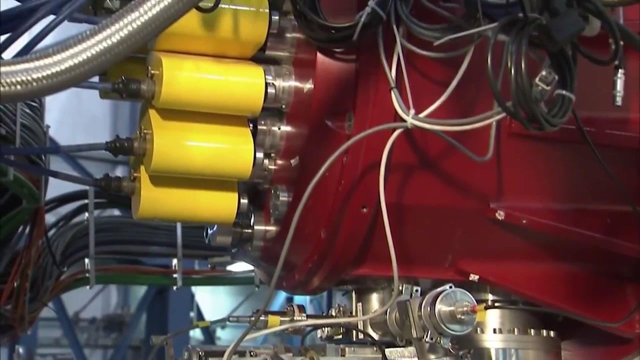 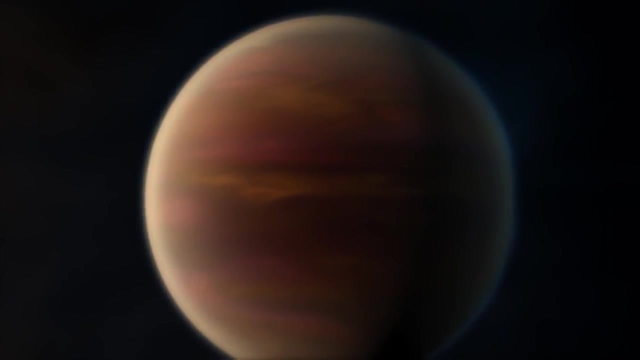 in wide orbits. NACO's eagle-eye vision made it possible to measure the light of Planet C, a gas giant ten times larger than the Earth. NACO's eagle-eye vision made it possible to measure the gas giant ten times larger than Jupiter. 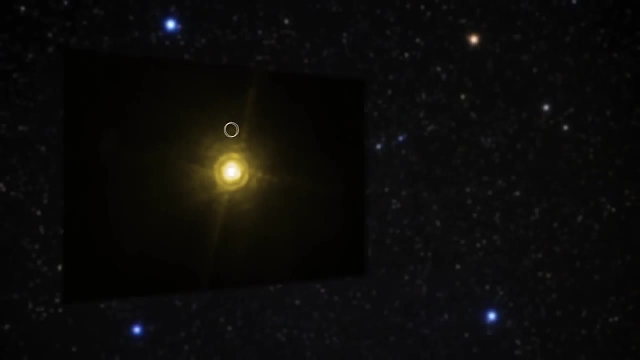 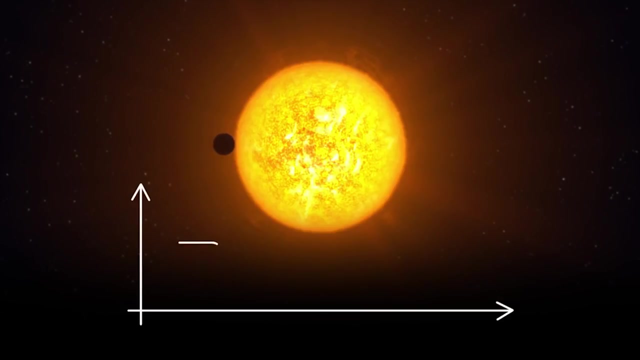 Despite the glare of the parent star, the feeble light of the planet could be stretched out into a spectrum revealing details about the atmosphere. Today, many exoplanets are discovered when they transit across their parent stars. If we happen to see the planet's orbit edge on, 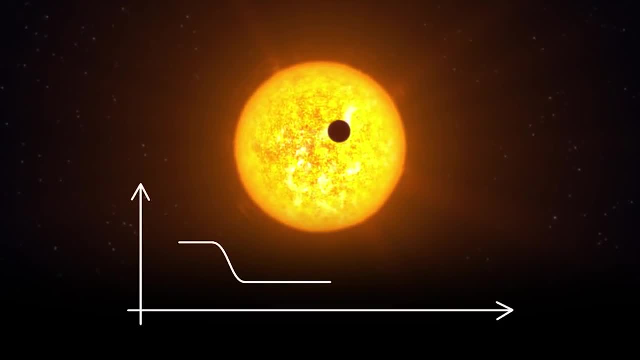 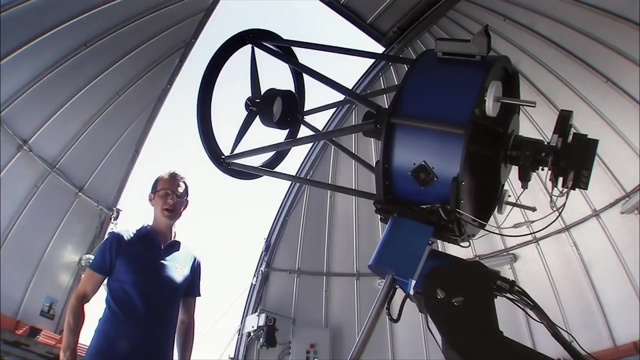 it will pass in front of its star every cycle. Thus tiny regular brightness dips in the light of a star betray the existence of an orbiting planet. The TRAPPIST telescope at La Silla will help search for these elusive transits. 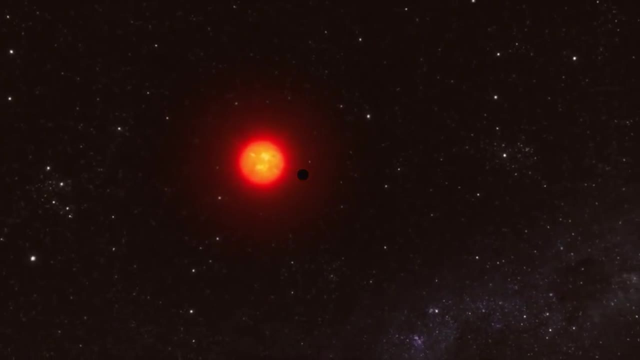 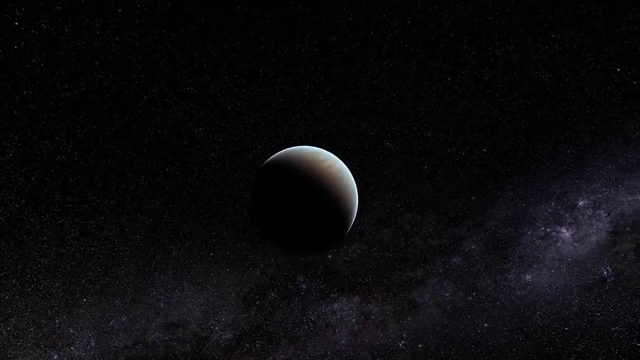 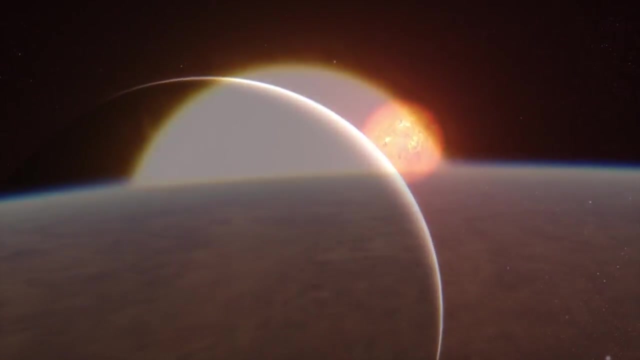 Meanwhile, the Very Large Telescope has studied a transiting planet in exquisite detail. Meet GJ 1214 b, a super-Earth 2.6 times larger than our home planet. During transits, the planet's atmosphere partly absorbs the light of the parent star. 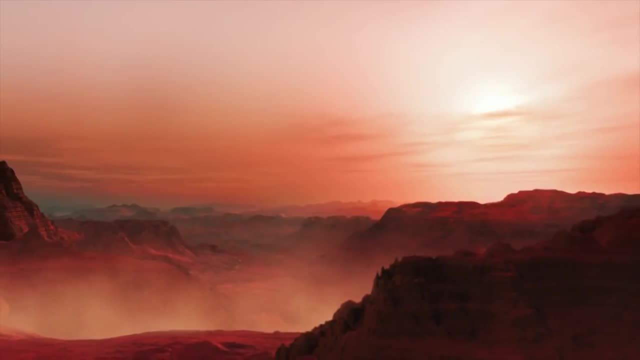 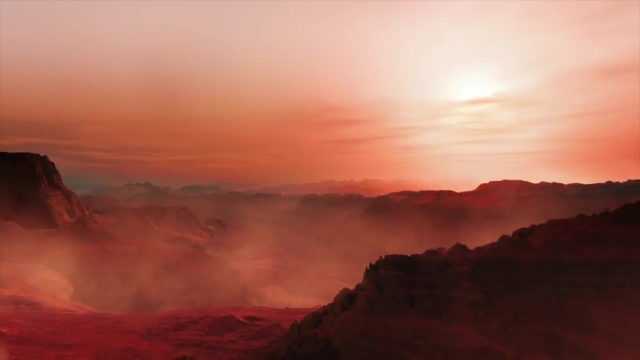 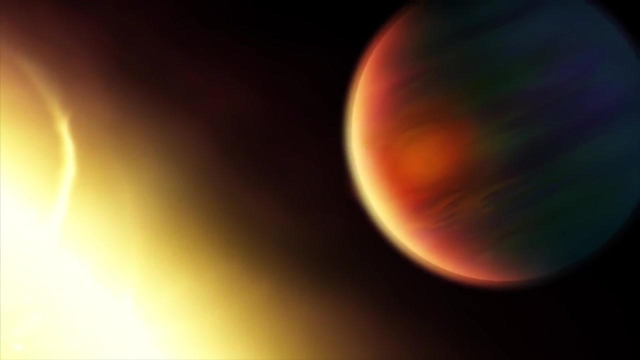 ESO's Sensitive Force Spectrograph revealed that GJ 1214 b might well be a hot and steamy sauna world. Gas giants and sauna worlds are inhospitable to life, but the hunt is not over yet. Soon, the new SPHERE instrument. 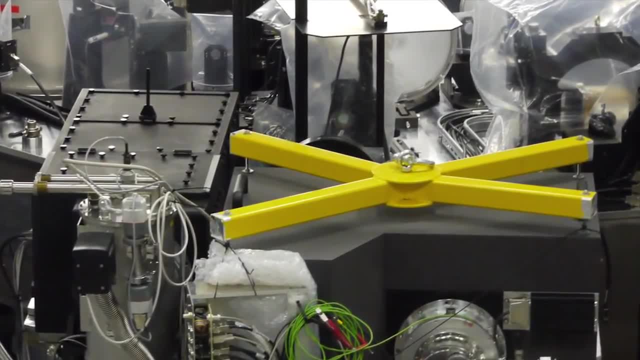 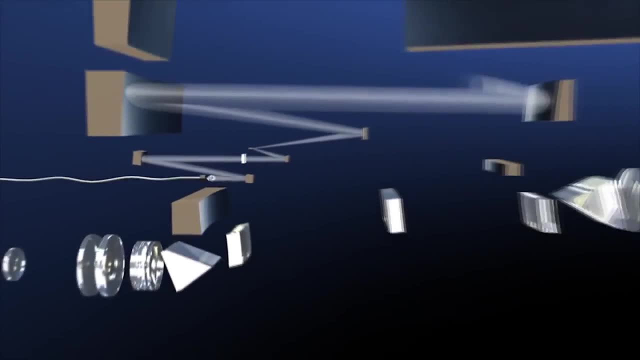 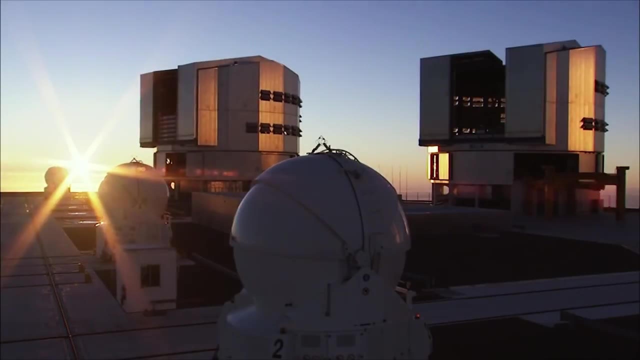 will be installed at the VLT, SPHERE will be able to spot faint planets in the glare of their host stars. In 2016,, the ESPRESSO spectrograph will arrive at the VLT and greatly surpass the current HARPS instrument. 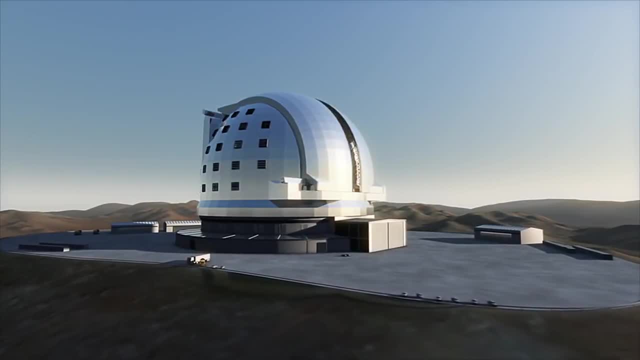 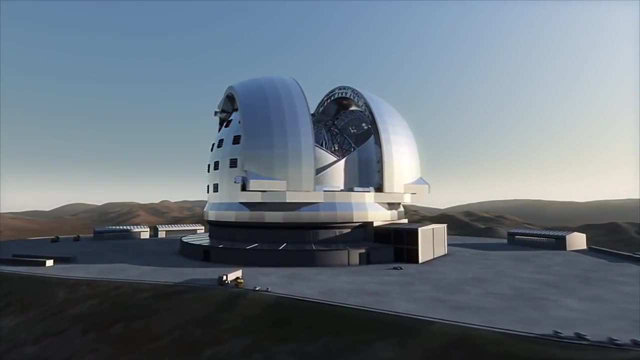 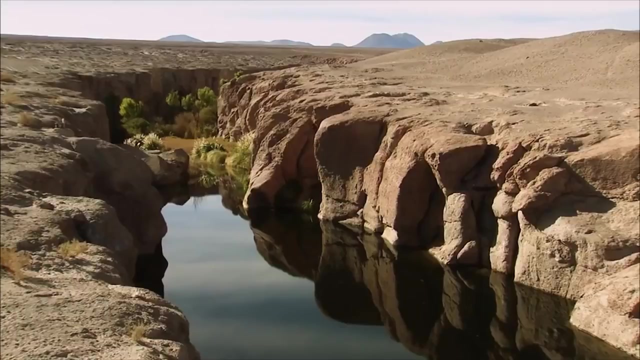 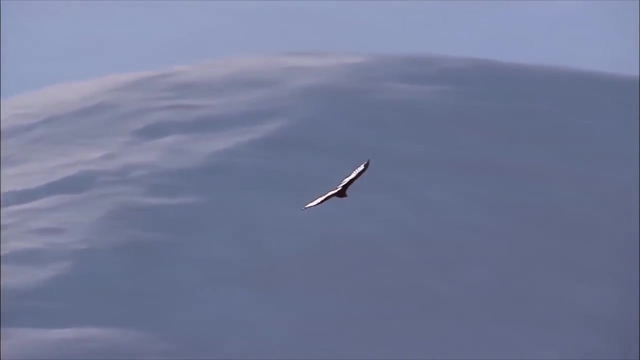 And ESO's Extremely Large Telescope, once completed, may well find evidence for alien biospheres On Earth. life is abundant. Northern Chile offers its share of condors, vicuñas, vizcachas and giant cats. Even the arid soil 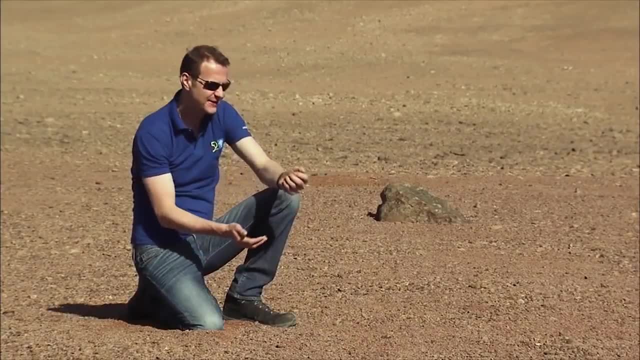 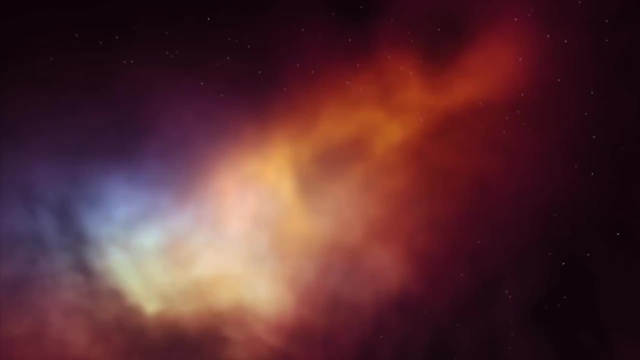 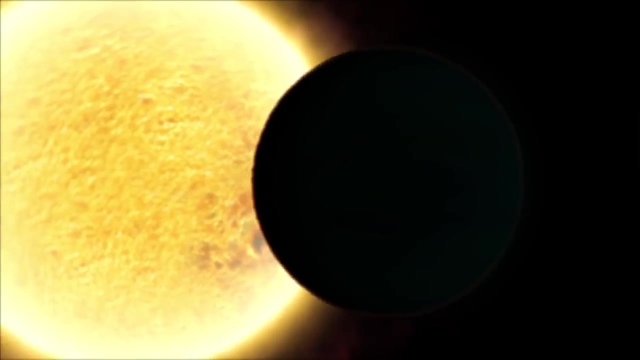 of the Atacama Desert teems with hardy microbes. We've found the building blocks of life in interstellar space. We've learned that planets are abundant. Billions of years ago, comets brought water and organic molecules to Earth. But how did they get to Earth? 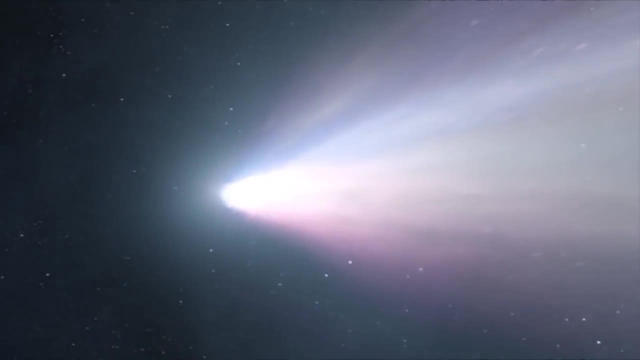 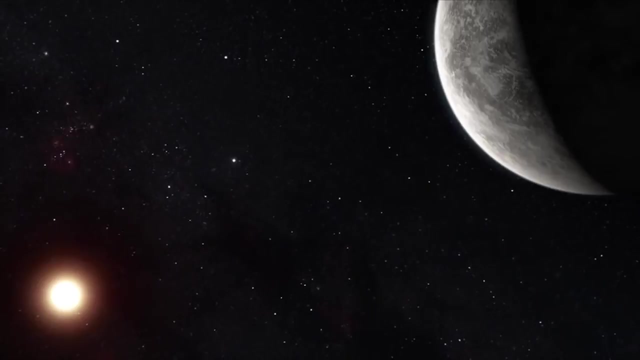 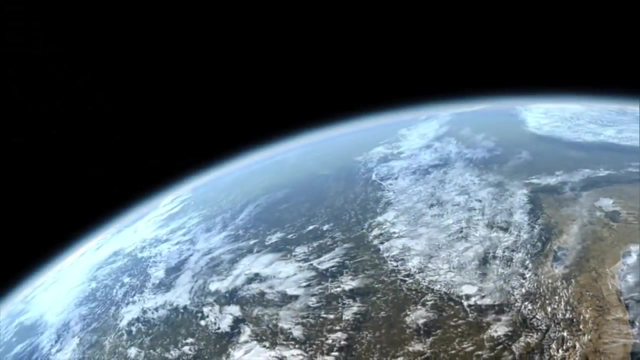 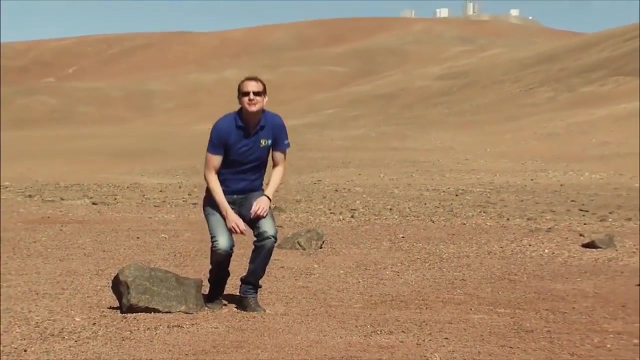 We're going to find out. Billions of years ago, comets brought water and organic molecules to Earth. Wouldn't we expect the same thing to happen elsewhere, Or are we alone? It's the biggest question ever And the answer is almost within reach. 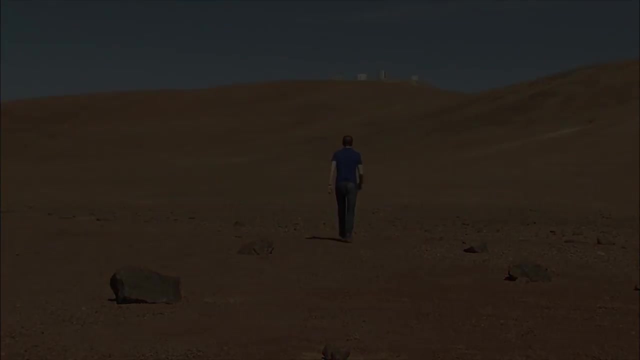 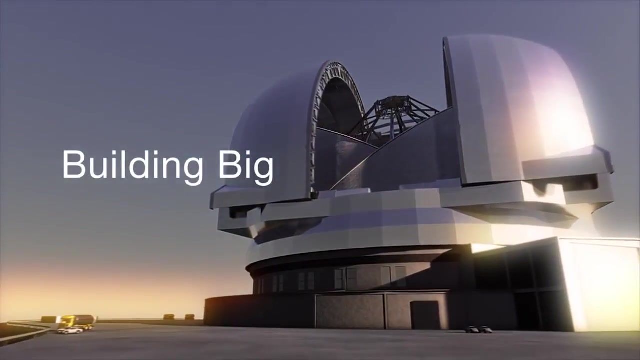 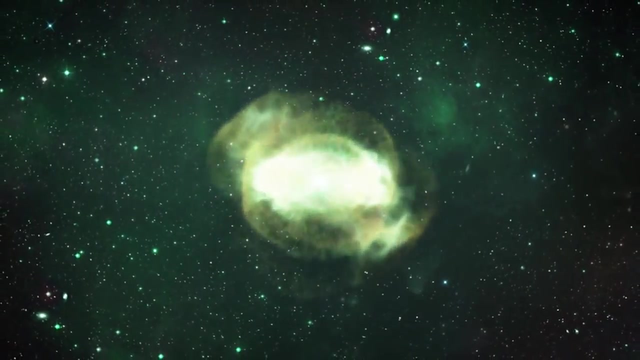 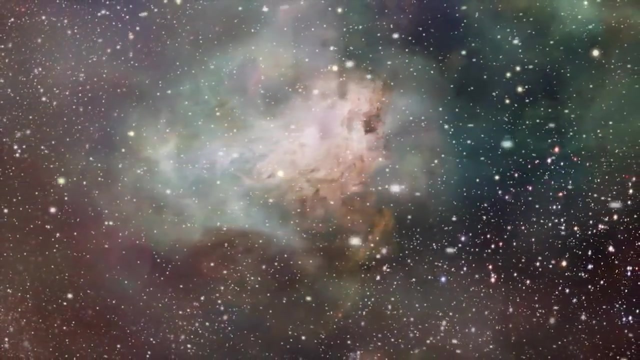 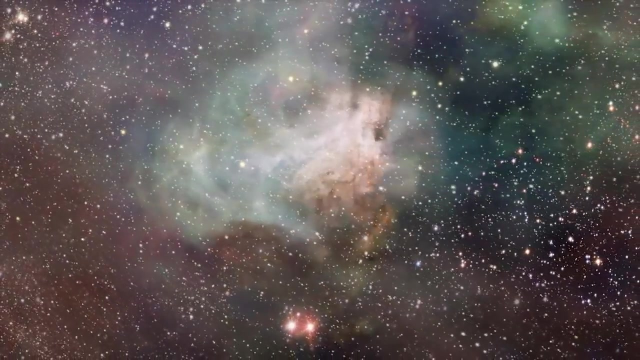 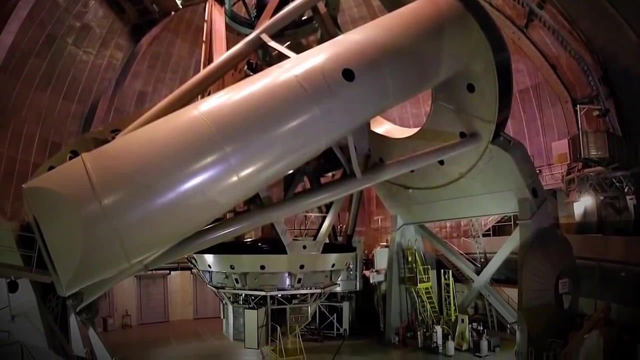 NASA's Lieu. Astronomy is big science. It's a vast Universe out there And the exploration of the cosmos requires huge instruments. This is the 5-metre hail reflector on Paloma Mountain. When the European Southern Observatory came into being 50 years ago, it was the largest. 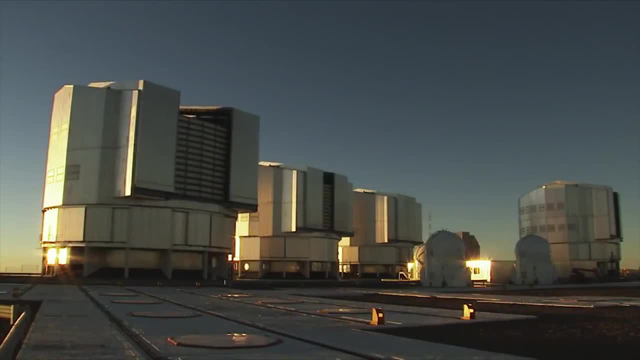 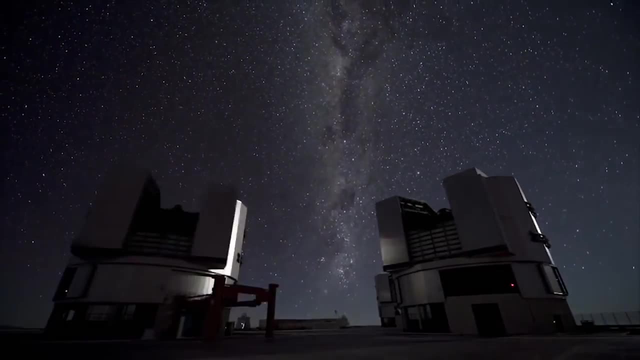 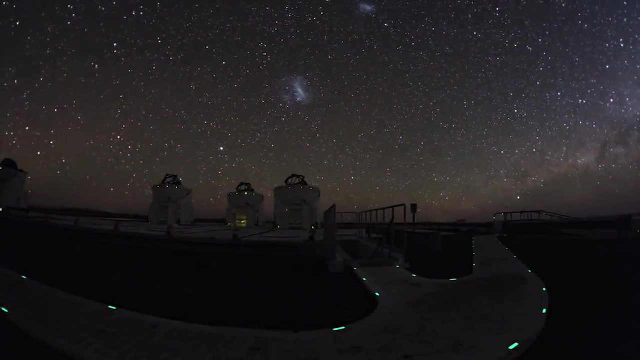 telescope in the world. ESO's Very Large Telescope at Cerro Paranal is the state of the art now. As the most powerful observatory in history, it has revealed the full splendour of the universe in which we live, But astronomers have set their sights on even bigger instruments. 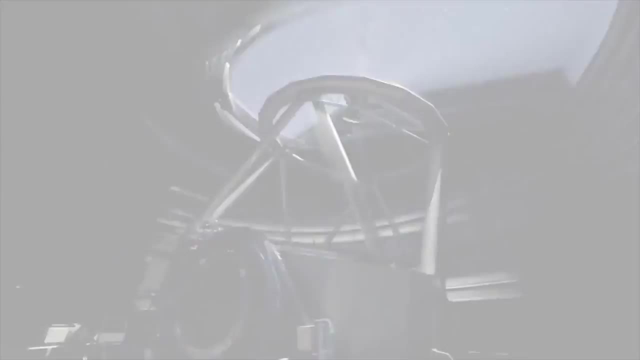 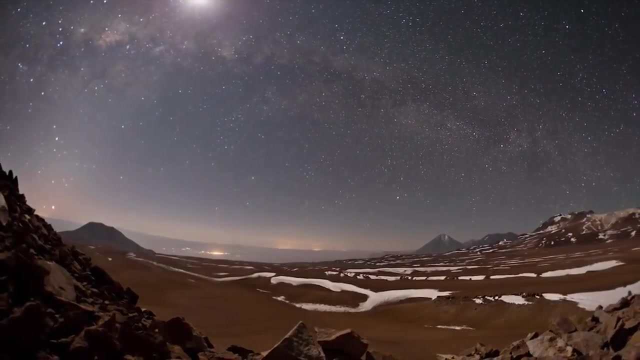 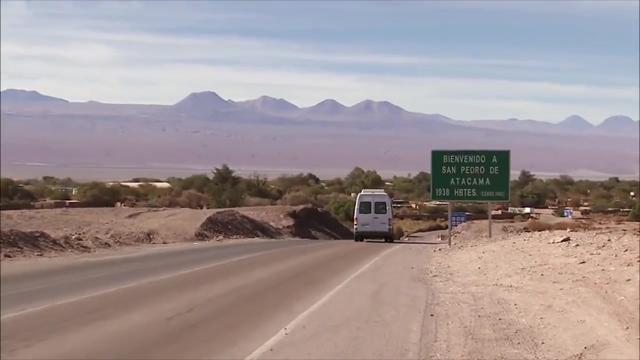 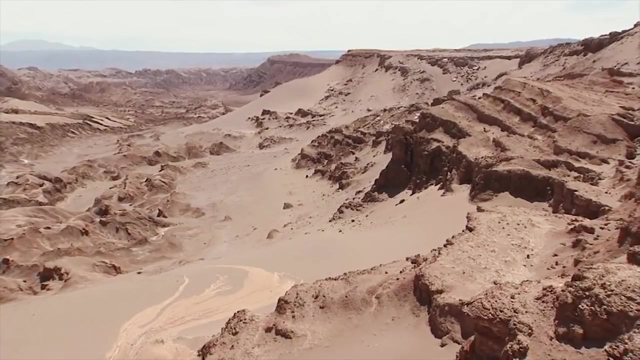 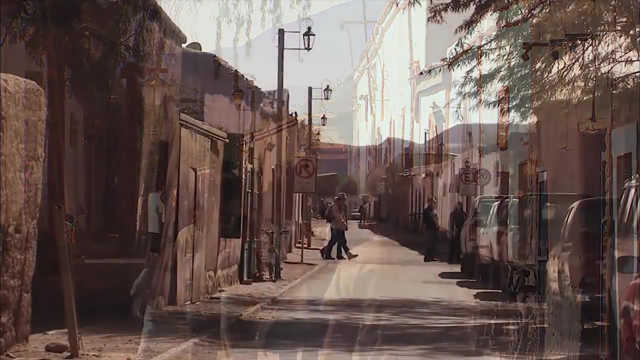 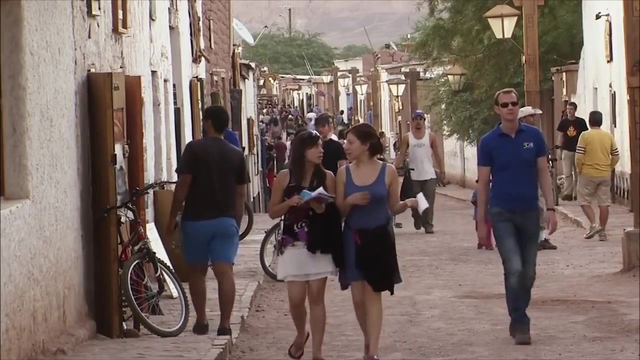 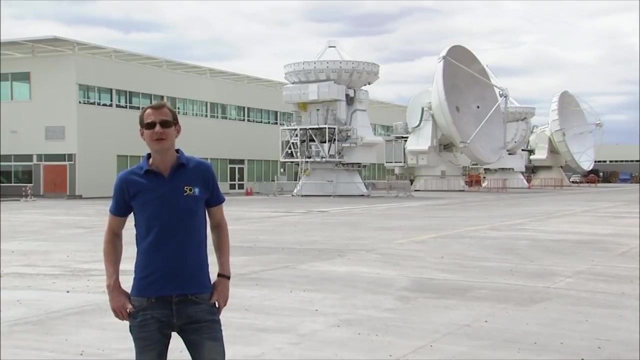 And ESO is realising their dreams. San Pedro de Atacama: Tucked amidst breathtaking scenery and natural wonders, this picturesque town is home to indigenous Atacameños and adventurous backpackers alike, and ESO astronomers and technicians. Not far from San Pedro, ESO's first dream machine is taking shape. 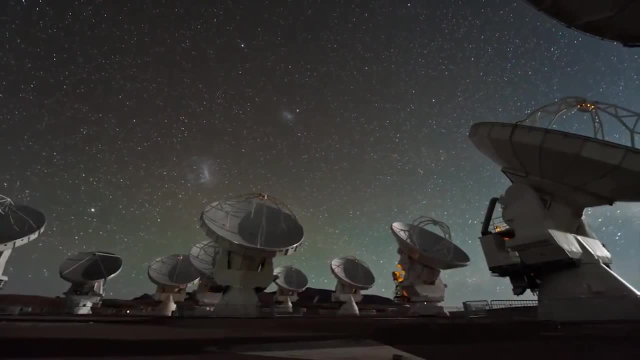 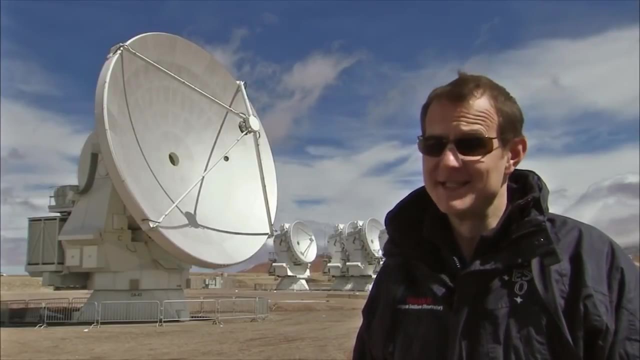 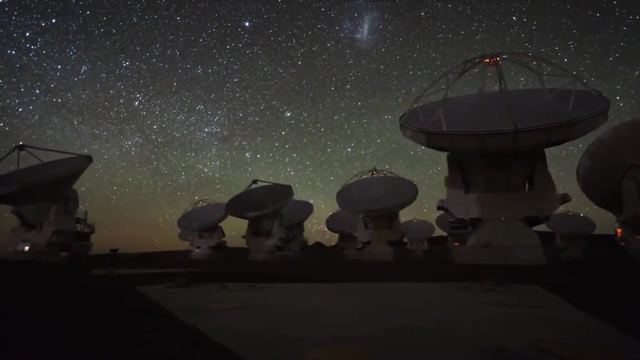 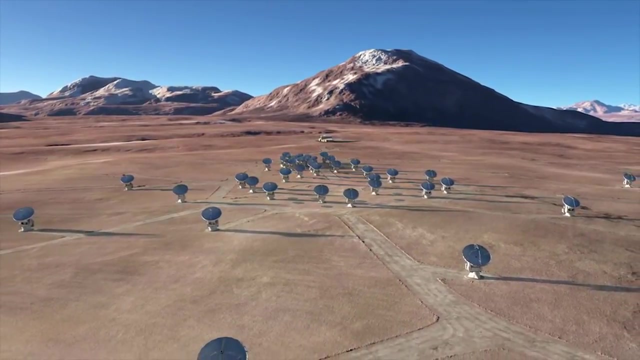 It's called ALMA, The Atacama Large Telescope. ALMA is a joint project of Europe, North America and East Asia. It operates like a giant zoom lens. Closed together, the 66 antennas provide a wide-angle view, But spread apart, they reveal much finer detail over a smaller area of sky. 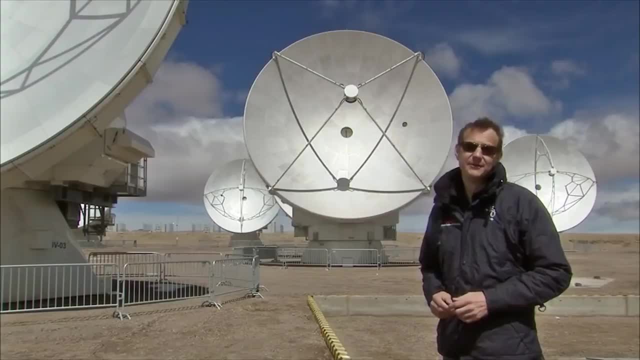 At sub-millimetre wavelengths, ALMA sees the universe in a different light. It's the first time we've seen ALMA in a wide-angle view. It's the first time we've seen ALMA in a wide-angle view. It's the first time we've seen ALMA in a wide-angle view. 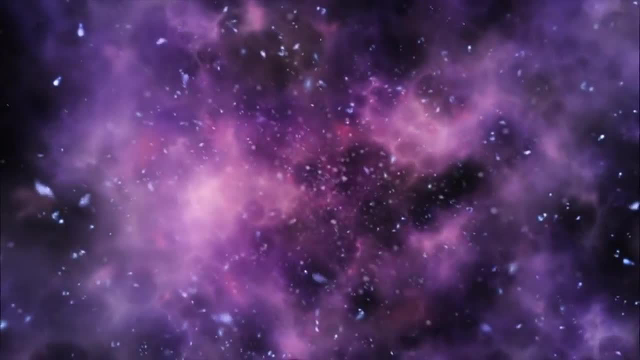 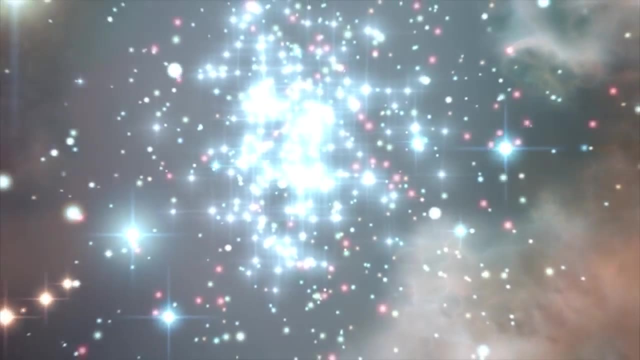 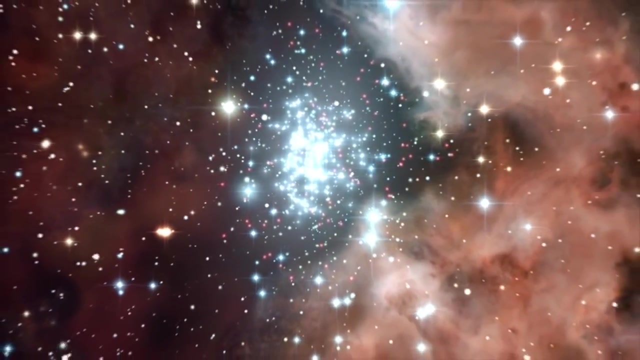 But what will it reveal? The birth of the very first galaxies in the universe in the wake of the Big Bang, Cold and dusty clouds of molecular gas, The stellar nurseries where new suns and planets are born, And the chemistry of the cosmos. 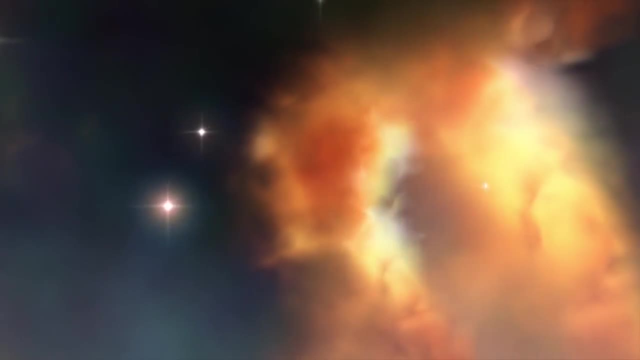 ALMA will track down organic molecules. It's the first time we've seen ALMA in a wide-angle view. It's the first time we've seen ALMA in a wide-angle view. It's the first time we've seen ALMA in a wide-angle view. 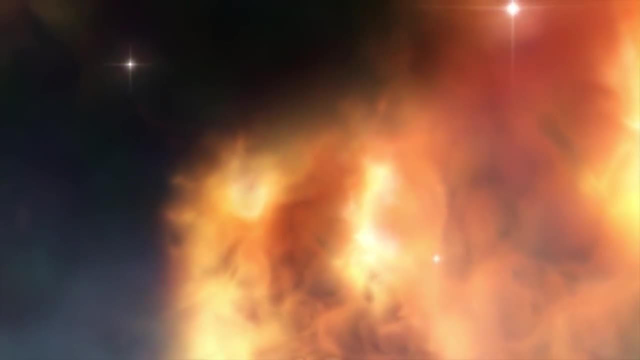 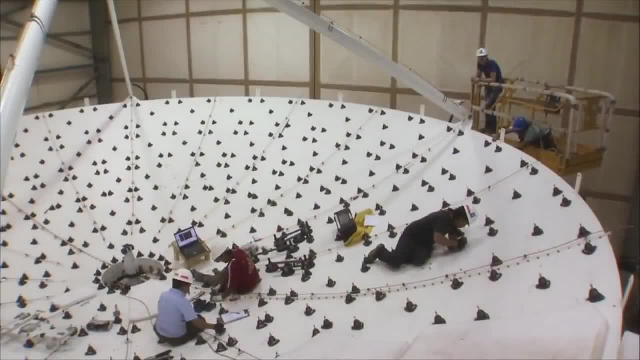 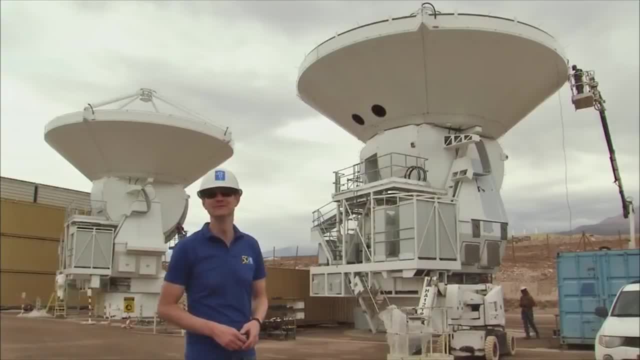 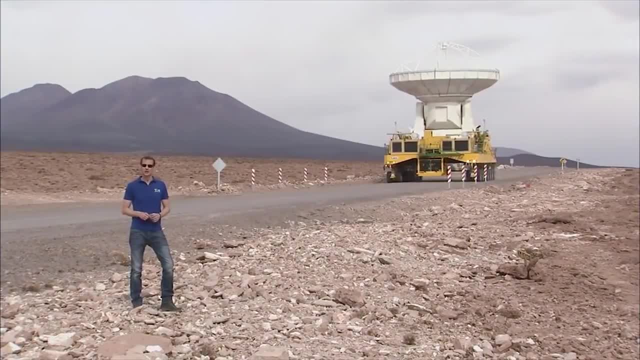 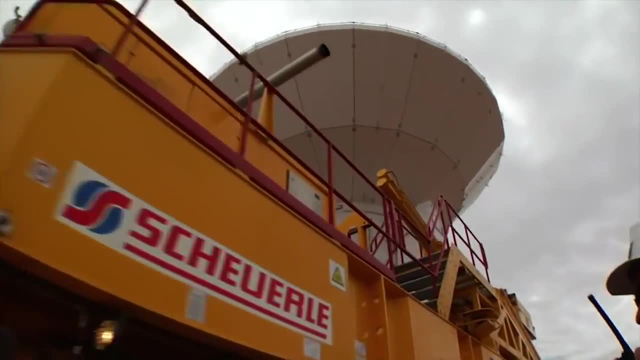 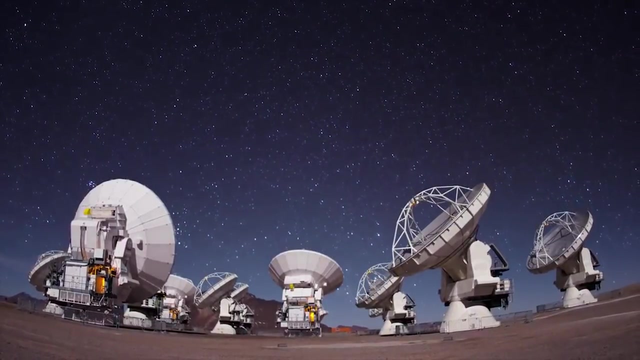 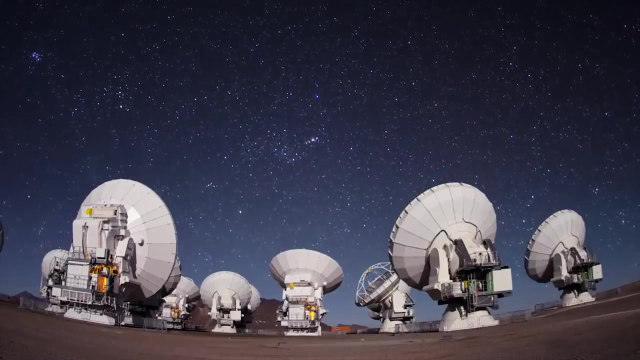 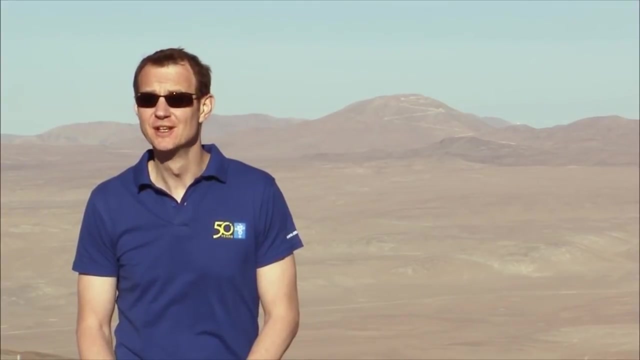 Two giant transporters called Otto and Loreth take the completed antennas up to the Chajnantur plateau At 5,000 meters above sea level. the array provides an unprecedented view of the microwave universe. While ALMA is nearly completed, ESO's next dream machine is still a few years away. 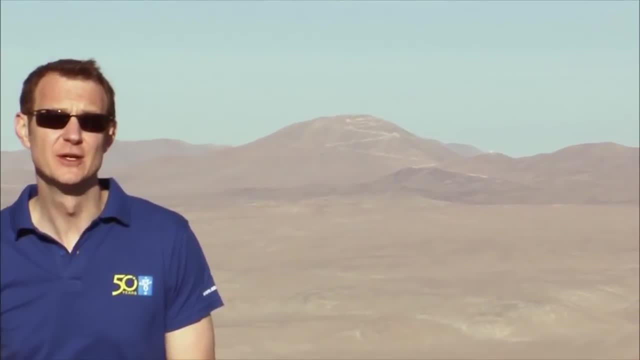 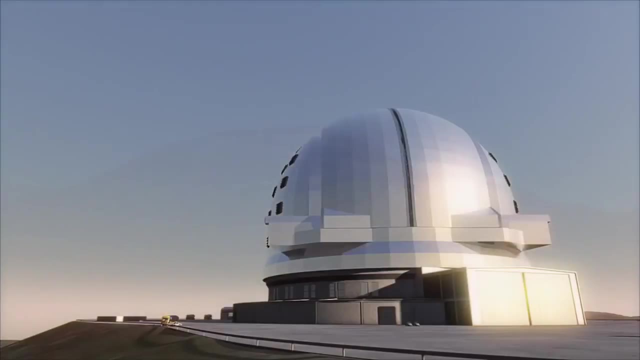 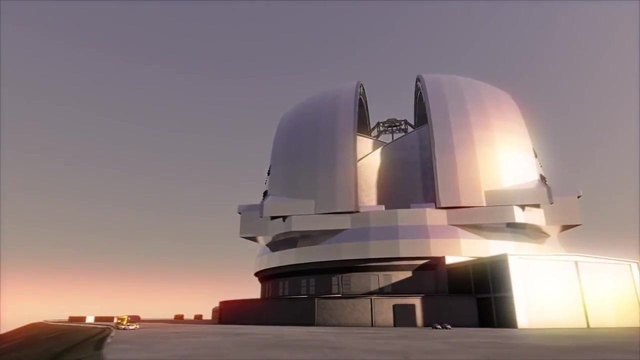 See that mountain over there. That's Cerro Amazonas, Not far from Paranal. it will be home to the largest telescope in the history of mankind. Meet the European Space Telescope. Extremely large telescope, The world's biggest eye on the sky.